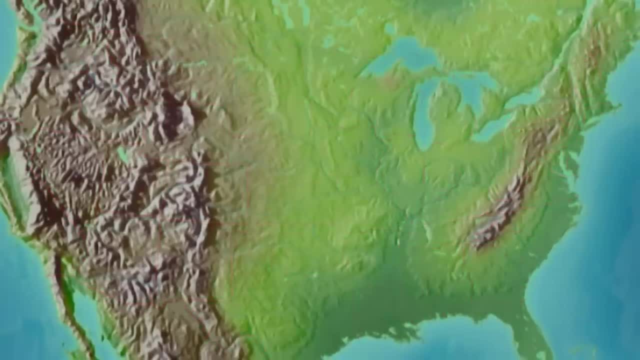 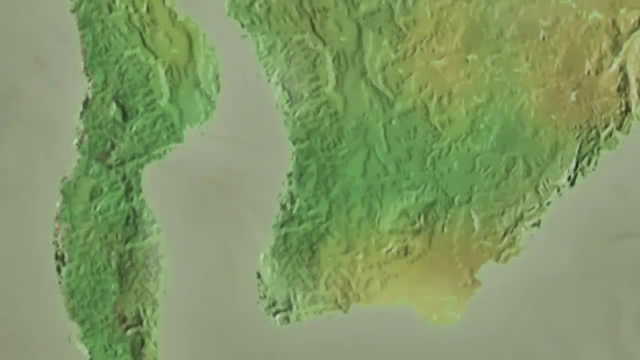 But 65 million years ago and beyond, it was full of dinosaurs. In those days, known as the Cretaceous, America looked a bit different. The continent was split down the middle by a huge ocean and the Rockies were only just beginning to form. 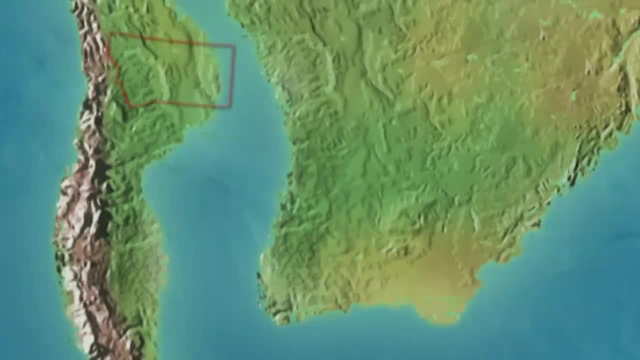 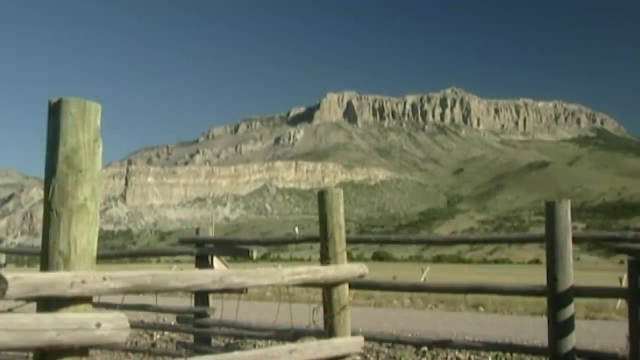 What's now Montana was a fertile plain sandwiched between mountains and sea. The landscapes changed, but in those days it was home to all kinds of fabulous beasts – hadrosaurs, triceratops, torosaurs, troodonts and many, many more. But in those days it was home to all kinds of fabulous beasts – hadrosaurs, triceratops, torosaurs, troodonts and many, many more. But in those days it was home to all kinds of fabulous beasts – hadrosaurs, troodonts. 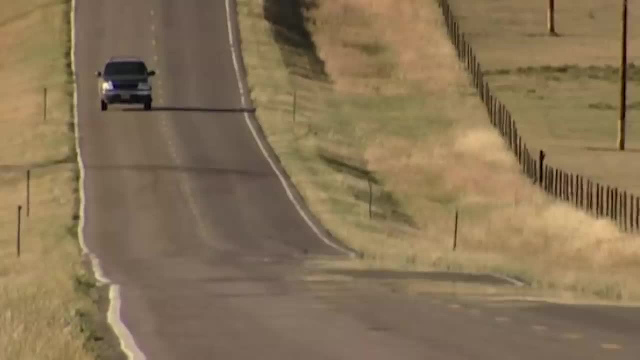 and many, many more. But in those days it was home to all kinds of fabulous beasts – hadrosaurs, troodonts, torosaurs, troodonts and many, many more. But in those days it was home to all kinds of fabulous beasts – hadrosaurs, troodonts. 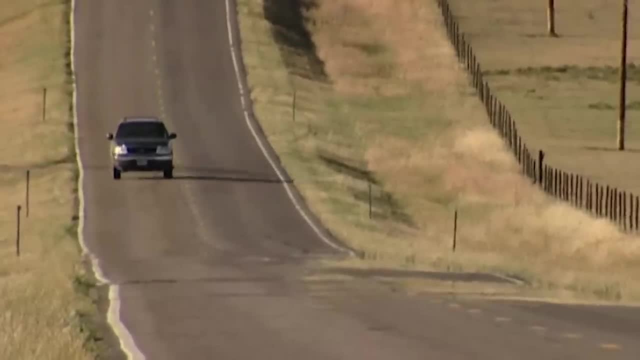 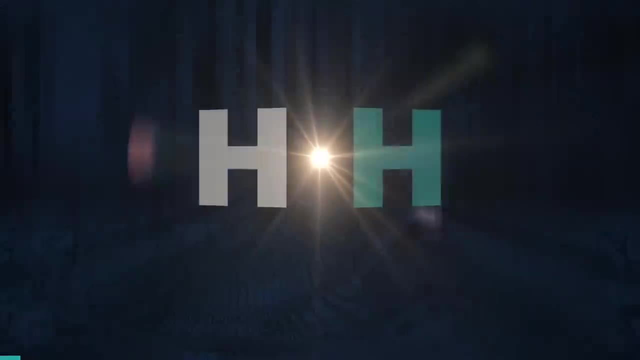 troodonts and many, many more. They're all just names at the moment, but over the next three weeks and 1500 miles, we hope to meet and even bag a few for ourselves. If you love history, then you'll love History Hit. 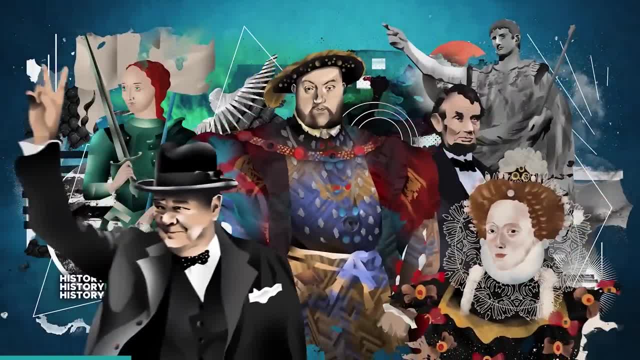 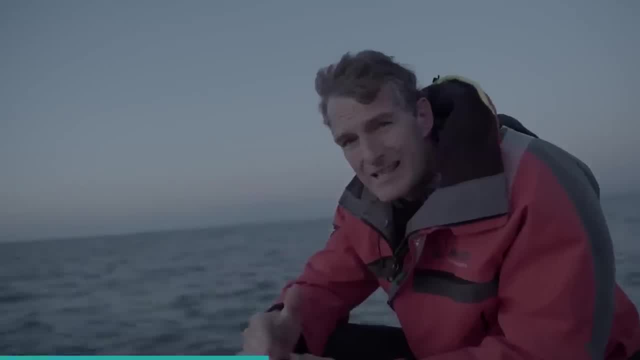 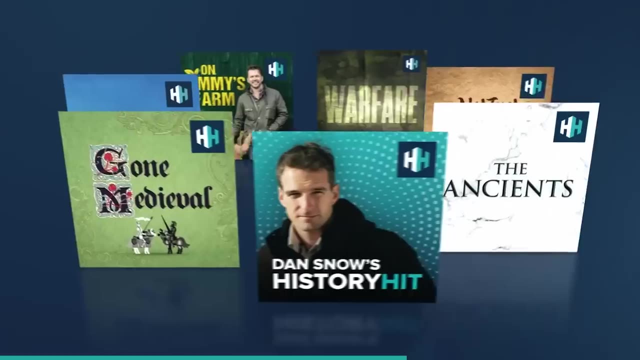 Our extensive library of documentary features everything from the ancient origins of our earliest ancestors to the daring mission to sink the bismarck. History Hit has hundreds of exclusive documentaries with unrivalled access. We're committed to bringing history fans award-winning documentaries and podcasts. 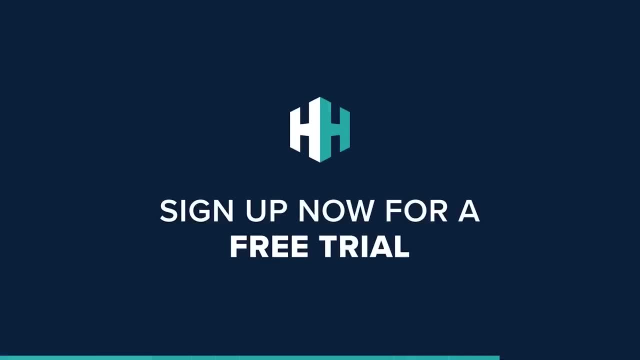 that you cannot find anywhere else. Sign up now for a free trial and Timeline fans get 50% off their first three months. Just be sure to use the code TIMELINE at checkout. I've got this image in my mind that there'll be the Rockies and on the side of them there'll. 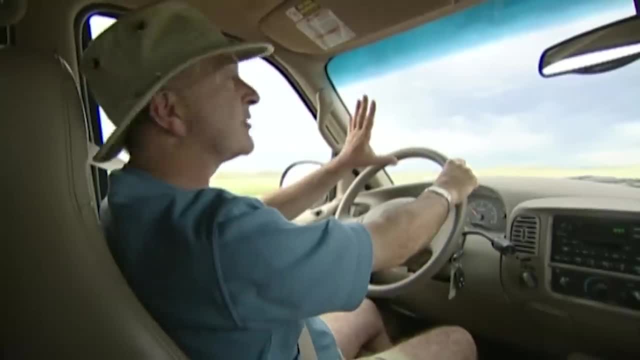 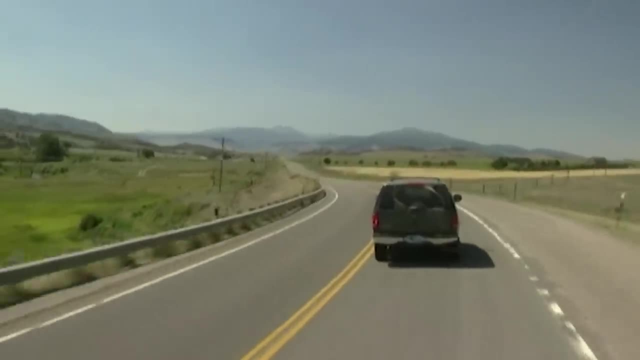 be this massive fossil of a Tyrannosaurus rex kind of just lying there, A fantasy idea. Tony, I reckon we should be lucky if we get articulated bones. to be quite honest, I mean, just think that thing has died and then there's going to be vast earth movements. 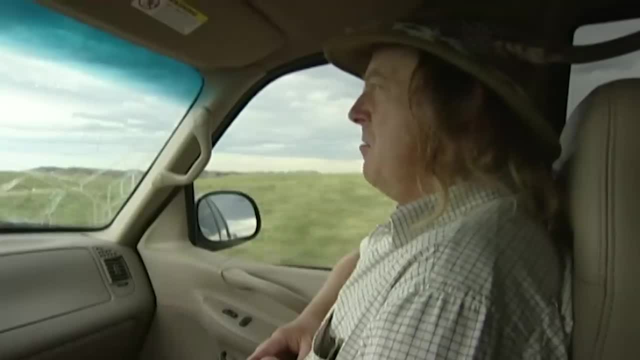 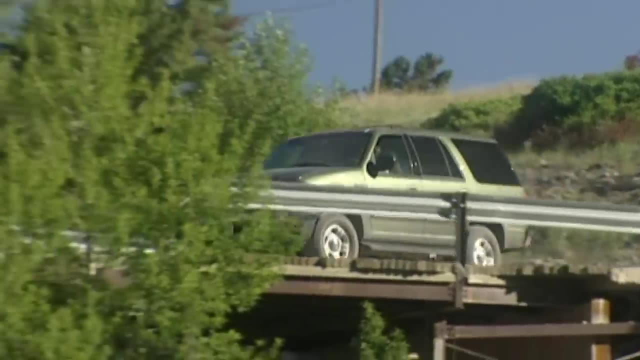 No, I reckon they'll be a bit more dispersed than that. I mean, have you ever actually handled a fossil? Does Mick Astin count? Our first site is a research dig in the west of the state, sponsored by the Museum of the. 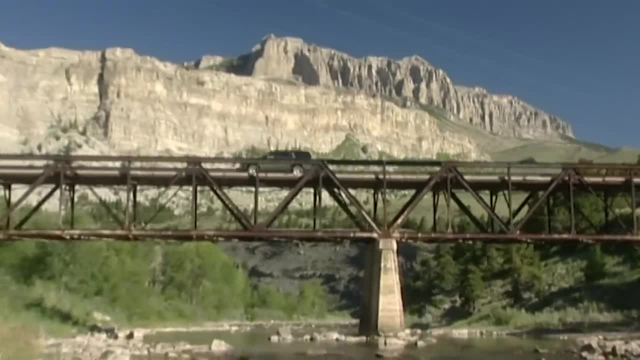 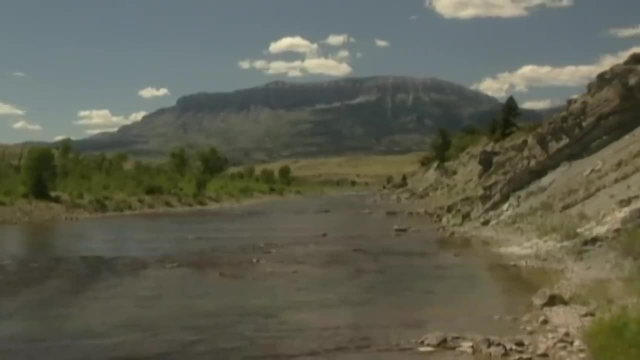 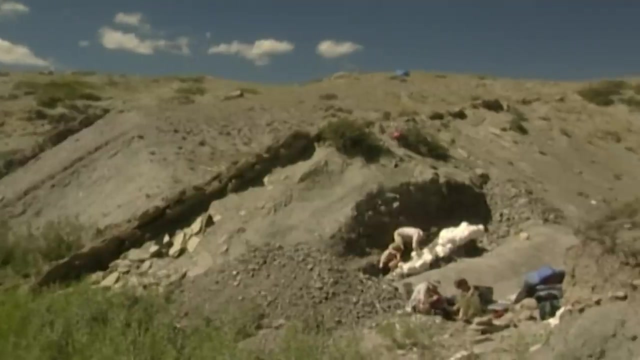 Its exact location's a closely guarded secret. It's been code-named the Bahamas and, although I can't see any beaches or yachts, it's a beautiful place. The site chief is Dave Vericchio. Have you got a dinosaur to show us? 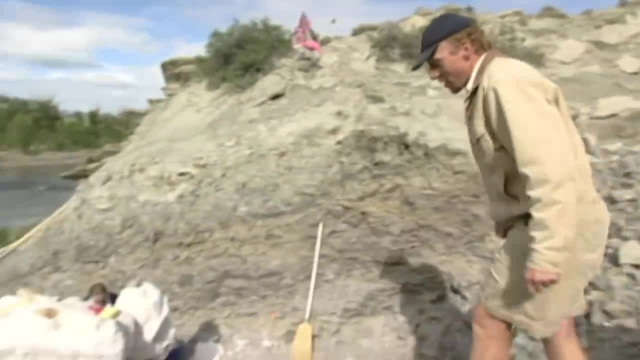 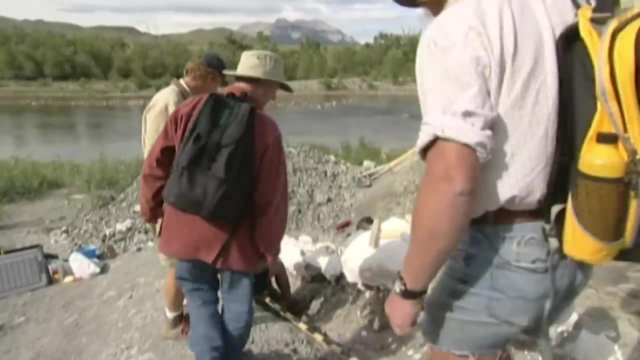 We do. We do A little bit of one. anyway, This is our quarry. here We're working on a Tyrannosaurid. It's a large predatory dinosaur from about 75 million years ago. Where is it? Where is it? 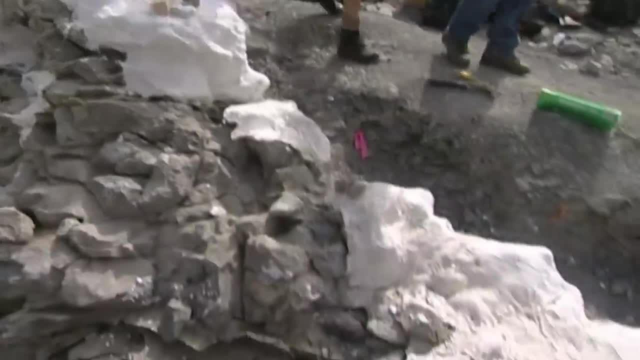 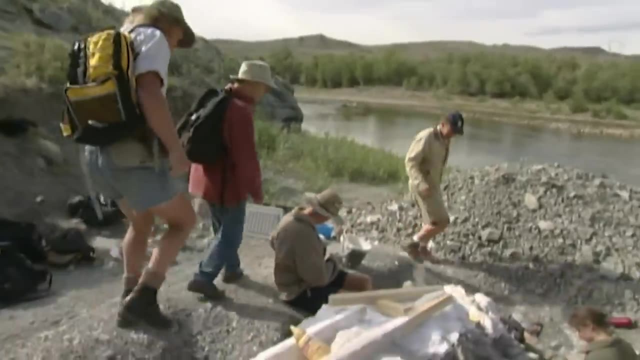 It's in our plaster jackets? It certainly is. It looks like it's broken every bone in its body. There's a bit of bone poking out here and there. Here's a metatarsal. That's one of the long bones in the foot. 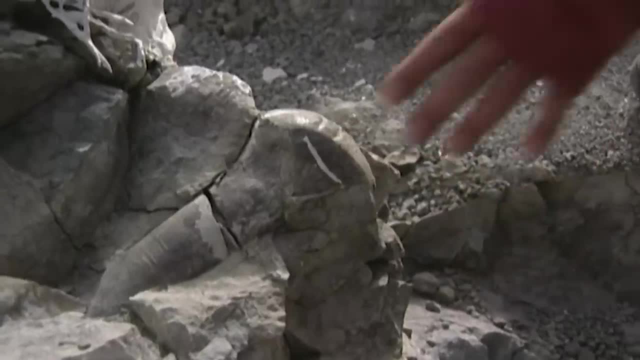 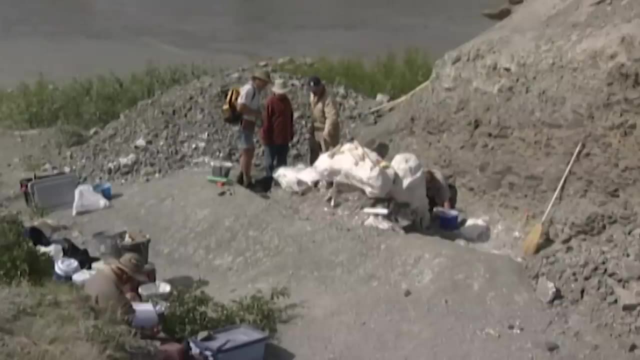 Oh, yes, You can certainly see that. See that, Phil? Yeah, Our first dinosaur bone. Dave, how much of the actual skeleton is here? This area has most of the skull parts, This big sort of mound in the middle. there has lots of vertebrae and ribs and then portions. 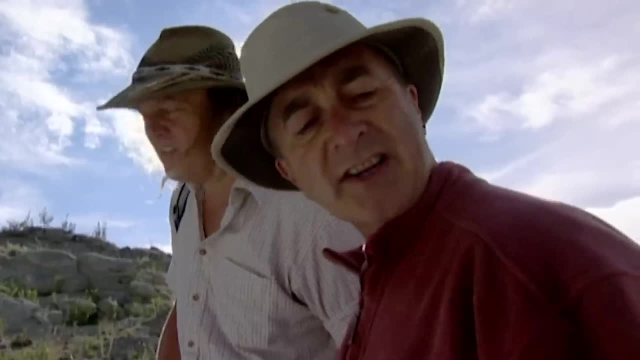 of the pelvis, we remove from the skull, That's right, And then we remove the spine from the back, And you called it a Tyrannosaurid. Yeah, It's a member of the Tyrannosaurid family. Which one is it? 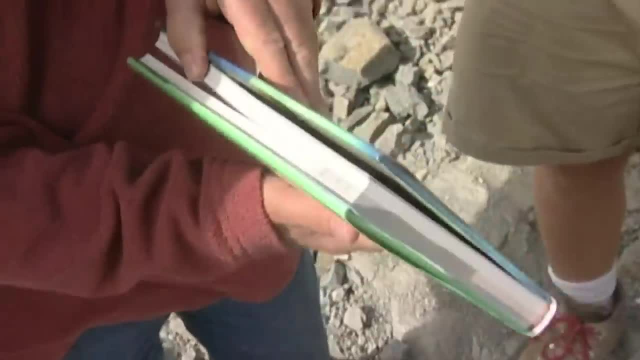 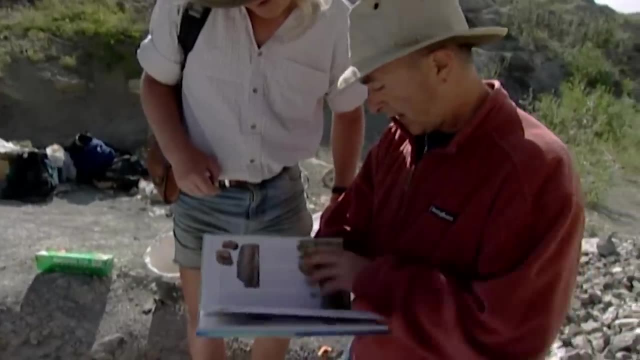 We're not exactly sure, but it's probably something like an Albertosaurus or a Displetosaurus, An Albertosaurus Sort of smaller cousins of a Tyrannosaurus rex. Oh, here's an Albertosaurus. So that's more or less what we've got. 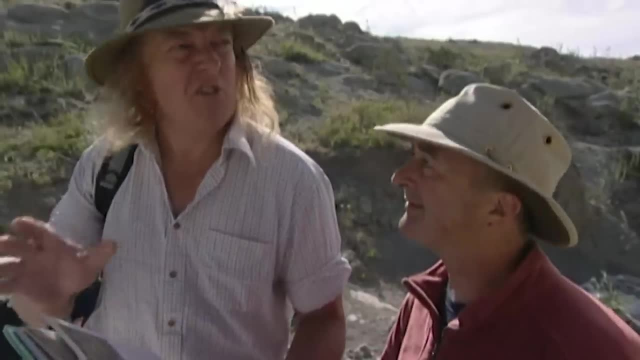 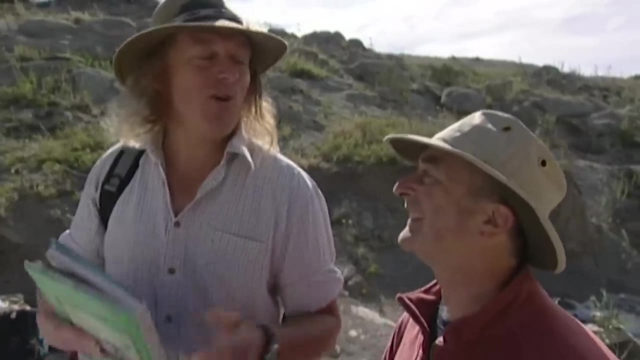 Mm-hmm, But is it actually articulated? No, it's all disarticulated. It's just a big jumble of bones. Yeah, Now you see Tony here. he was quite confident that we were actually going to come down here. 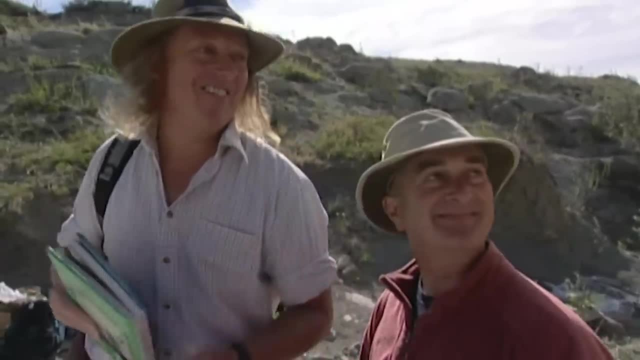 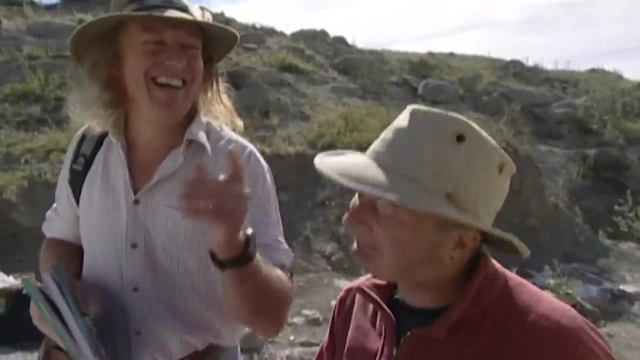 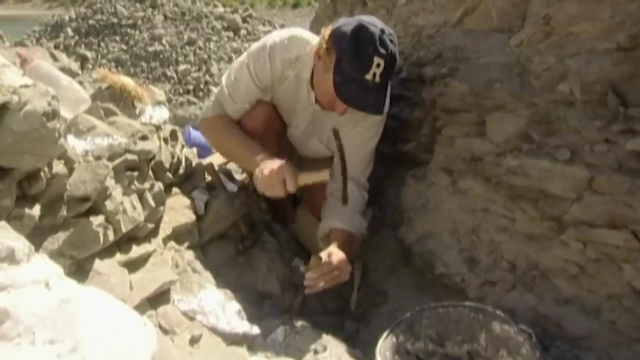 and there was going to be this massive dinosaur laid out in front of us. I thought we'd have a rock face just like this, and then you'd see this reclining dinosaur. I think that's in the movies. The digging process is a bit of a surprise too. 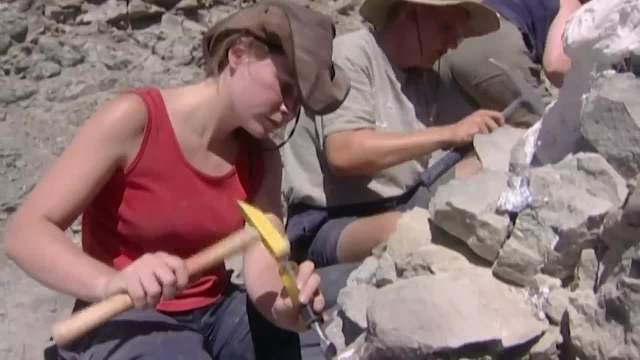 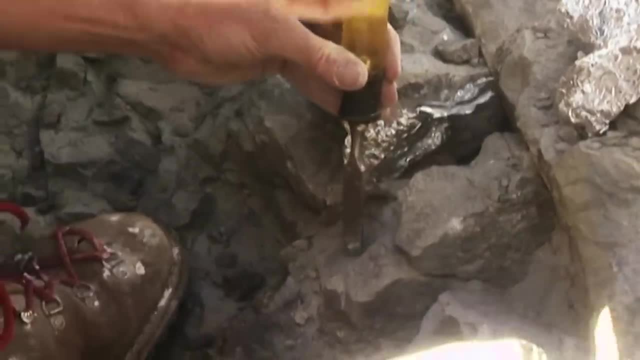 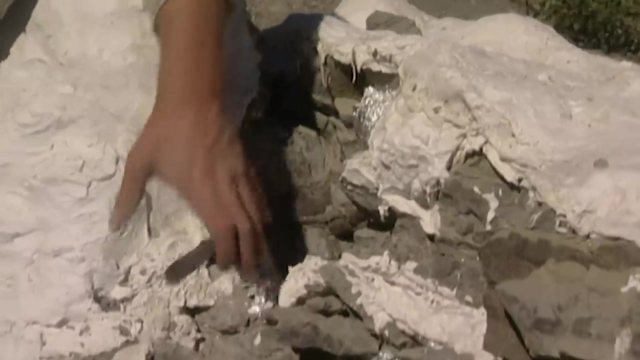 I'd expected to see the paleontologists carefully excavating each bone, cleaning the rock off it as they went until they could lift it pristine and intact. But the bones are extremely delicate, so the idea is to leave as much rock on them as possible. 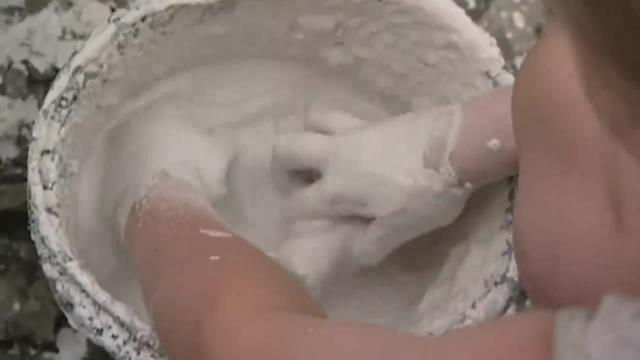 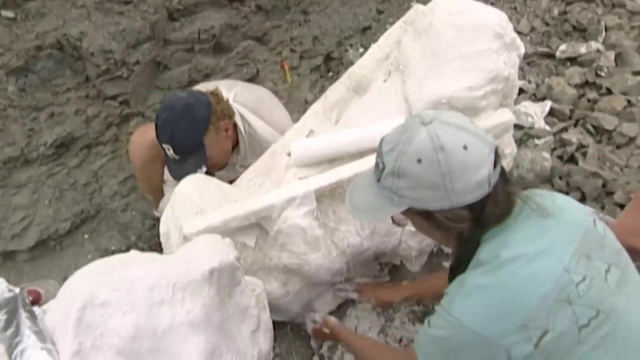 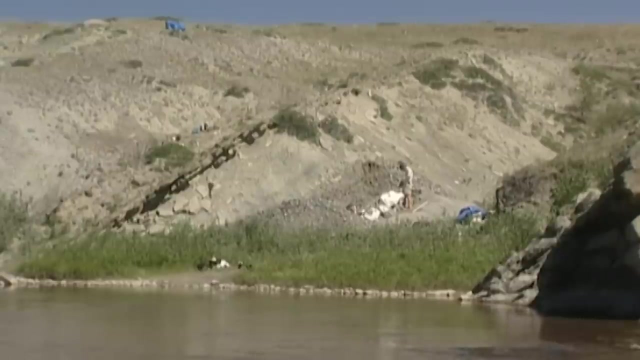 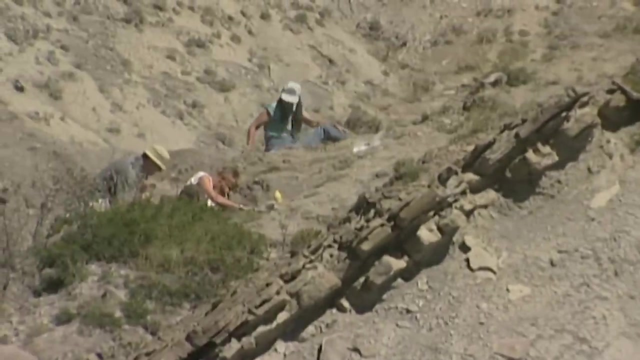 record how they lie, then wrap them in plaster jackets for extra protection. No one really gets to see the bones in their naked glory until they're cleaned up in the labs. The Tyrannosaurid isn't the only dinosaur on this site. Next door to the predator, Dave's found its prey. 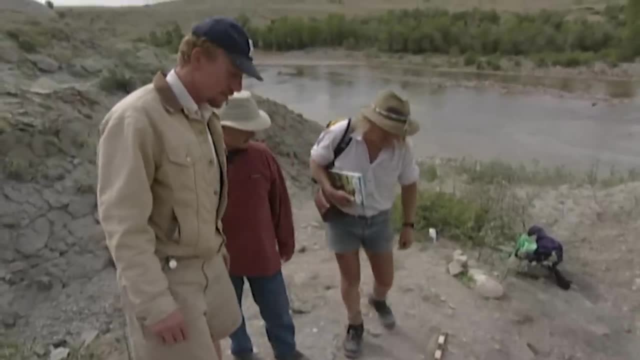 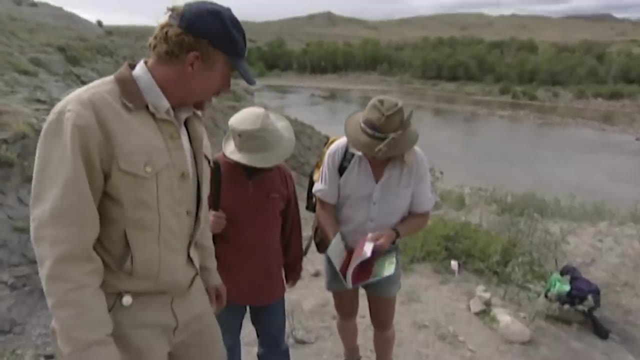 We have a jumble of hadrosaur bones from probably many individuals, all sort of tossed together in sediments. Hadrosaur, Hadrosaur- Look up in the book. It's like a duck-billed dinosaur. This one actually might be closer to a lambiosaurus. 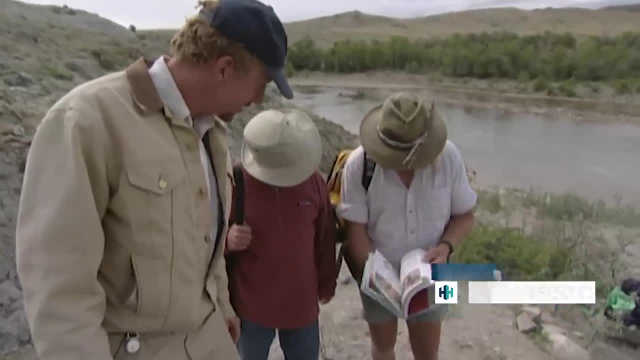 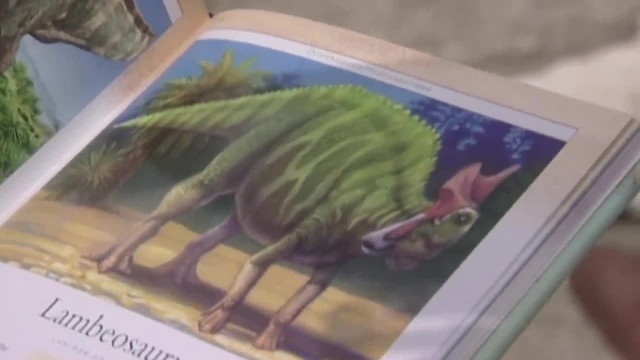 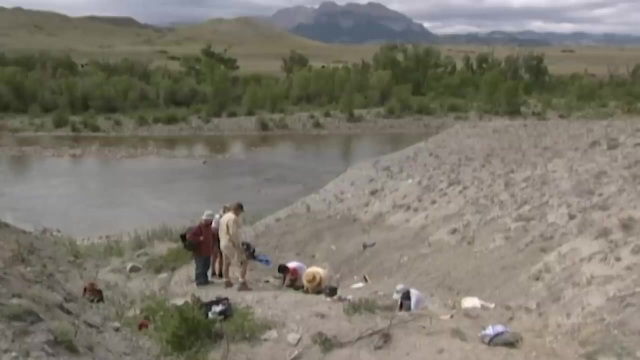 Oh, there he is, 187.. That, Oh, come on, You get taxpayers' money to find something like that. Yeah, they get a lot of it. It's vivid on the page and, unlike the Tyrannosaurid, its bones are vivid in the ground. 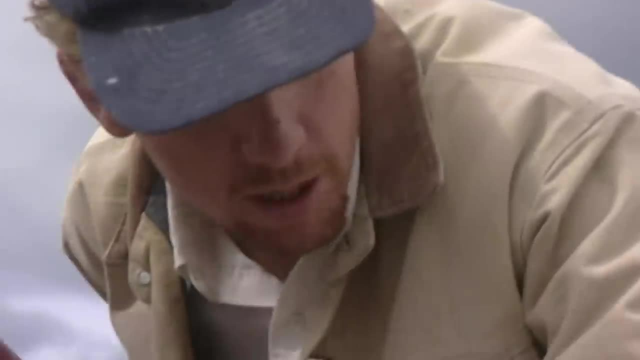 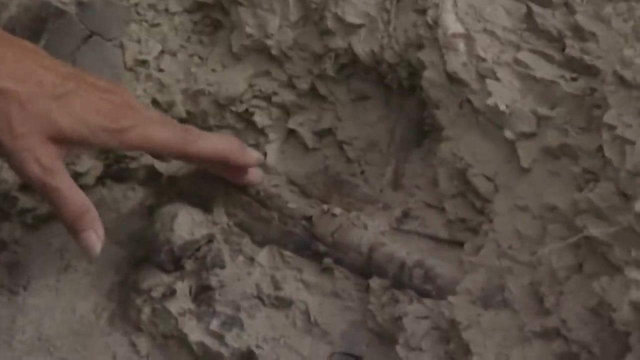 Oh wow. What exactly have we got there, Dave? The big bone on the left is the femur. It's one of the large bones from the thigh, And then that kind of long one cutting across is the ulna. 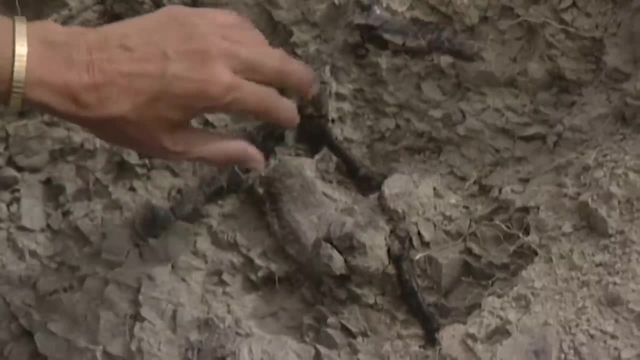 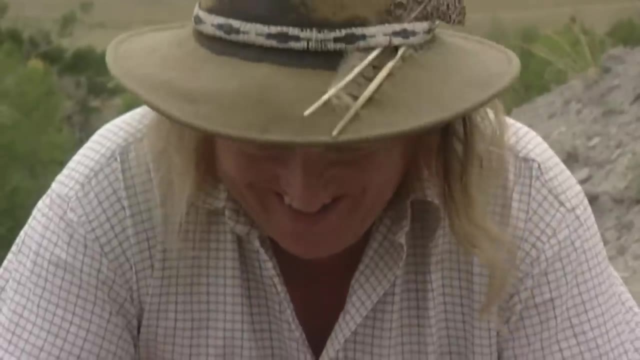 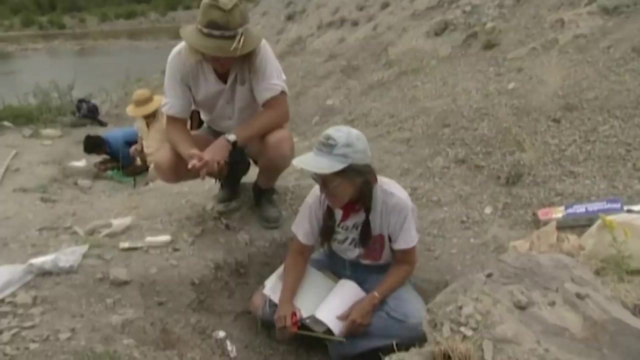 We've got a rib coming across here and a vertebrae. It might seem incredibly rude, but I've done quite a bit of digging. Ah, okay, Is there any chance that you would let me have a go on your site? Sure, you bet. 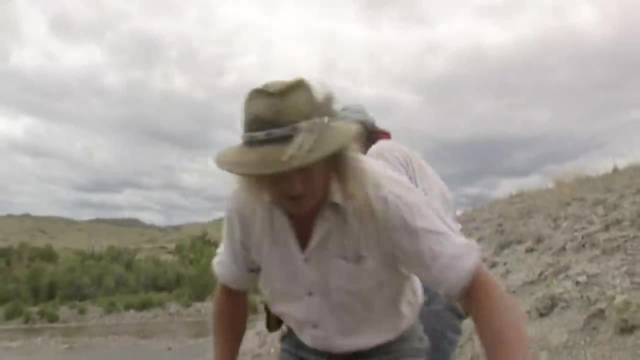 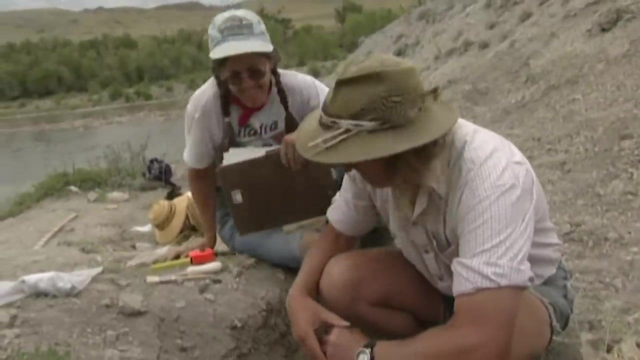 Problem. Yeah, that's just what I mean. if you're an excavator, you want to try and do as much as you can in different types of circumstances. Firstly, what am I going to be using? Okay, these are the tools. 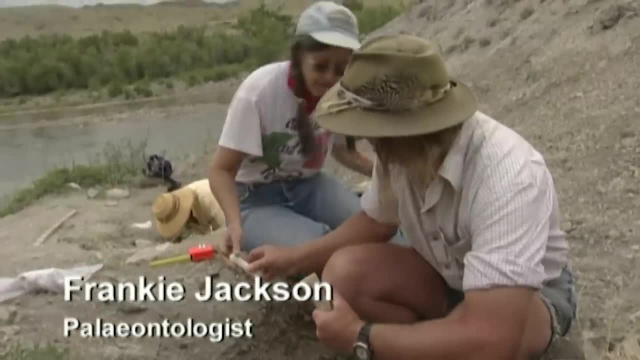 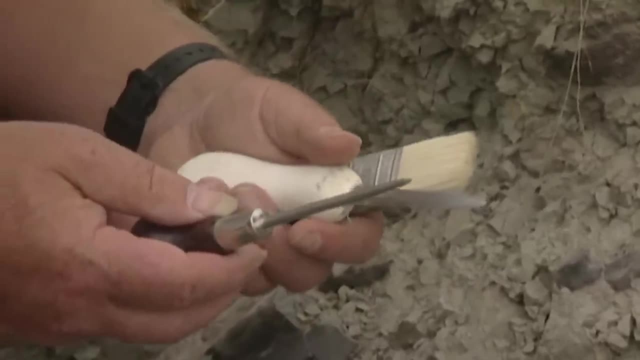 Paintbrush. I can understand that, Yeah, and you can have your choice. That's an oyster knife actually. Yeah, it's a traditional hole, So I'm not going to need my trowel after all. then 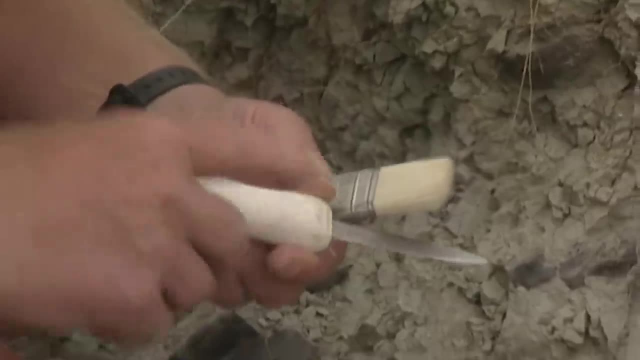 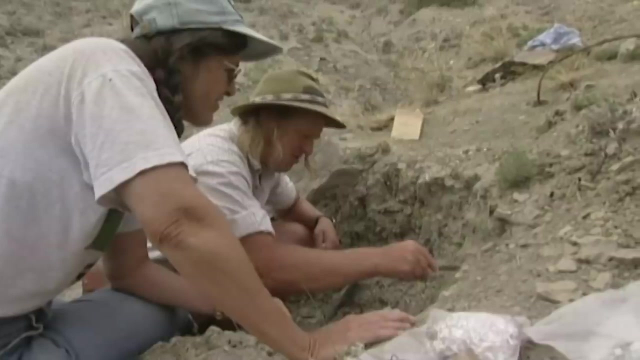 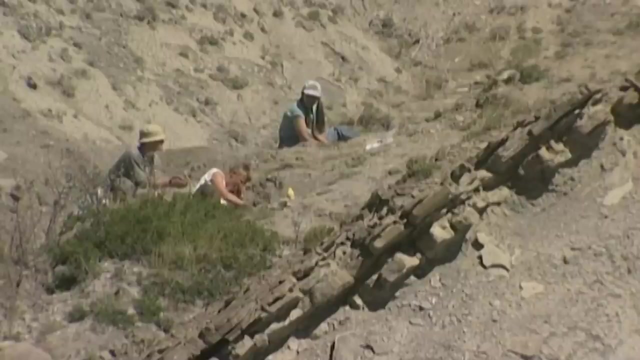 No, I don't think so, So you could just start up here and then start teasing it off. I mean, the first thing that strikes me is that it's incredibly crumbly Right Indeed, Although the two sites are close to each other geographically and in time. 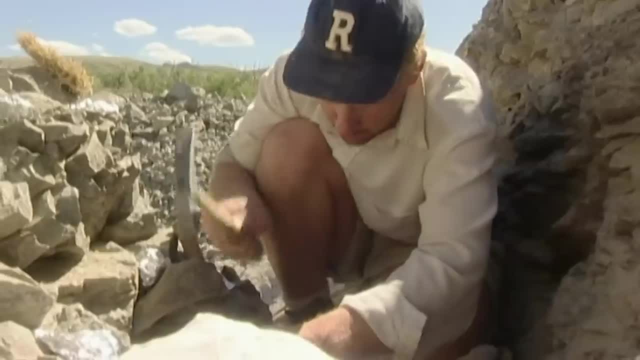 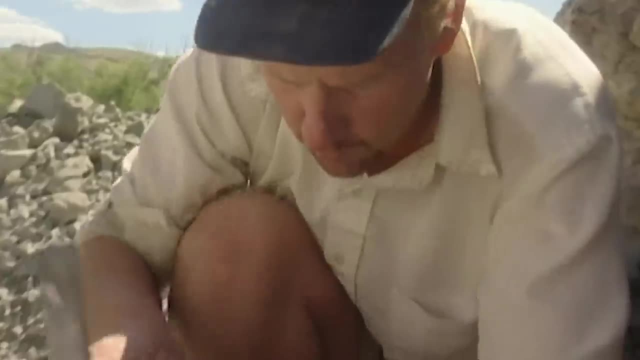 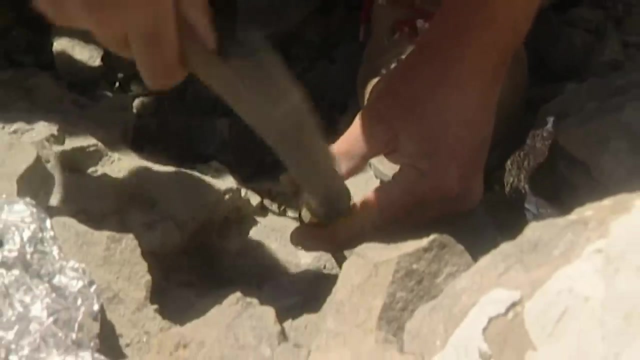 they demand different techniques. The Tyrannosaurid bones are densely packed and the rock encasing them is very hard. It would be impossible to extract them one by one, so the paleontologists are simply trying to separate them into manageable blocks which they'll remove later. 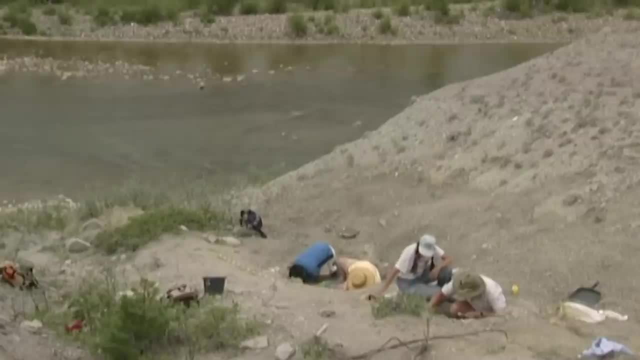 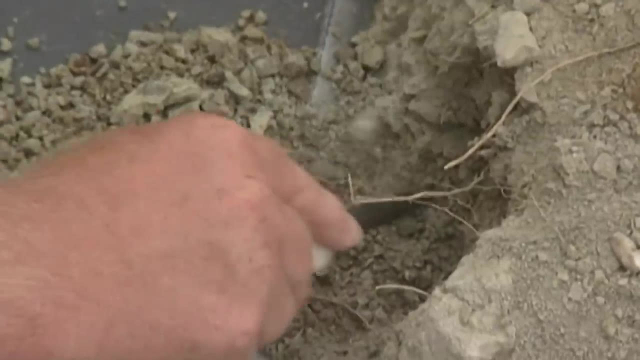 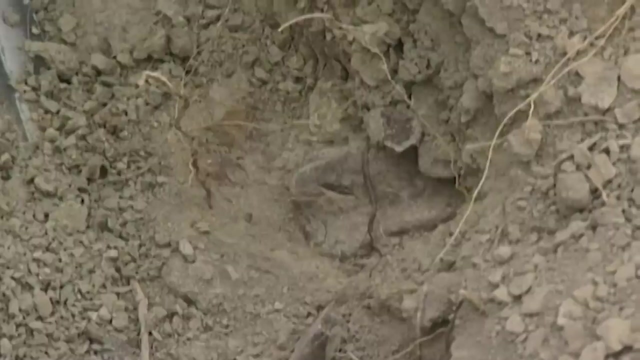 But at the Lambiasaur site it's much more like archaeology. The rock's no harder than soil and the bones are much easier to get at. It's just a matter of scraping till you find one. Oh, look at that. 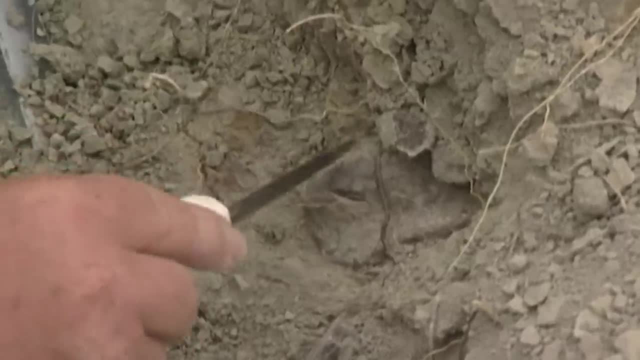 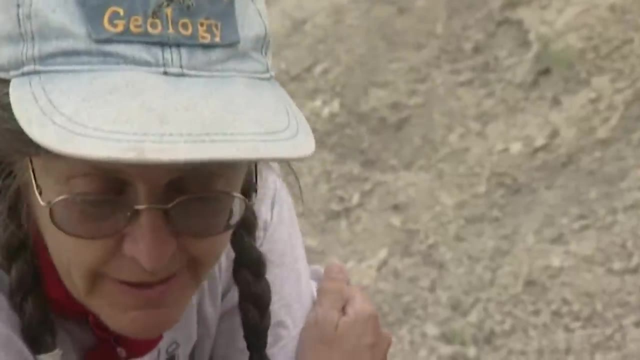 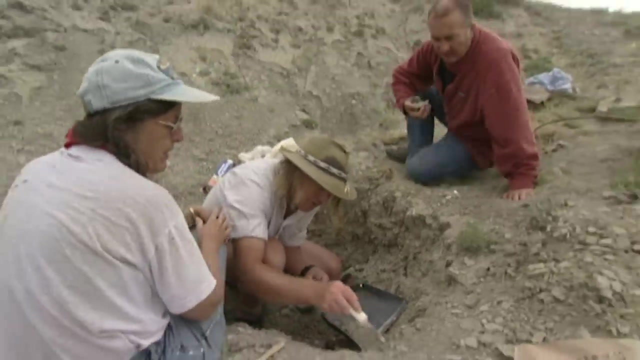 Is that bone? It's got to be bone. Oh, it's getting bigger. Centrum: This is gas right now. OK, so what's the centrum? It's the centre of the vertebrae. Phil's obviously delighted to have found his first-ever dinosaur bone. 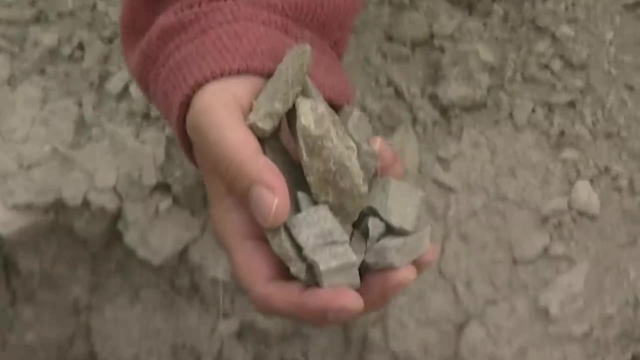 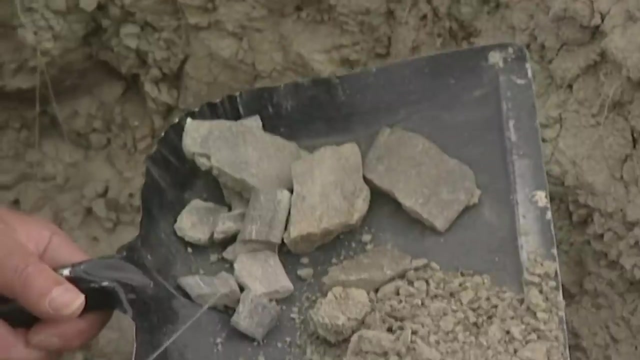 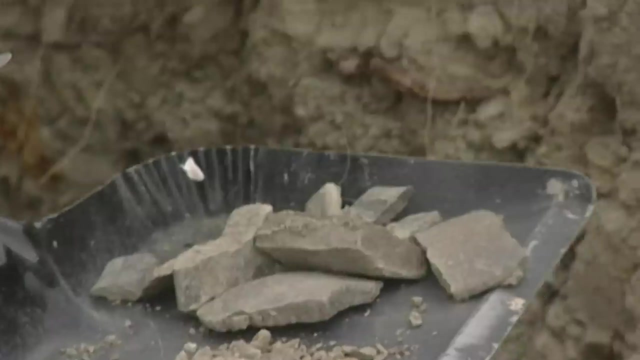 but it's taken him a good hour And in the meantime I've been wandering about the site and found all these, Frankie, are they rocks or are they bones? They're bones, Hadrosaur bones, Which makes the score about 10-1.. 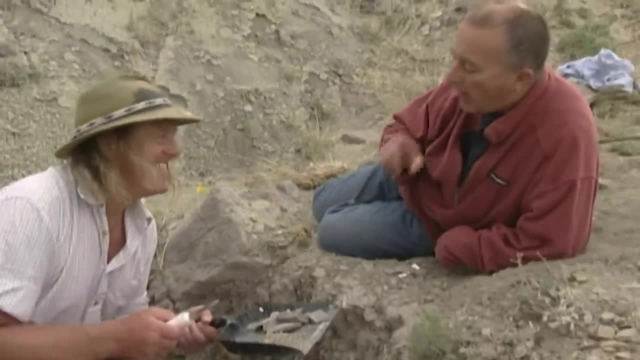 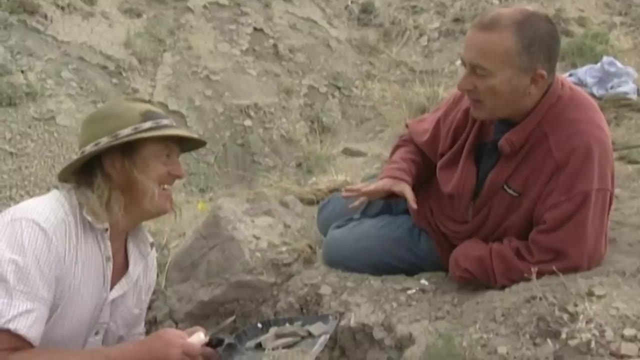 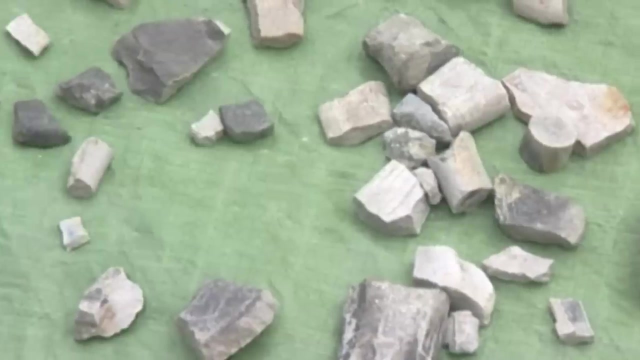 to me. What I'm beginning to realise is, when we first came up here, I thought that finding a single dinosaur bone would be something that was really rare. But we come up here. it's like a tray full of crisps. In fact, Dave and his team have found hundreds of bones. 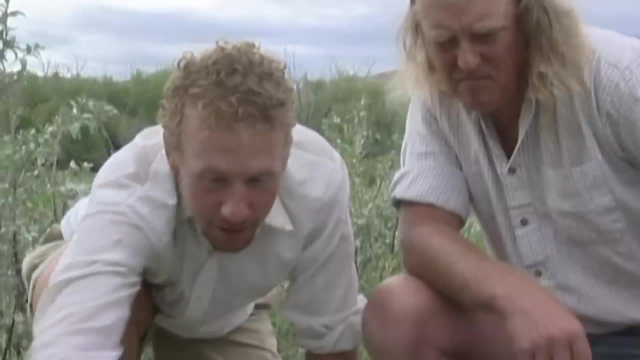 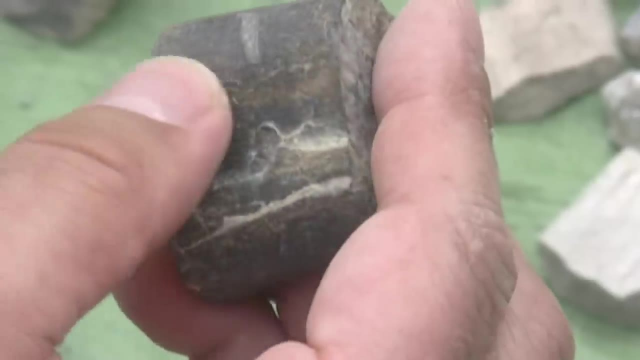 just lying on the surface, And they're full of valuable information. This one, for instance, has a tooth on it Suggesting that the lambiosaurs were lunch for a predator. Any idea how many lambiosaurs might be here? 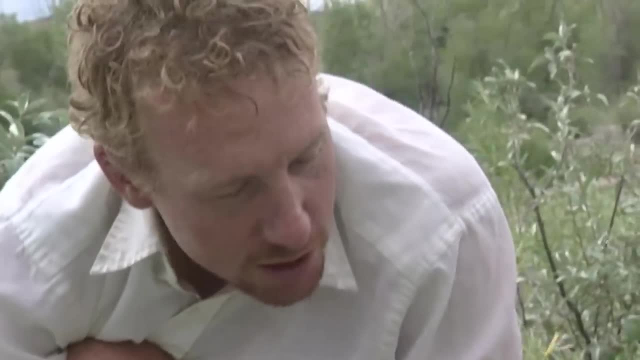 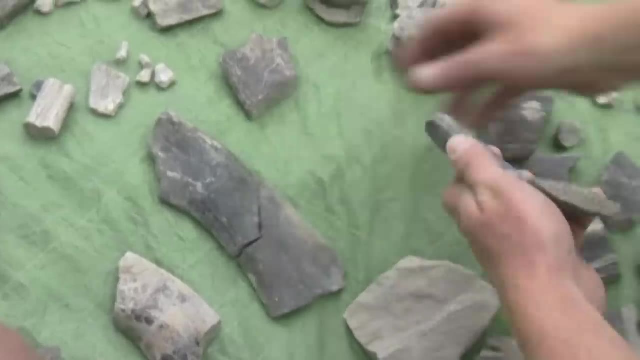 We have several individuals. Probably at least three are represented here. These are scapula shoulder blades, So we have three of those. Can I have a feel? Yeah, Here you go, Tony. It's funny, isn't it? because bone is actually very light. 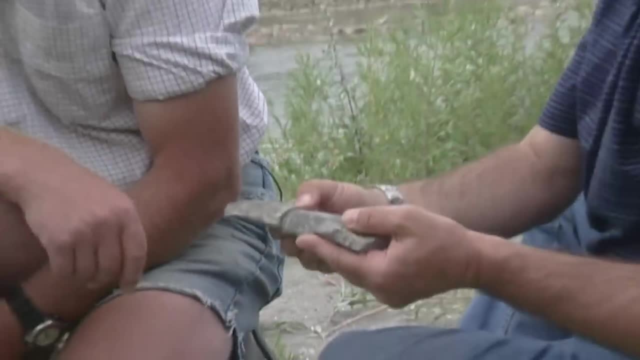 but this is definitely the weight of stone. That's just right. I mean, it's totally mineralised, isn't it? Yeah, It's totally mineralised, isn't it? The word we like to use is permineralised. 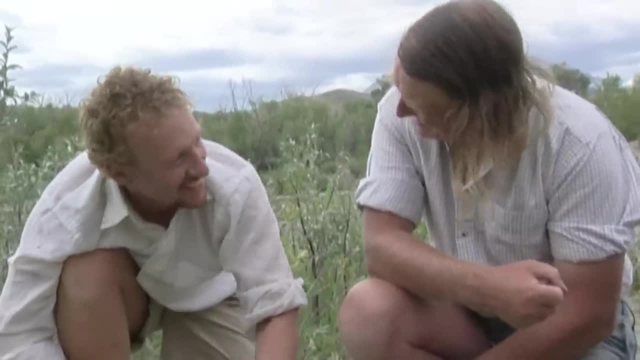 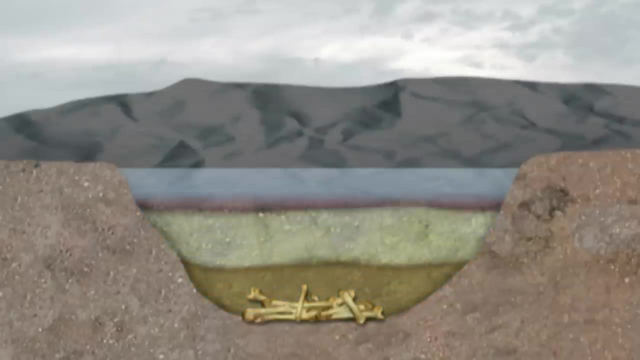 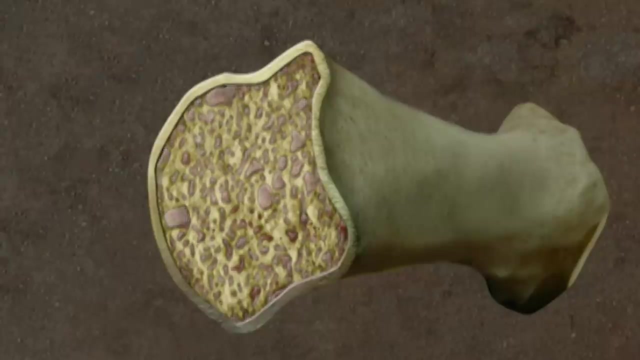 Permineralised- Yeah, if you can say it. Permineralisation happens when bones get rapidly covered by layers of sediment, often in streams or lakes. The organic material in the bone quickly decays, leaving a hard, sponge-like shell. 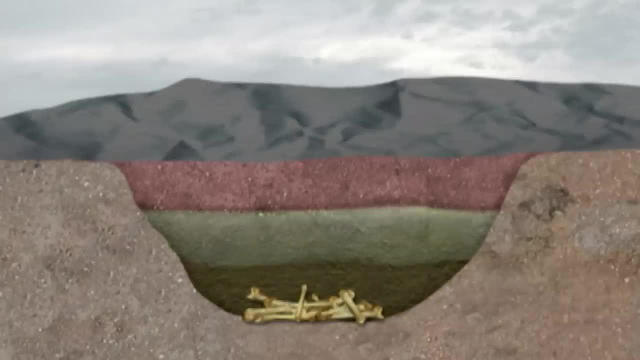 Over thousands, perhaps millions of years. the sediments gradually turn to rock. Groundwater percolates through it, leaving mineral deposits in the cavities of the bone. What you're left with is a fossil, a bone frame filled with rock. 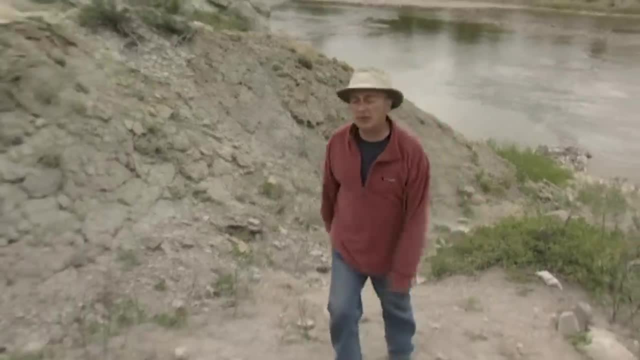 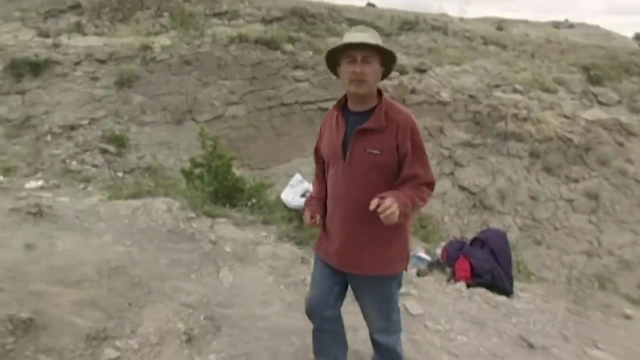 I've left Phil for about an hour and a half scraping away in his little trench, or quarry, as I now understand, paleontologists call it, And if we're doing archaeology, an hour and a half would be a perfectly adequate amount of time. 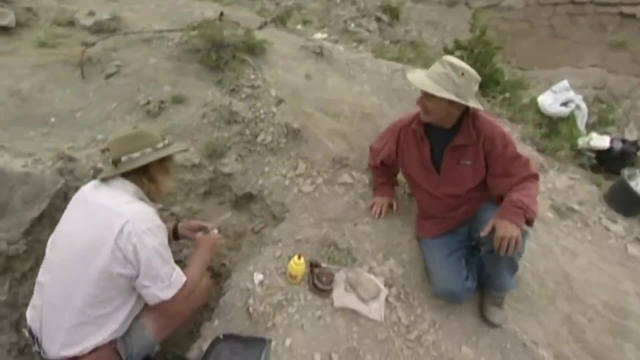 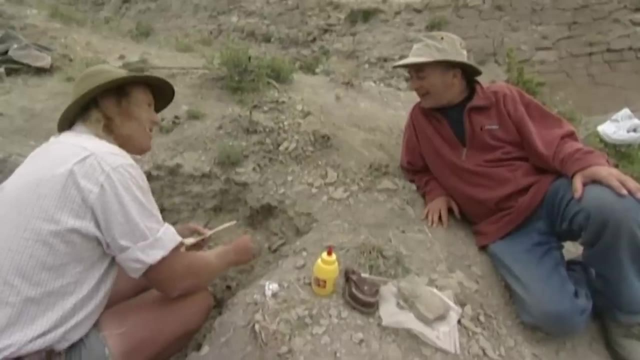 for him to come up with something good. How you done Really well, Tony. What do you think of that? There's my bone, Do you remember that? Yeah, but it's about an inch bigger than it was when I was here last. 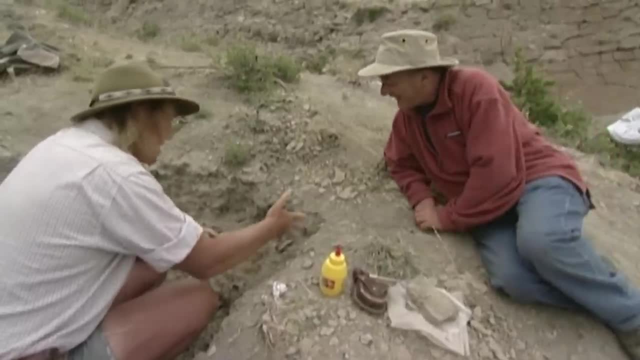 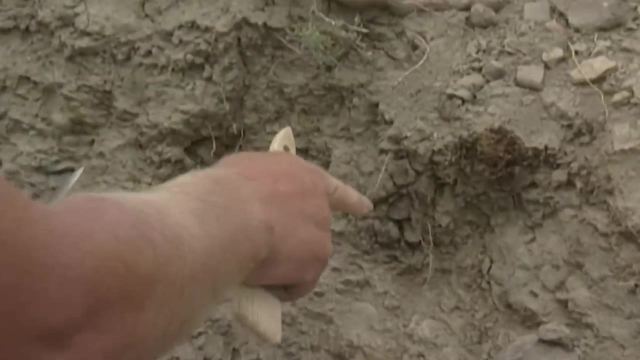 It is enormous. I've exposed it all the way round. I had to clear a lot of dirt all the way round there, clear me away along here and in the process, look, I found a load more bones in there. I mean, this is a very slow, painstaking business. 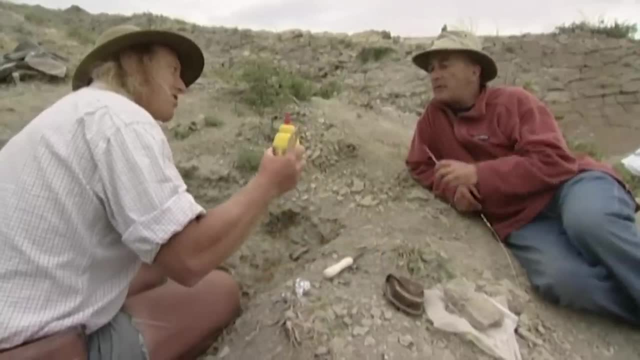 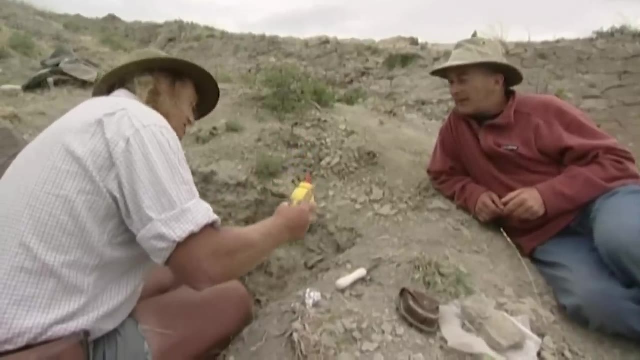 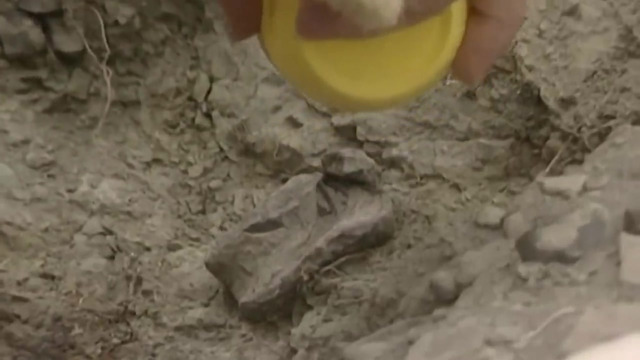 One more process. Why have you got mustard? There is no meat left on that bone. This container, this container is full up with a hardener, Tony, because that bone is so delicate, So I'm about to pour some hardener on it. 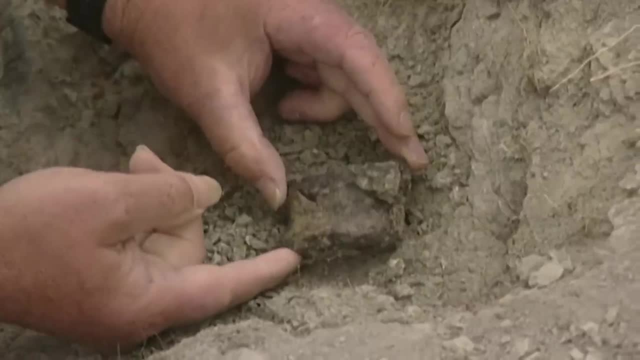 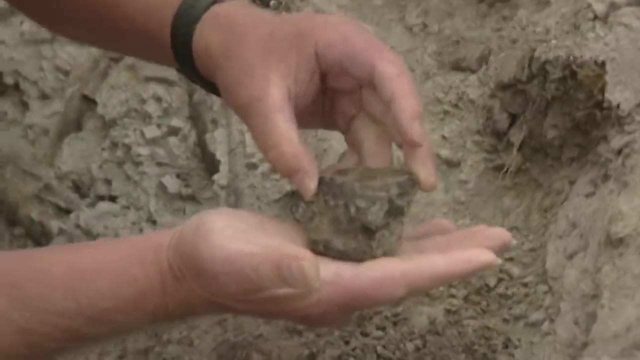 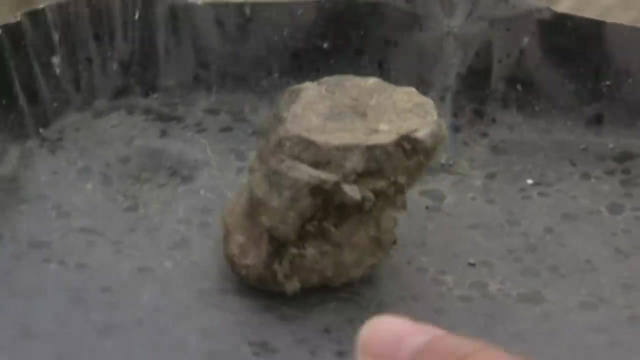 That's about got it covered, Is that it? Yeah, Our first day of dinosaur hunting? Hey, how about that then? has been a success. Phil's bagged a lambiosaur, 74 and a half million years older than anything he's excavated before. 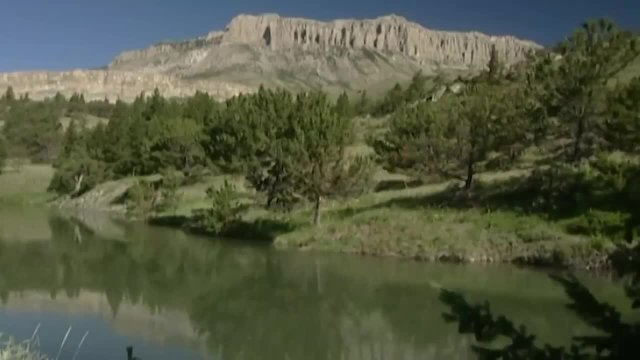 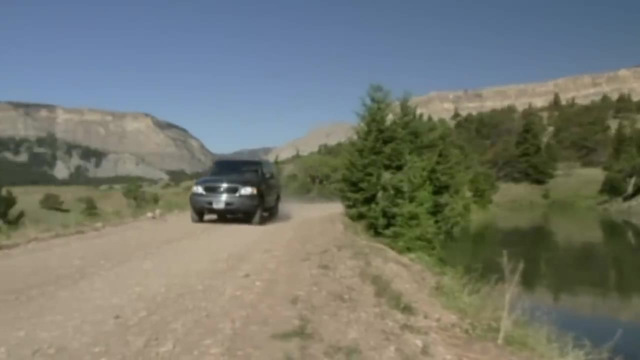 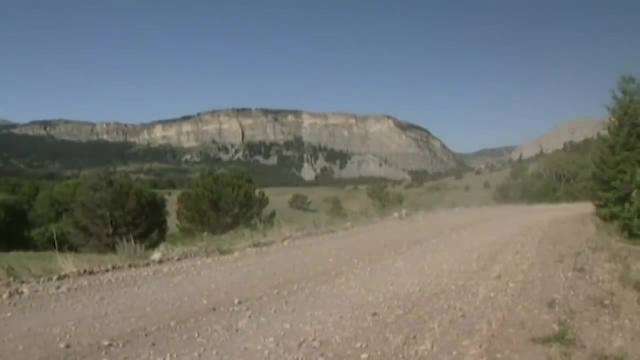 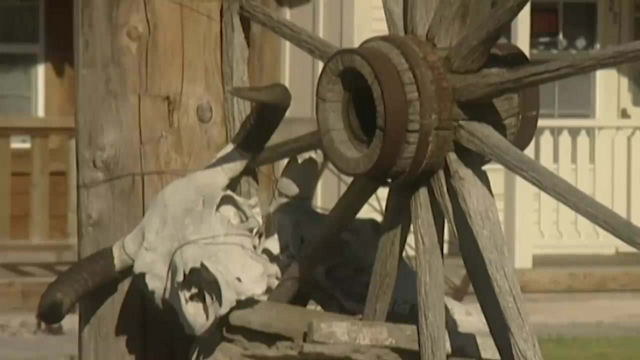 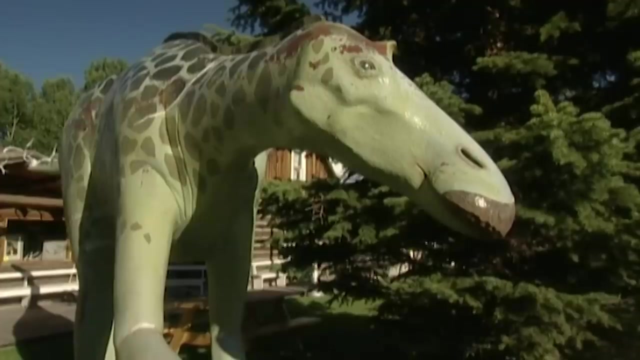 Well done, mate, But tomorrow it's my turn. We're going to a brand new site and I've been promised a crack at a good old-fashioned predator. Join us after the break. This is Choteau, a small town just down the road. 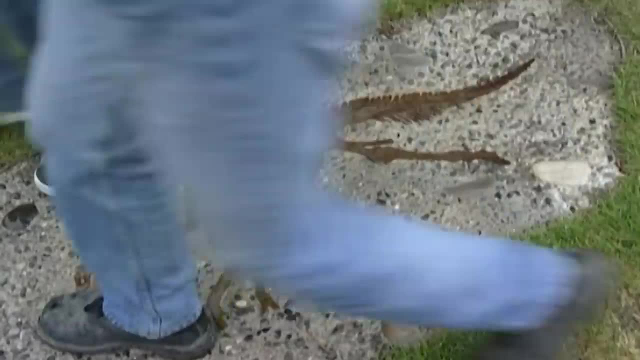 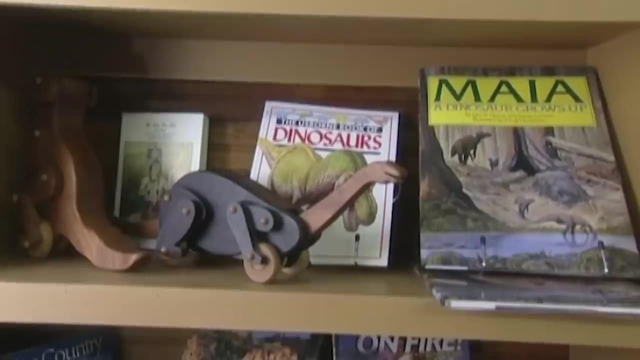 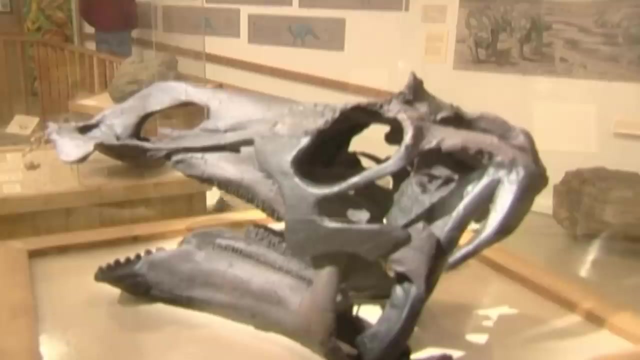 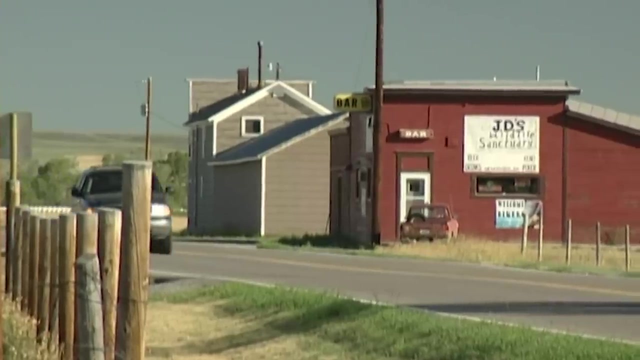 from the Bahamas dig. It's at the heart of the Montana dinosaur belt. If you're into dinos, this is the place to be, Which is all very well for the armchair dinosaur hunter, but Phil and I are looking for something a bit more hands-on. 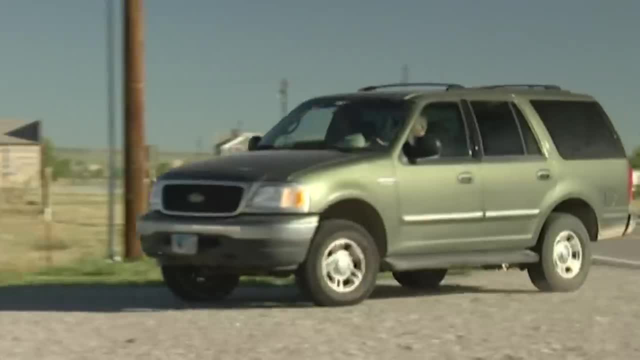 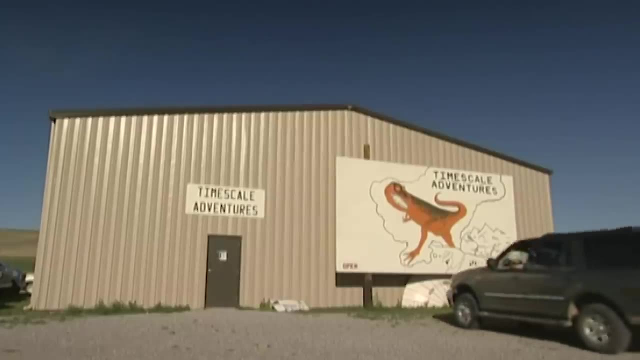 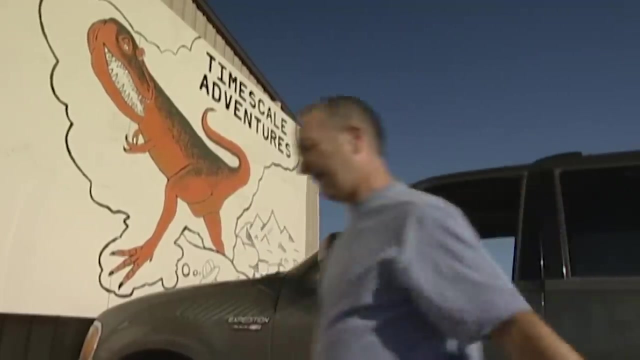 And in a one-horse town a few miles up the road. we've found it At Timescale Adventures. members of the public can sign up for a day, a week or a fortnight of hardcore dino hunting. It's a neat idea. 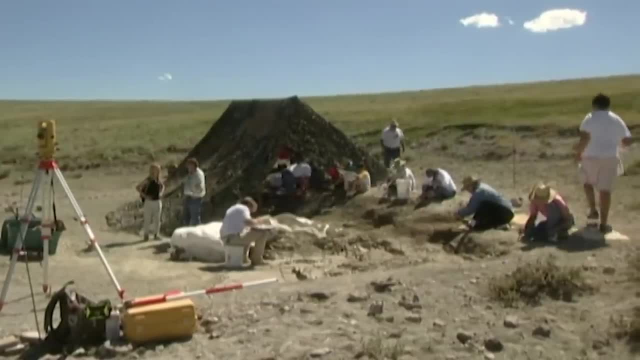 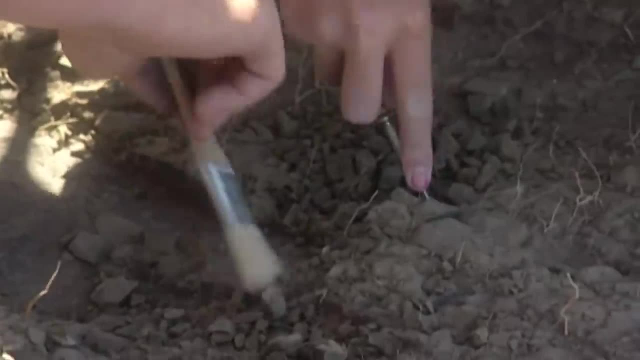 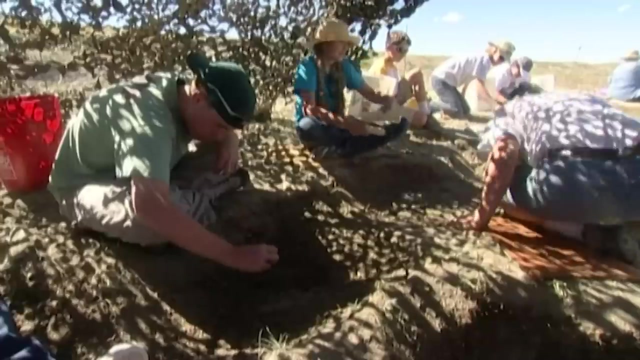 Paleontologists, like archaeologists, are always complaining about lack of funds, but not Timescale boss Dave Trexler. These people have all paid him good money to come and help him dig up his dinosaurs. In return, they get a basic training. 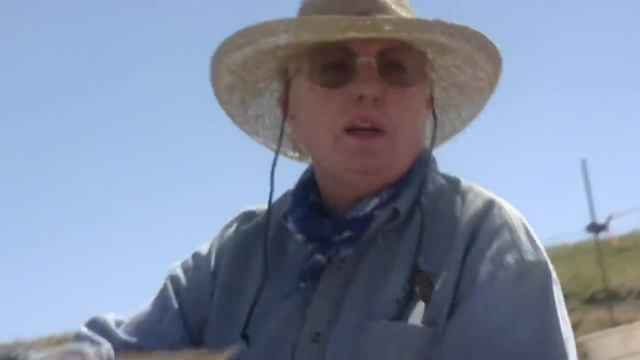 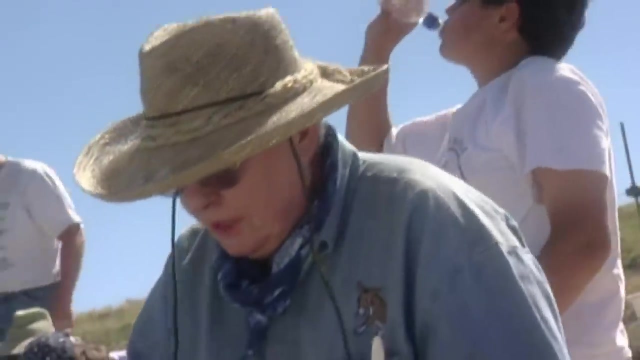 in paleontology. It's a really good opportunity because you know there's not many places you can go as a layperson to to act. They actually dig bones. They won't let you on the sites And dinosaurs to me. 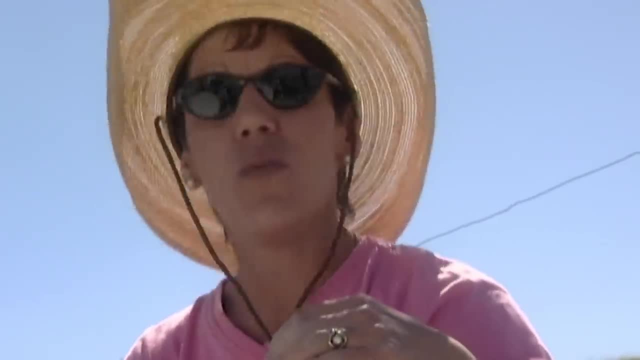 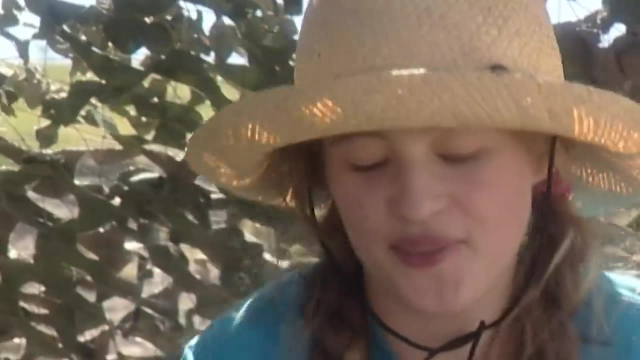 were almost like a myth, And so coming out here and actually seeing these bones and the process and how careful you have to be, it's just it's like a whole new world to me, So it's really exciting. It's pretty fun. 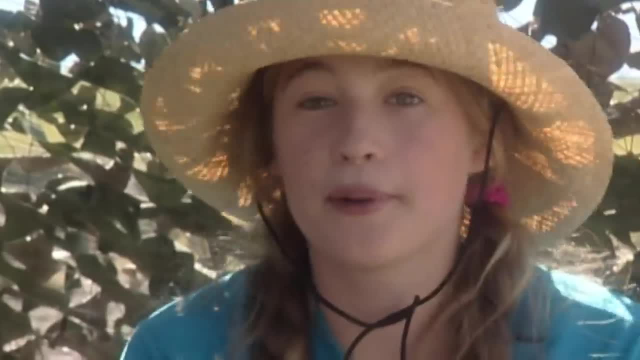 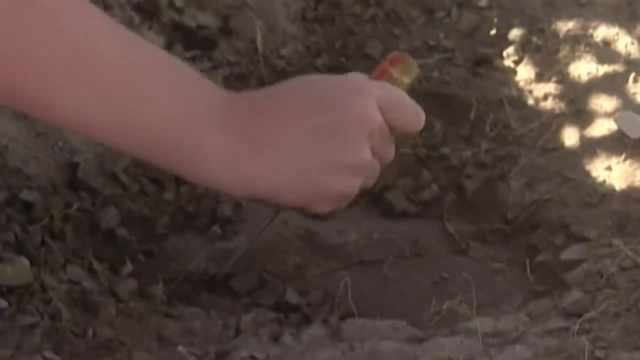 And I like doing this and I like doing the prep work like gluing the bones together. But, um, I don't know if I like to do it as a profession, but it's pretty fun just to do it and come out here. 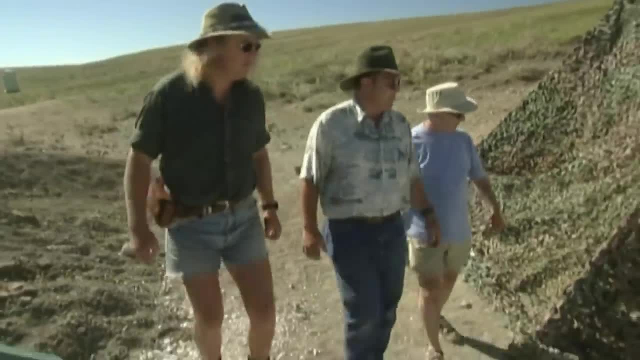 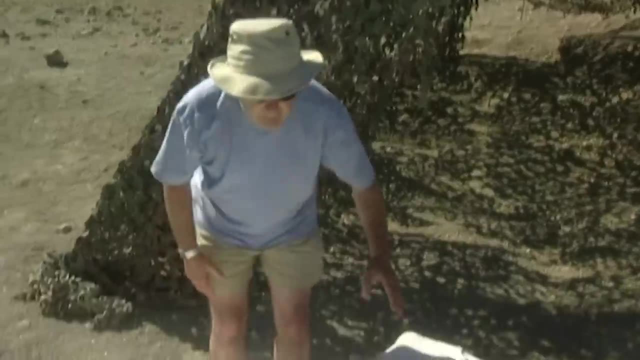 Phil and I can only spare a day, But we've got this bit of the site to ourselves And the hunting looks great. There's a heck of a lot of bone here, Dave. There's bone all the way down here, all the way down there. 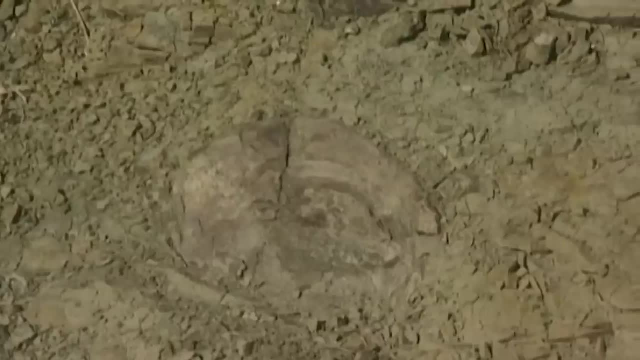 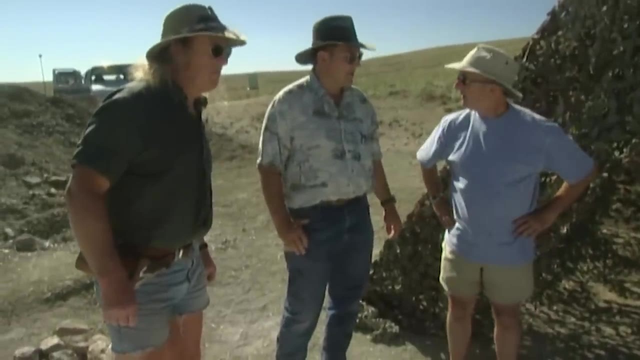 There's bone over there, bone right over there, bone there, bone there, bone there. What have you got here? We have the remains of at least eight individuals in this quarry, Two different types of dinosaurs. Five of the individuals are duck-billed dinosaurs. 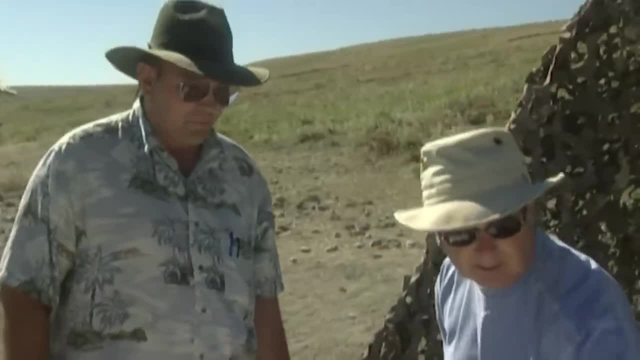 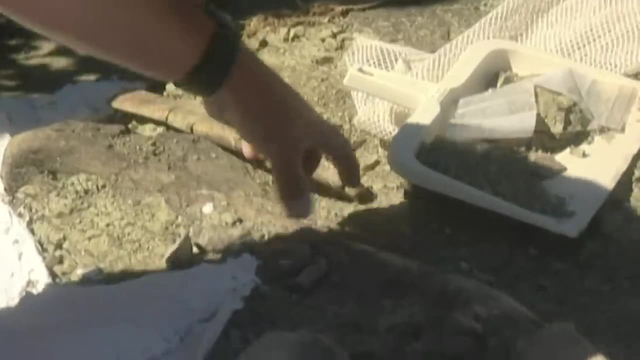 and three of them are Tyrannosaurid. And what do you think we've got here? This is actually part of the pelvis of one of the Tyrannosaurids. This is called the pubis bone. It's the part of the pelvis. 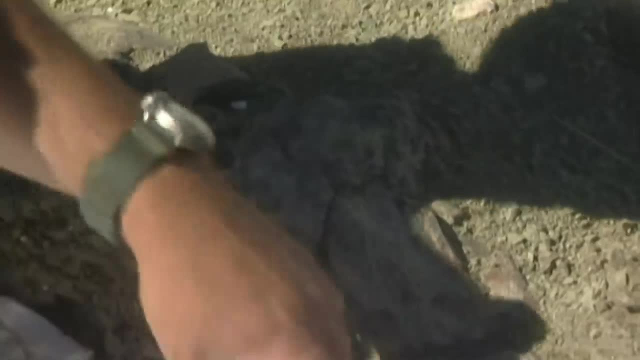 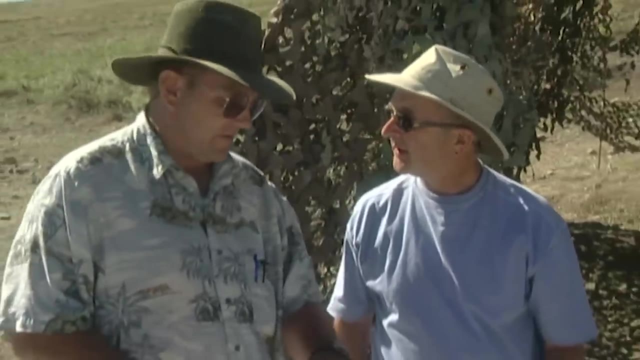 that sticks forward And this is part of the ilium which sticks over the top. So is this where we're going to start this morning? Actually, this area is very delicate. That's the reason we're plastering around it. We're not to the point. 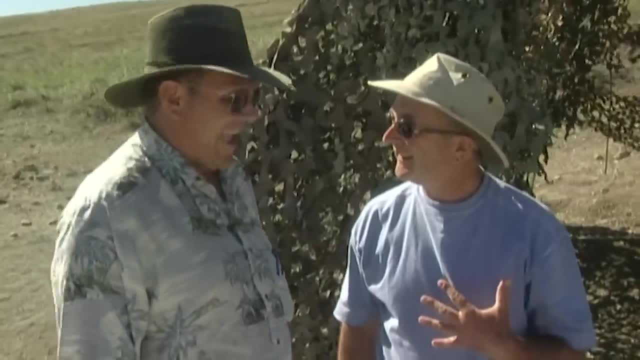 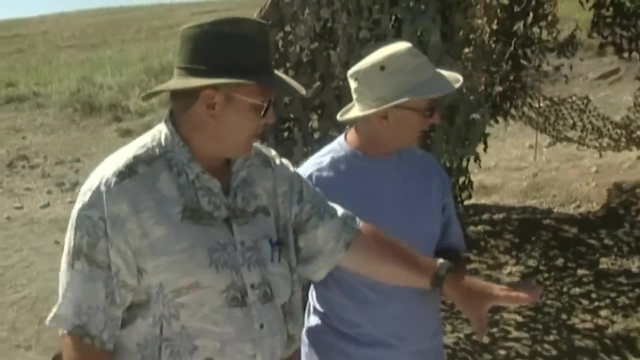 where we can work on this one. You're saying you don't trust me. Actually, I don't trust me. I refuse to work on there myself right now. What we will have you work on, though, is part of the animal back over here that we need to. 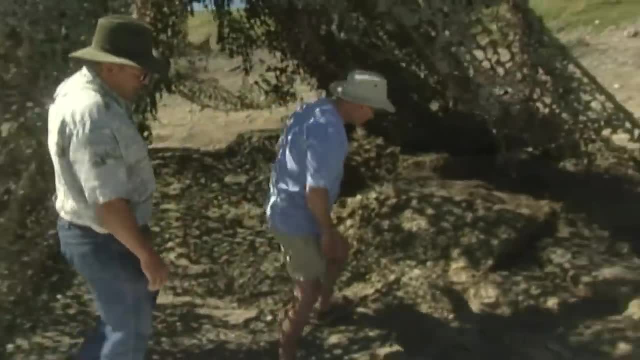 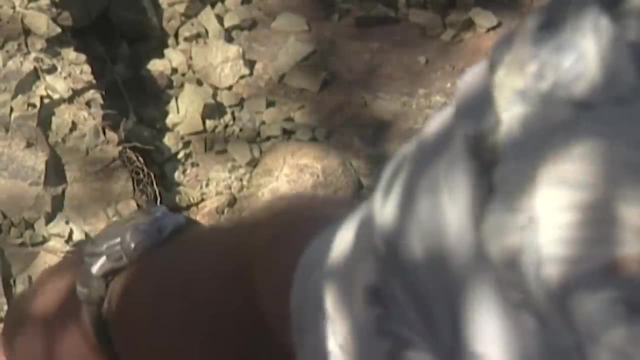 Dave wants us to work on an area he's only just started exploring. I can't see any bones, but Dave assures me under here somewhere is another Tyrannosaurid which is much better than Phil's sissy plant-eater. Phil, will you be very careful. 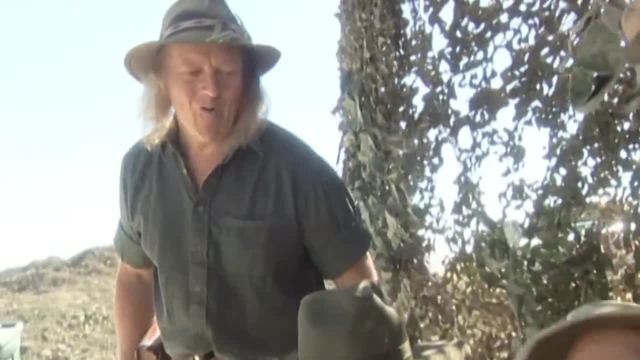 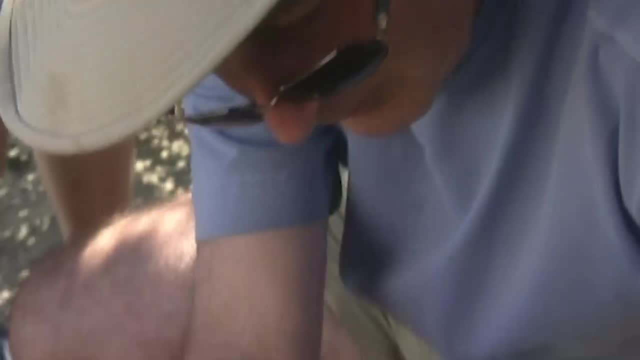 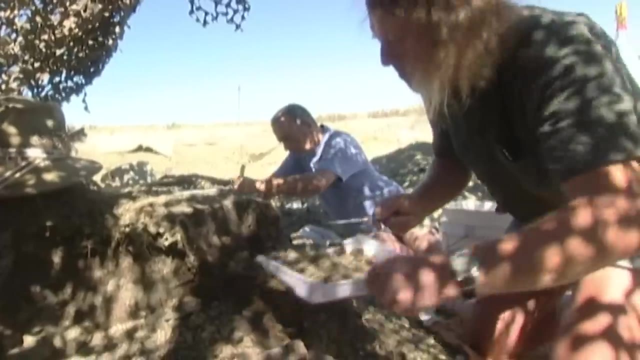 on the edge of my trench, please. Ten years I've wanted to say that You'll be using a brush and Dave gives me my tools, shows me where to scrape and I'm away. These are natural. I'm determined to find. 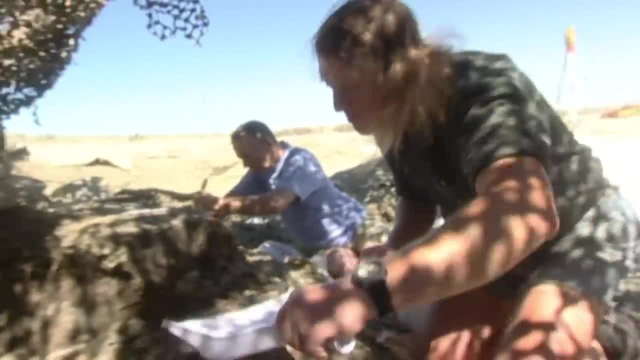 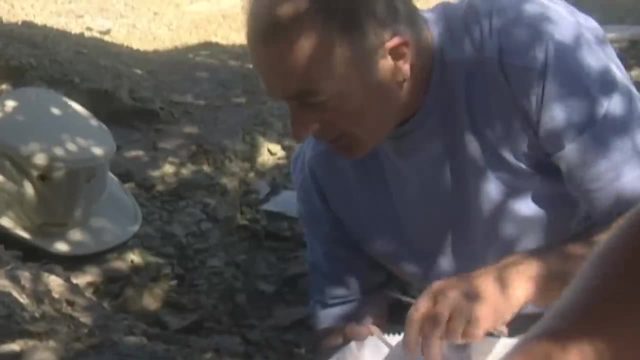 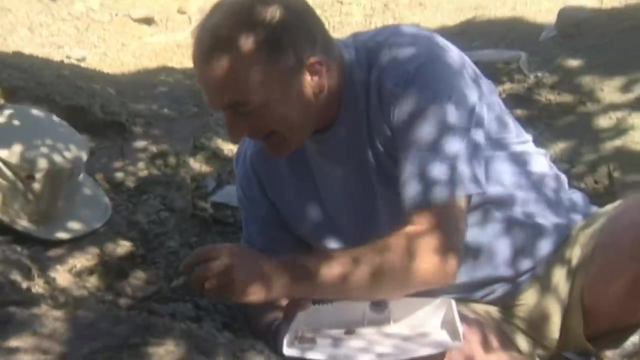 a bone before Phil, But it's several hours before I get a scent of my prey. I found a knobbly thing here And I don't know if it's bone or rock. Come and have a look. A knobbly thing. 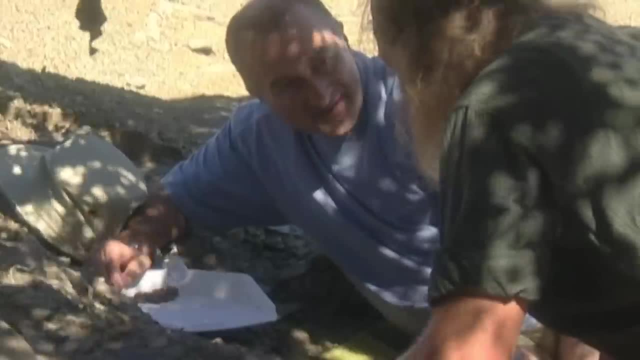 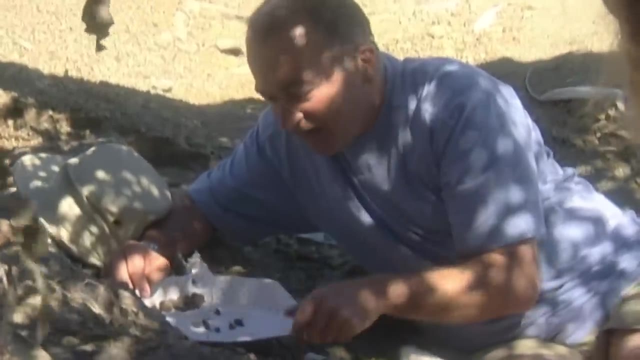 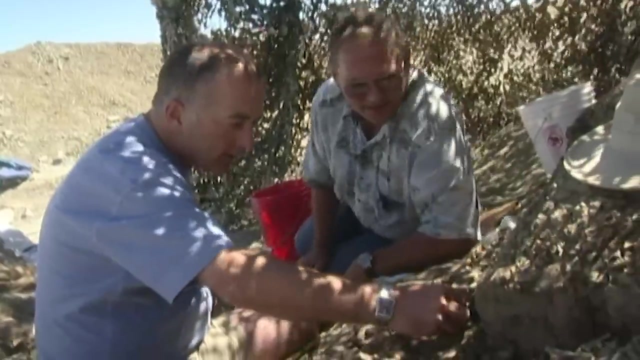 It's not what I call an academic Exciting. if it is bone, This is my bone. Is that? Will that be your first ever bone, In a manner of speaking? The bone and rock are so similar, though I need expert confirmation. 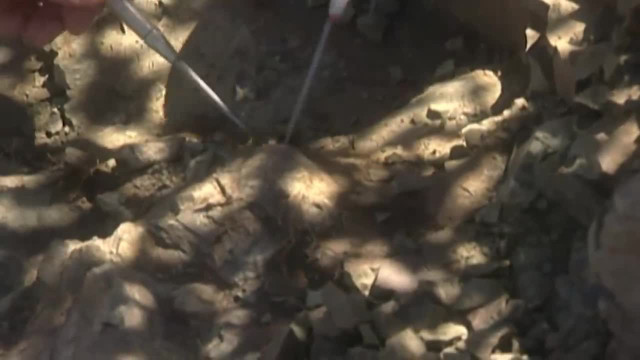 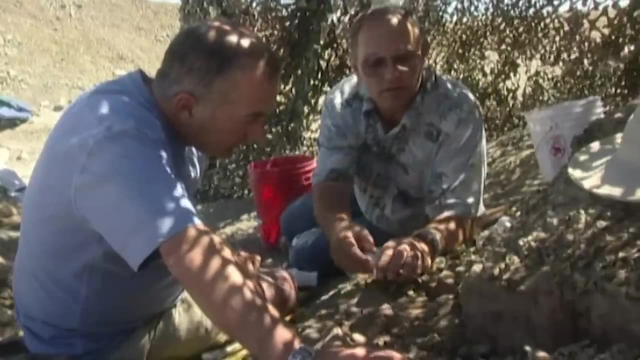 Do you think this is bone? This is all dinosaur bone right here. Yes, All the way around, It's bone. Phil Whoa. Well done, Tony, But I'm discovering what a slow process this is, After nearly a day. 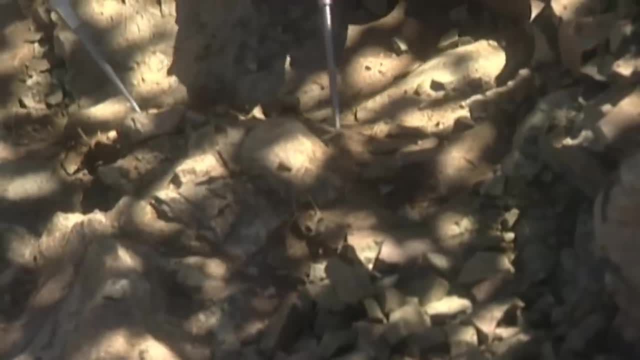 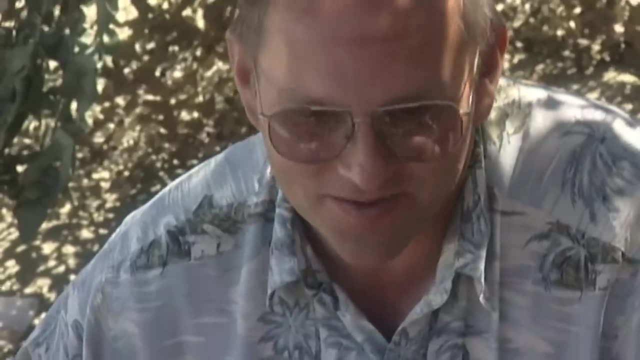 working at my new bone. it's still firmly rooted in the rock. I'm not going to be able to get this out, am I Not? today? Probably not. We're looking at a bone that is liable to take two days of excavation. 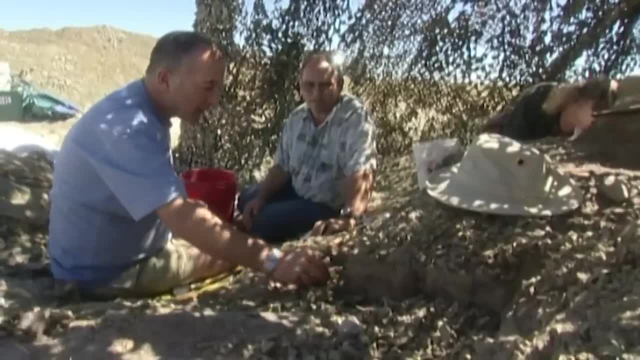 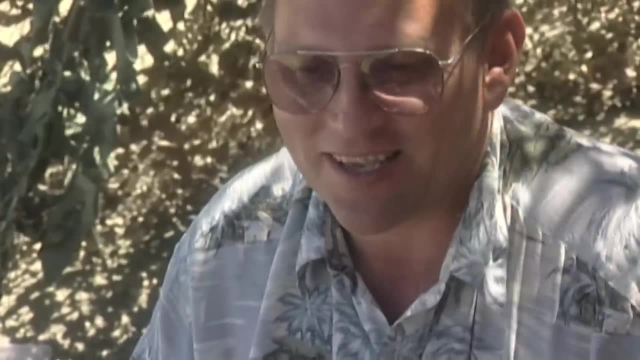 before it's ready to remove. OK, just speculation. What bone? What bone could this possibly be? from what kind of dinosaur? Of course, it's bad to guess, but it looks like it was the neck vertebrae of a tyrannosaur. 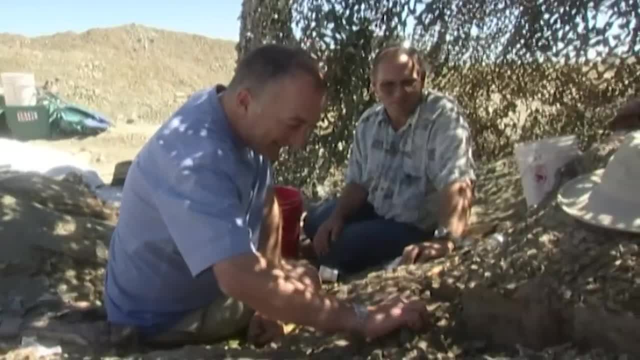 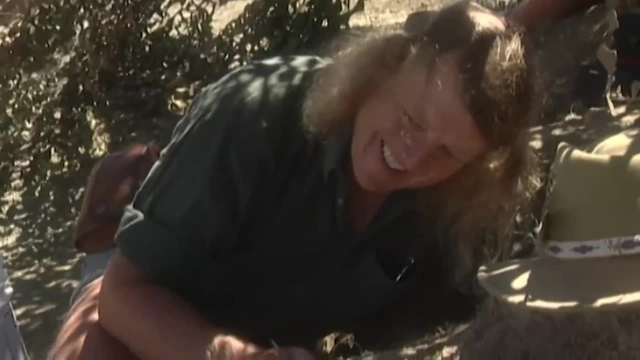 Even though I've had to leave my bounty in the ground, I can at least say I've helped to excavate a 75-million-year-old dinosaur. Don't it make you feel good? No, I can go back, happy Phil, I think we can both. 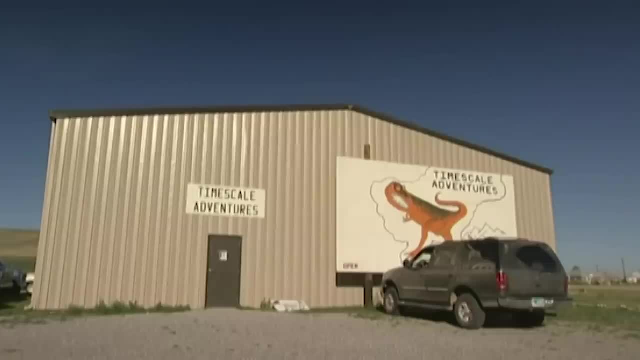 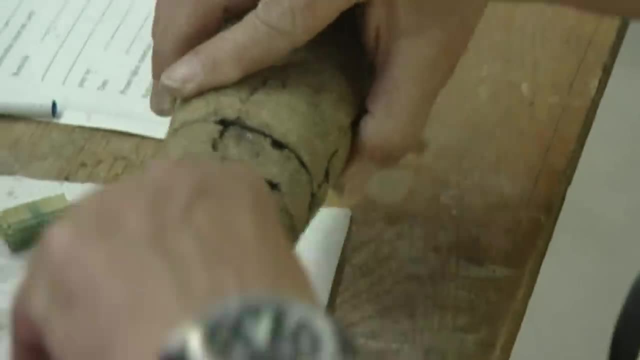 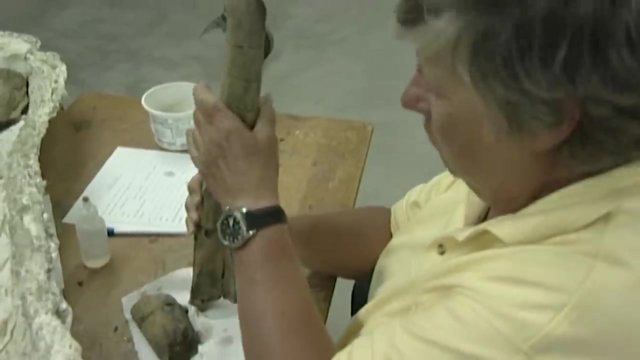 go back, happy Tony, But schemes like this are controversial. Most of the work, including some fairly technical stuff, in the labs is done by members of the public with little or no paleontological experience, And, although Timescale claims it's a non-profit-making organisation, 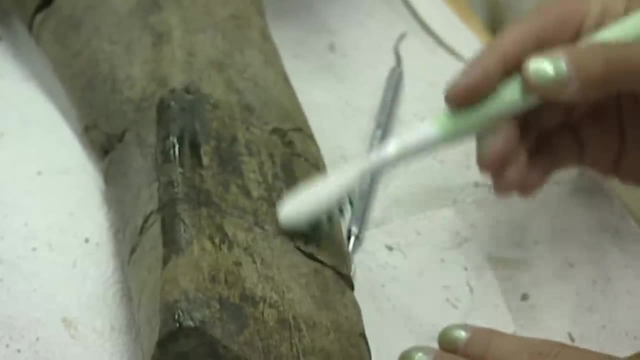 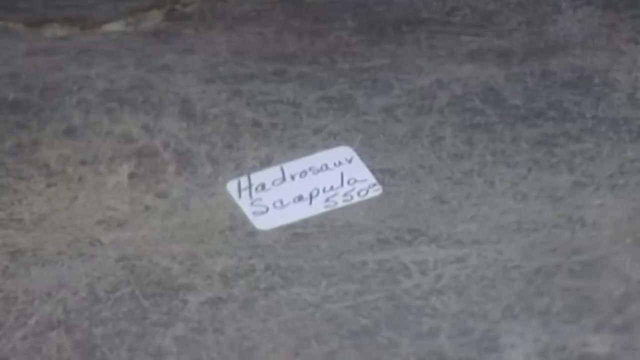 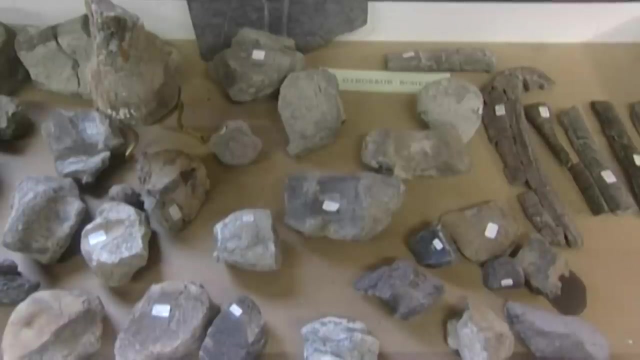 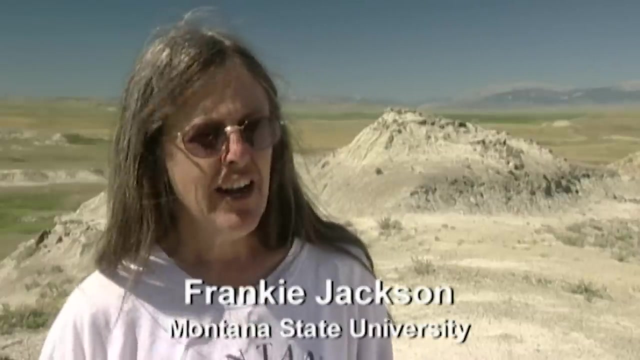 dedicated to research. its basic concept is uncomfortably similar to the black sheep of the paleo world: Commercial companies who dig up bones or indeed charge members of the public to dig up bones for sale on the open market. There are commercial outfits that do excavate and collect data. 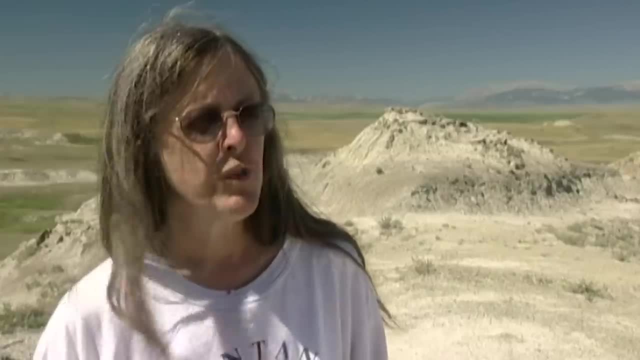 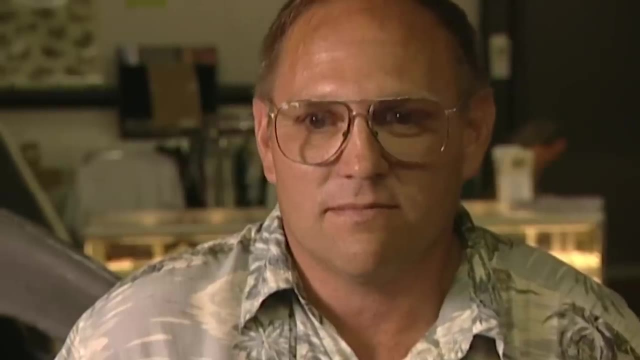 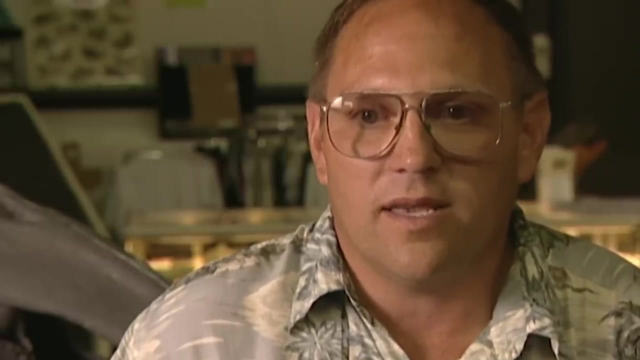 but a lot of them. the bones are just removed. We lose the data, we lose the research involved with these sites. What happens to the bones after your clients have dug them up? Actually, we keep them. They're permanently in our care. 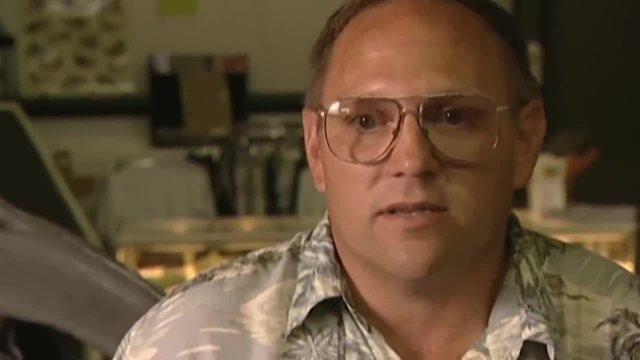 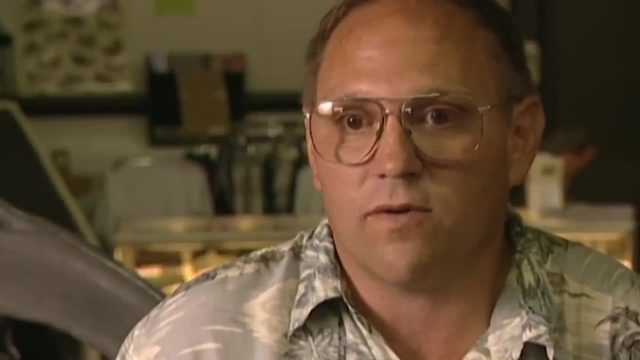 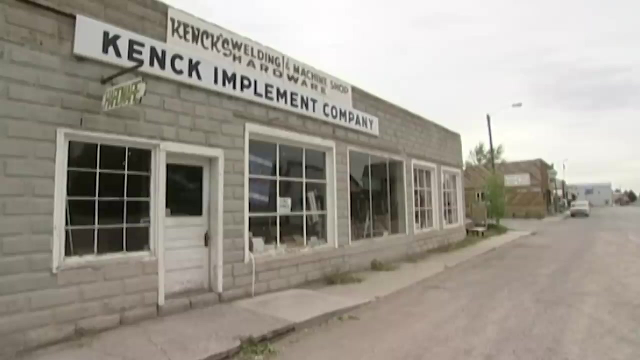 and they remain part of the public trust. We may not keep them physically on premises. A lot of times we will loan specimens to other institutions for research or display purposes. But yeah, they're always in the public trust, But not everyone. 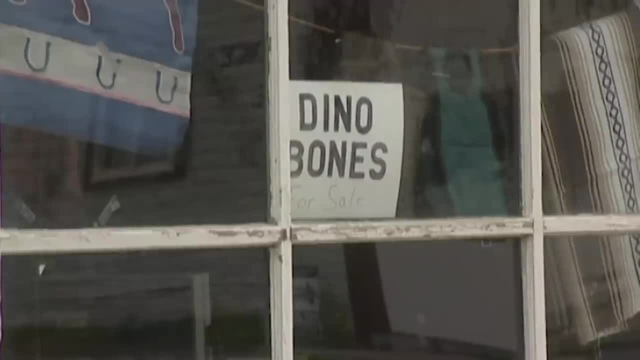 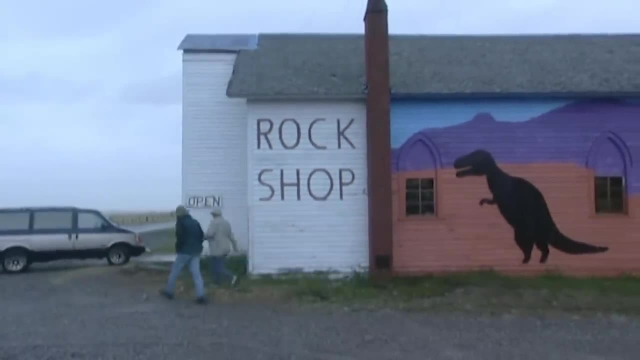 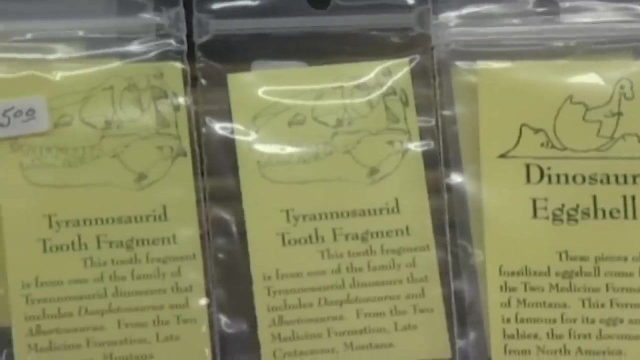 is as ethical as Dave. There are masses of bones for sale around here. The biggest local fossil retailer is The Rock Shop in Bynum, Which just happens to be run by Dave Trexler's mother. Where do you get all your bones from? 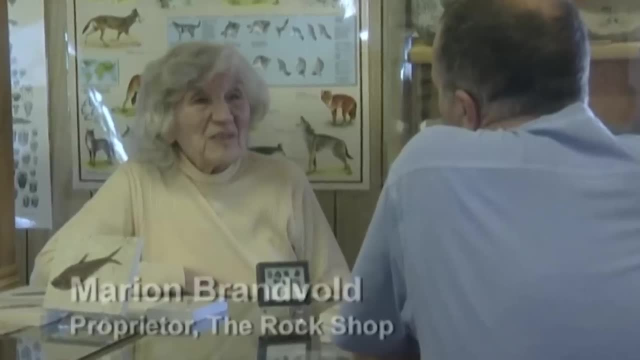 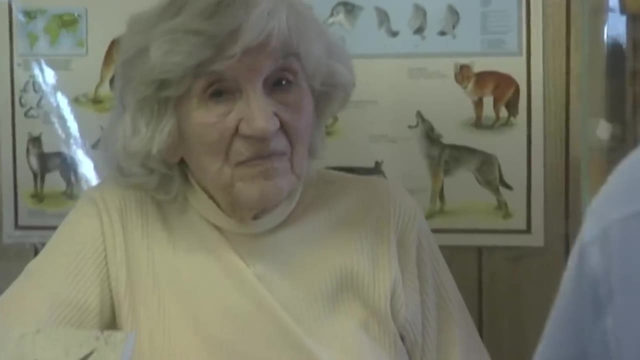 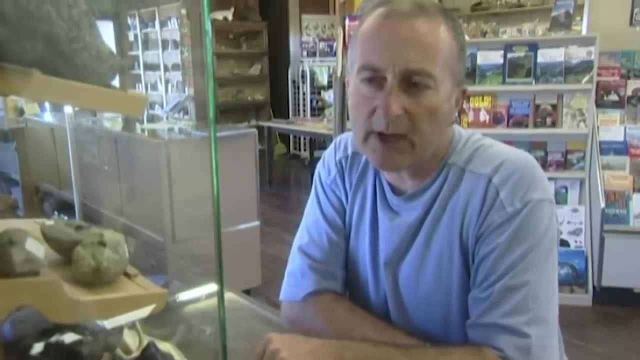 We buy them And you don't just advertise where you buy them. They're on private property And that's about all I say about them. Some people say that it's wrong to sell dinosaur bones. How do you feel about that? A lot of the paleontologists do. 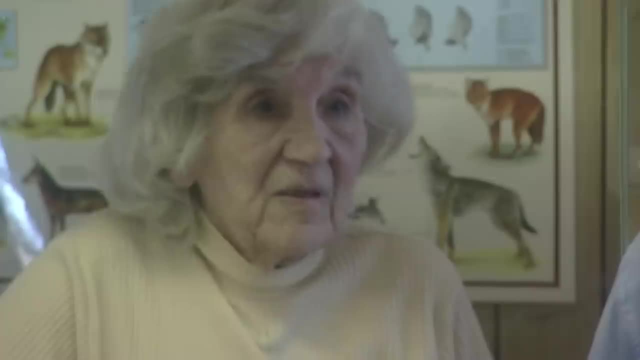 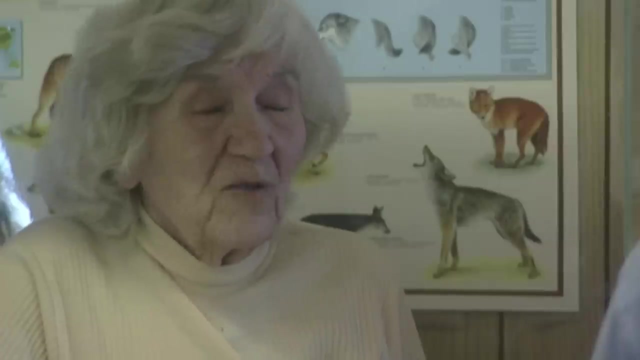 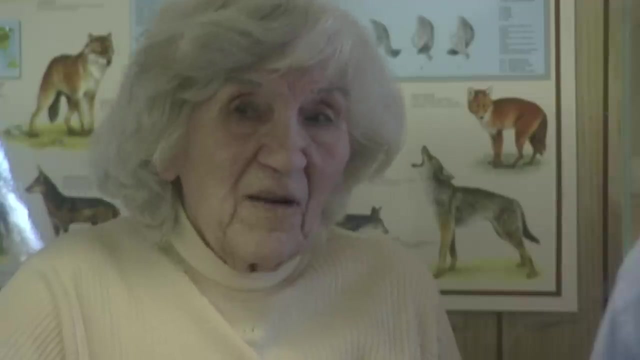 And my son, Dave, won't come in here and sell a bone. I would rather see them taken to school with some child to show and tell. Plus, why not have one on your mantel to look at, Or even on a card table? 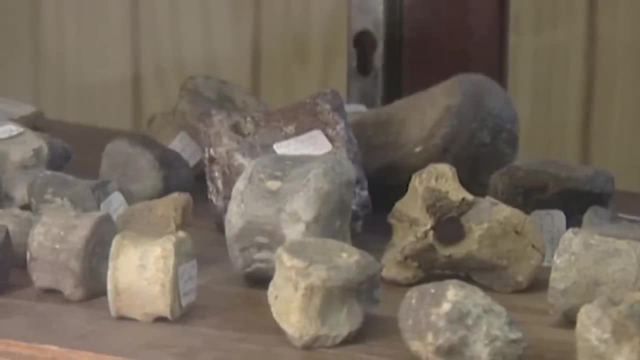 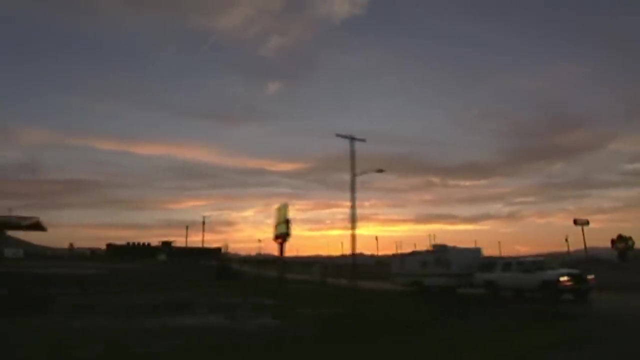 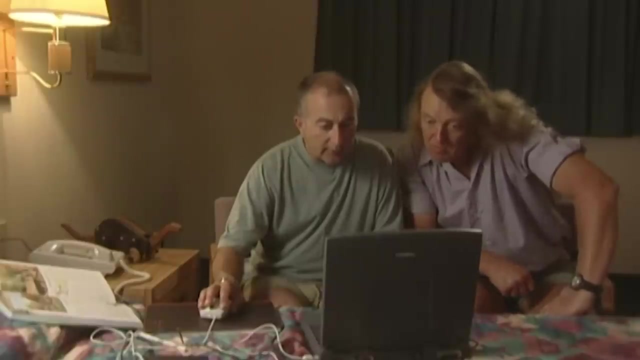 Even on a table Somewhere. Phil and I wondered if this was simply a local phenomenon or part of something much larger. So back at the hotel, we hit the net and discover bones galore. Here we are: Jurassic Age dinosaur bones for sale. 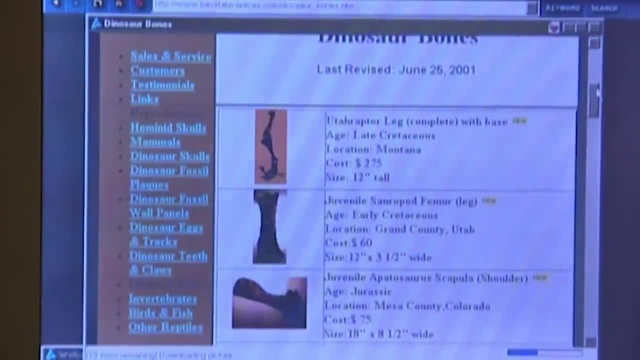 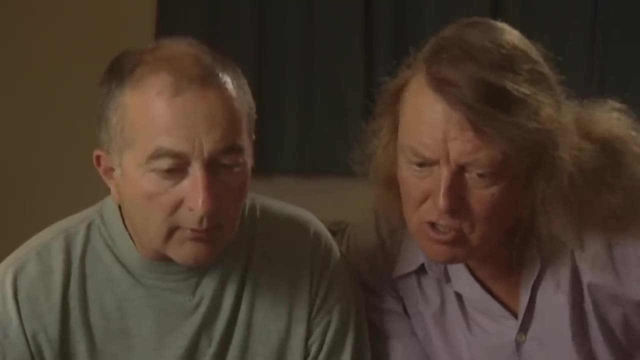 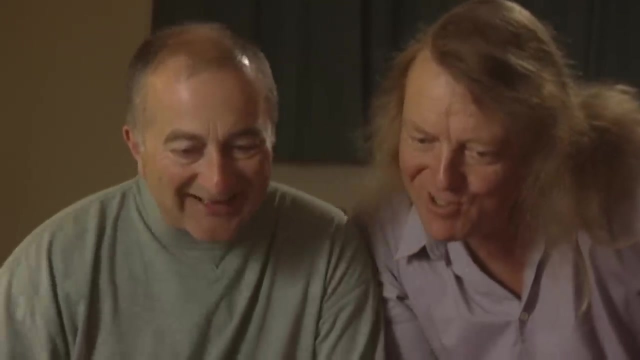 Let's have a look at it. Allosaurus metacarpal bone: Very nice rare bone, Only minimal reconstruction. 450 bucks- Oh, this is a real beauty. 900 bucks: Awesome texture and preservation of the small processes. 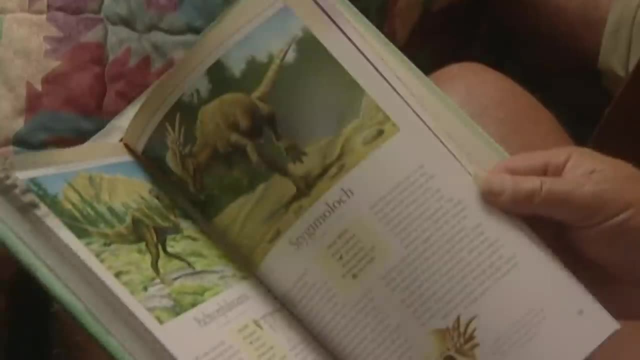 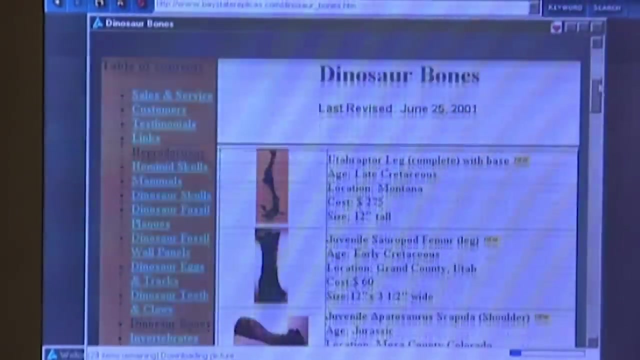 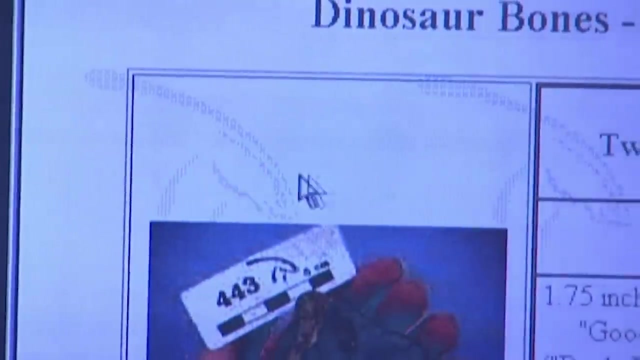 Camarasaurus, Have we got that? No one's been able to gauge accurately what the global dino bone market's worth, But a recent estimate by the Los Angeles Times puts it at more than $80 million a year And growing. It's very sick really, I think. 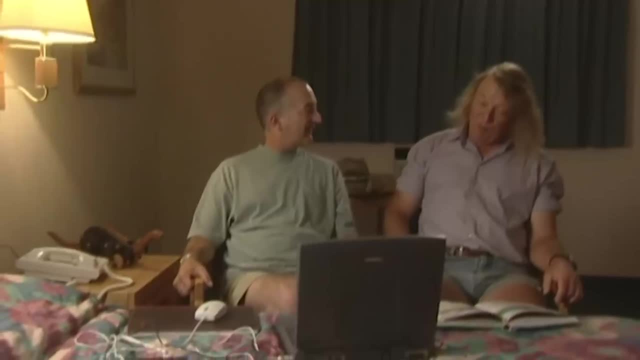 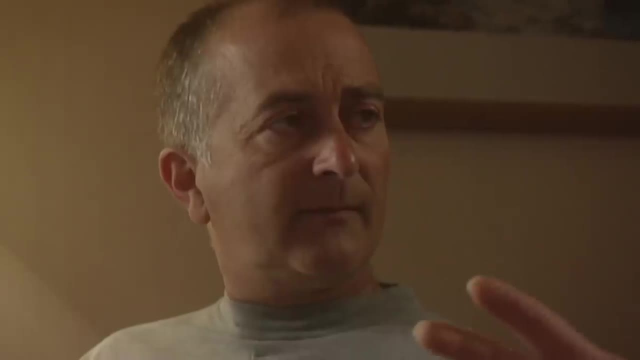 You know I mean. What do people want with one dinosaur bone At that price? the one thing that you really want- sorry to be boring- is context. You want to know where this stuff comes from. It's valueless other than that. 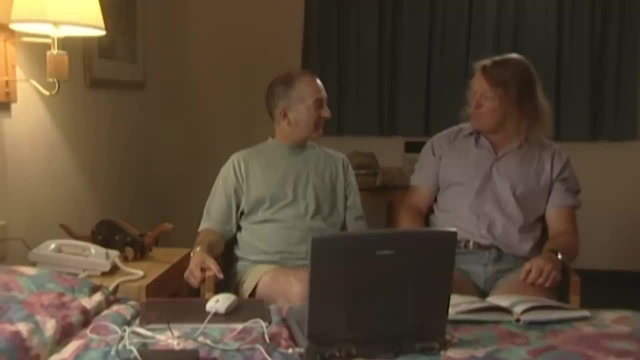 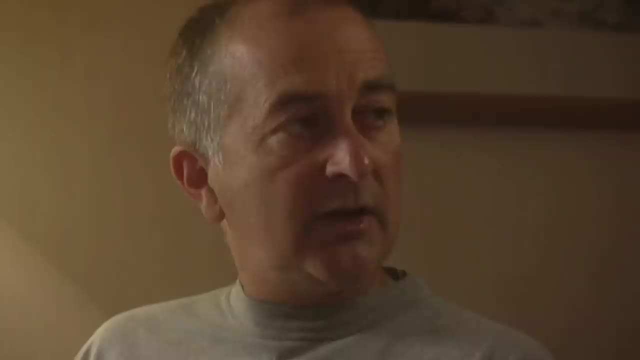 And there they are exchanging good money for stuff which is scientifically valueless but was probably very, very valuable when it was in the ground. But on the other hand, Phil, if you look through Montana and Utah and Argentina and China, there's a hell of a lot. 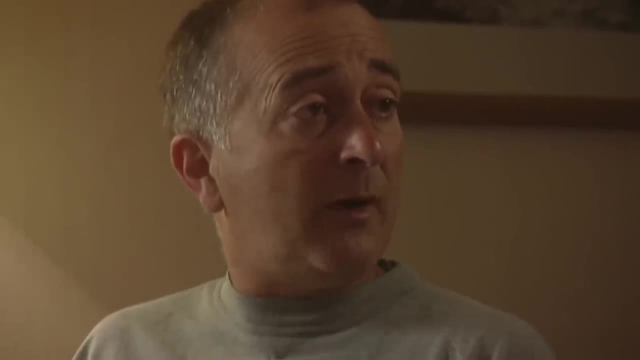 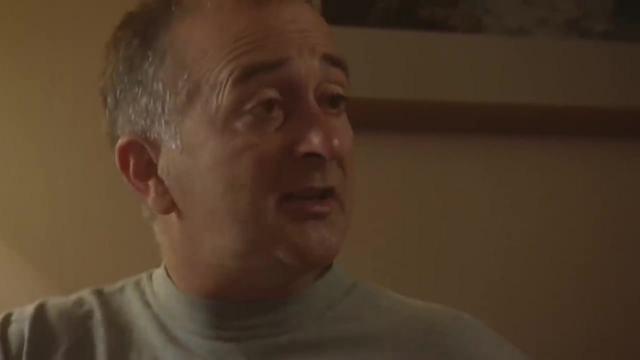 of mountain ranges that seem to be chock-a-block full of bones Where we were, we were walking on them like they were sherds of pottery from a massive Roman site in the Middle East. I mean there were that many of them. 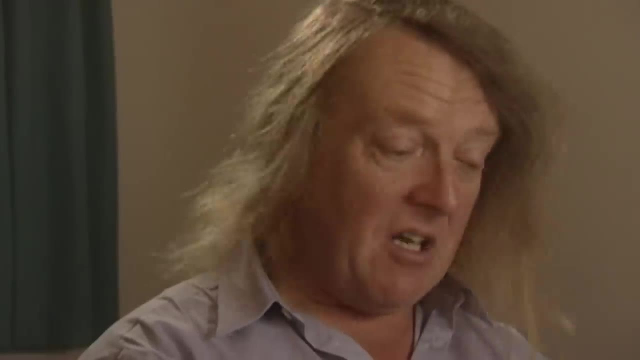 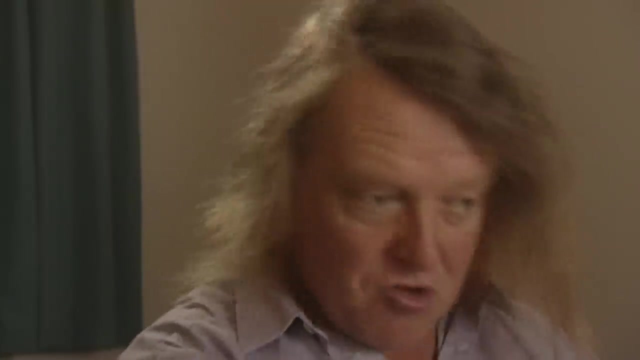 Yeah, yeah, Can we begrudge people who've got a little crush on dinosaurs just spending a few bob on a little bone like that? But a lot of that stuff is not unstratified, It's coming straight out of the ground. 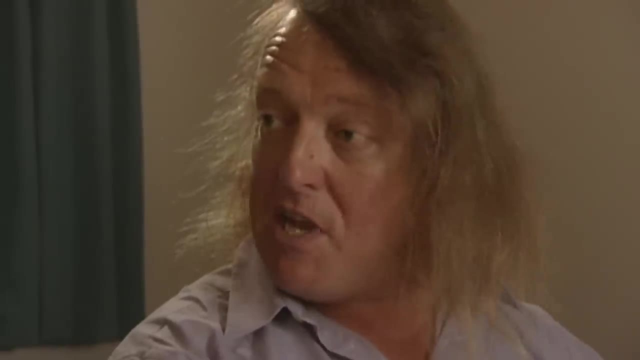 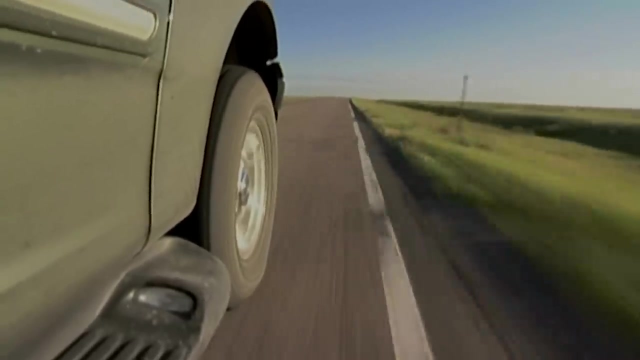 It's being dug out virtually as we speak, And I mean it's tantamount to just having a dig and flogging off the find. You don't do it. Luckily our schedule doesn't leave Phil too much time to wallow in his grief. 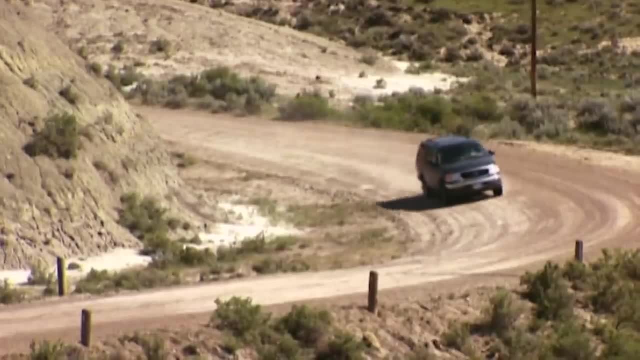 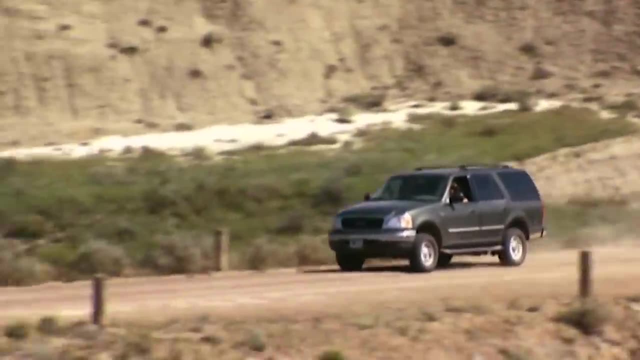 We've got an eight-hour drive to the eastern edge of the state to meet one of the most successful dinosaur hunters in the world, Jack Horner. He's currently digging in the alarmingly named Hell Creek. Apparently it's stuffed full of T rexes. 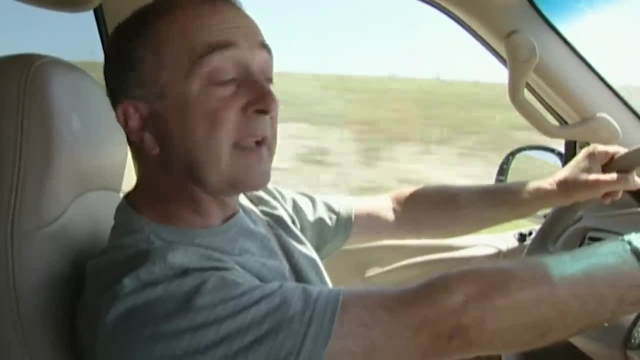 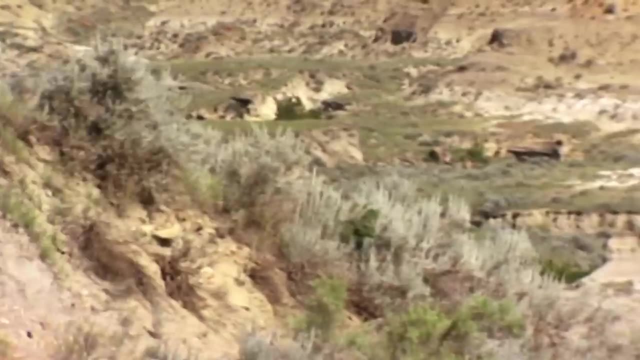 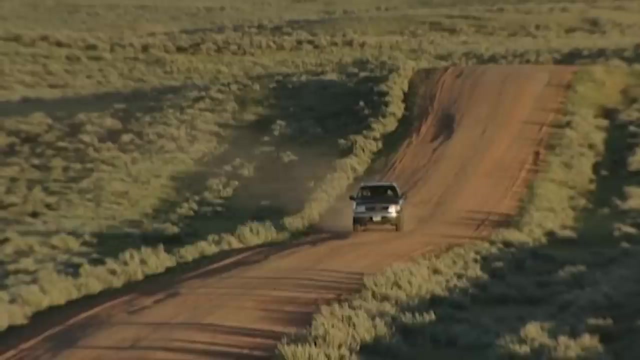 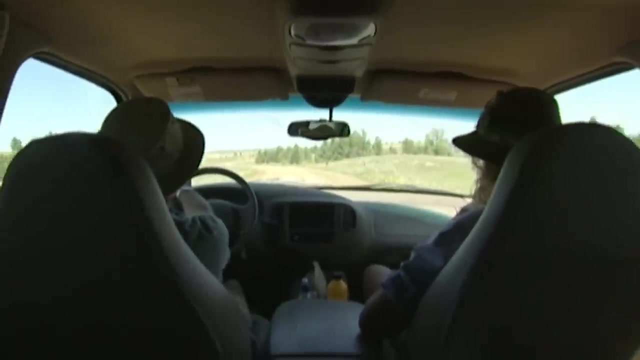 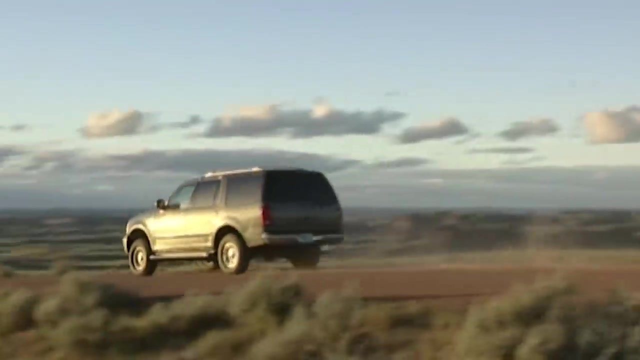 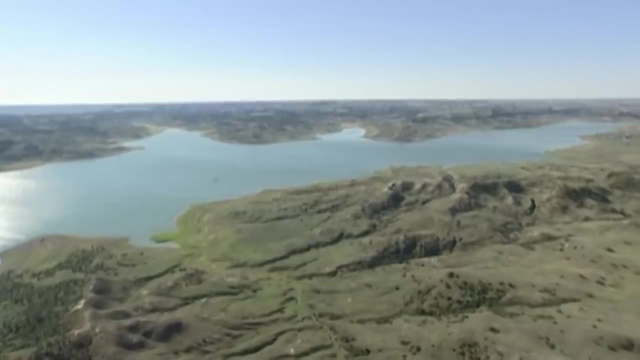 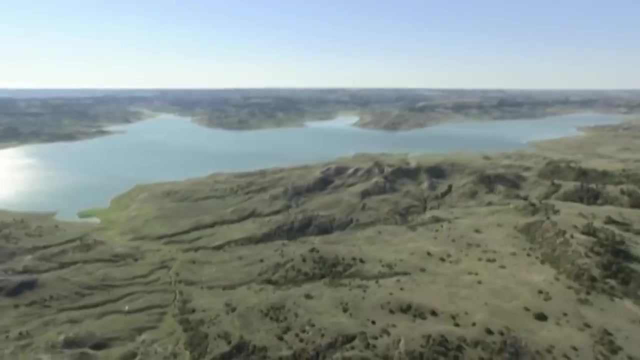 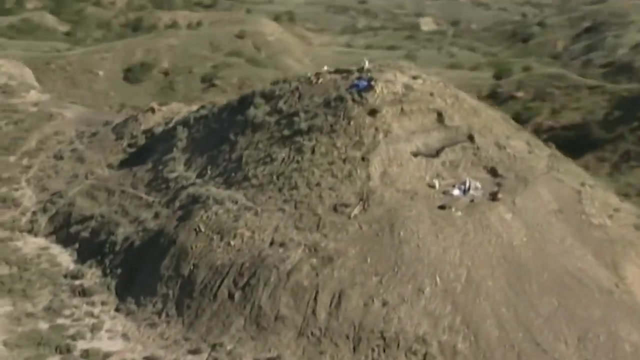 and we're going to see his latest discovery. Only problem is it's halfway up a cliff. Join us after the break. Hell Creek is home to one of the largest dinosaur excavations in the world, Hidden in these hills and gullies. 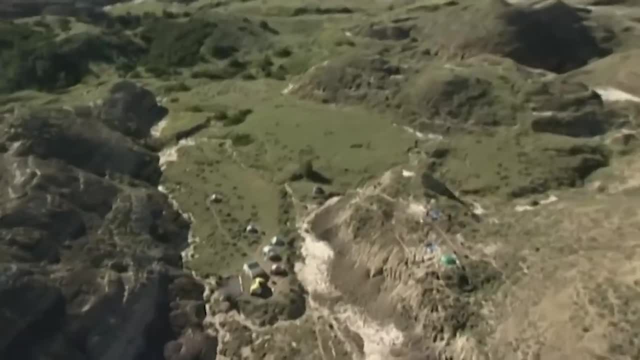 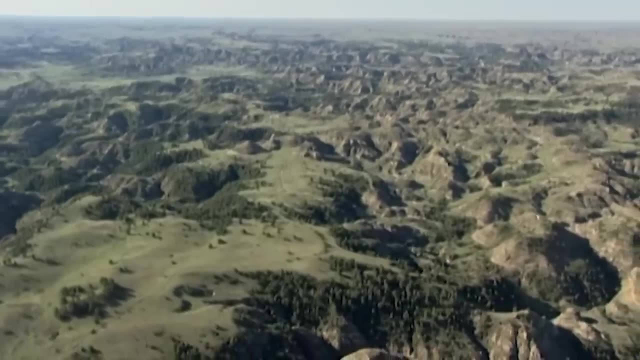 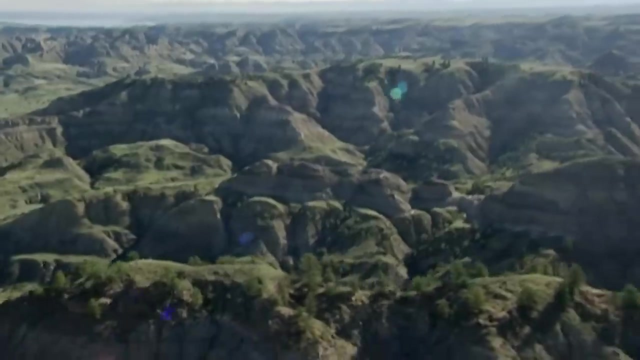 spread over at least 10 different sites is a team of 50 paleontologists all trying to piece together a picture of life here more than 65 million years ago. But you can't dig up a dinosaur until you've found it. So project boss Jack Horner. 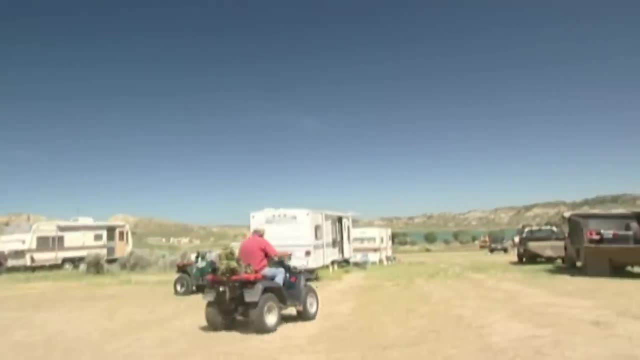 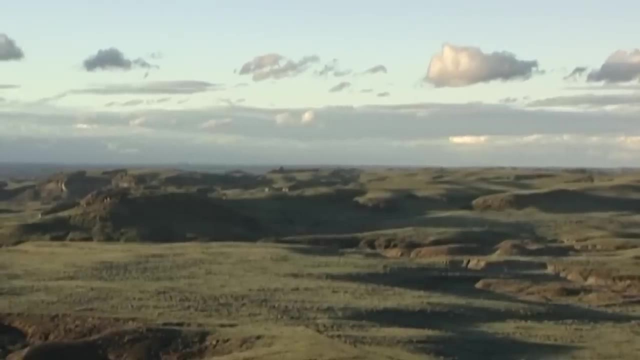 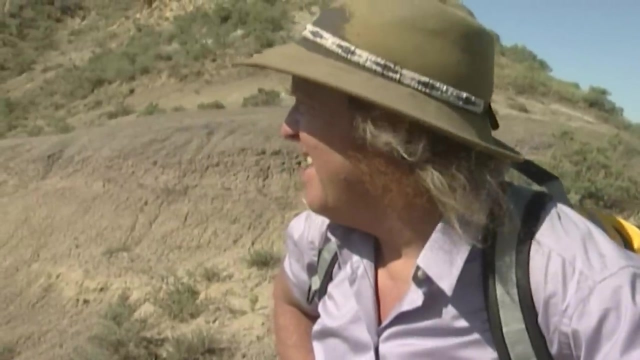 is going to give us a lesson in the most basic skill of dinosaur hunting: prospecting for bones. This, though, is rattlesnake territory and Phil's snake-phobic. Even though he's wearing top-of-the-range protection, he's very nervous. 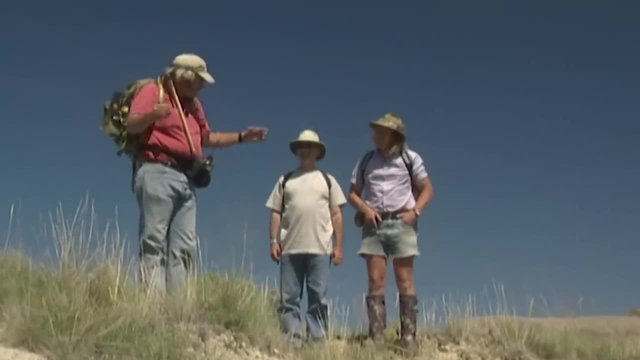 You don't have anything to worry about. Even if you see a snake, even if it bites you, you're fine, You're all right. It can't get you in the knees, It can't get that high- Unless, of course, 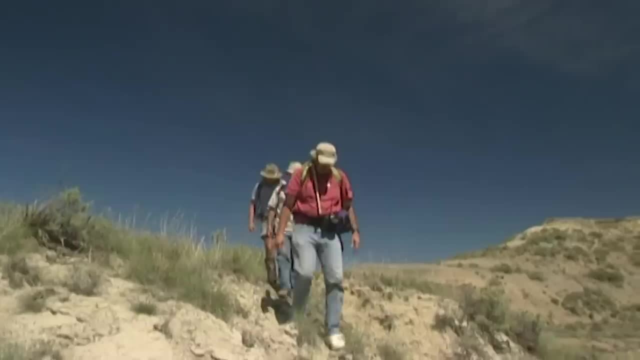 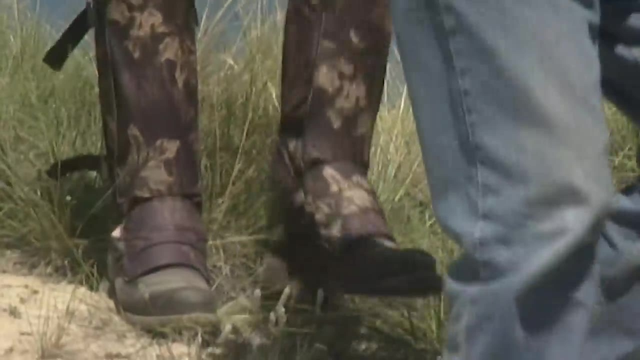 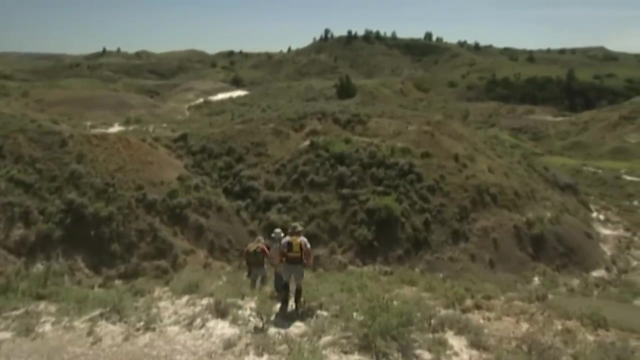 you're down in a valley and he's sitting on the hill. Not surprisingly, Phil decides the safest place is at the back And we're soon trekking in the midday heat into the shadeless Badlands. Is the terrain always this difficult? 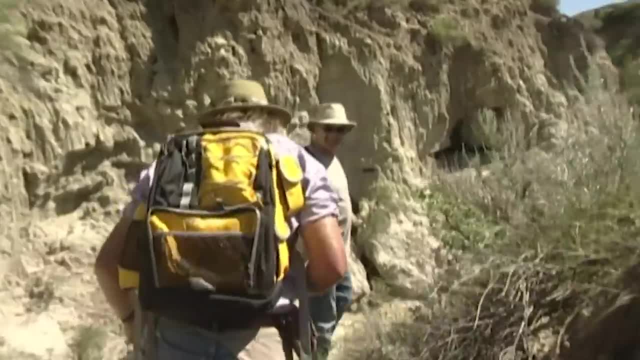 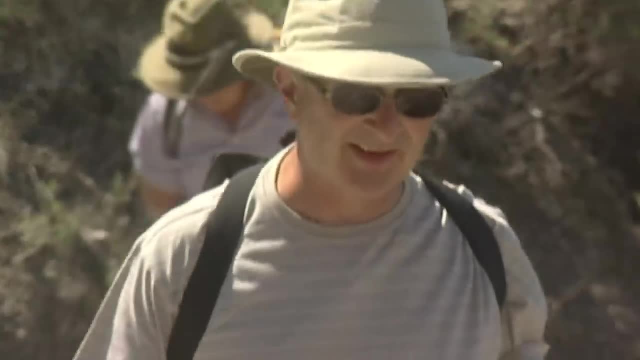 This is pretty simple. terrain here Simple. Most of our terrain's a lot more difficult than this. There's no great secret to prospecting. All you've got to do is walk for miles and look at the ground, Though, whether Phil's looking for bones or snakes, 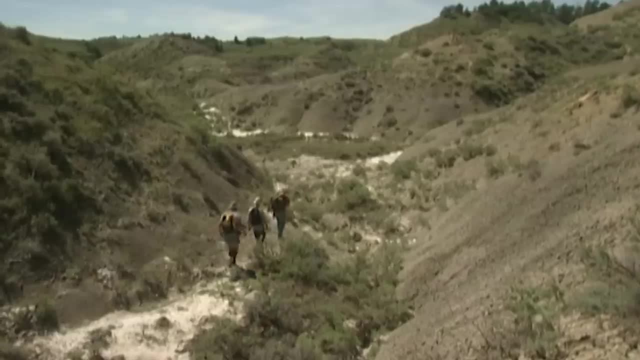 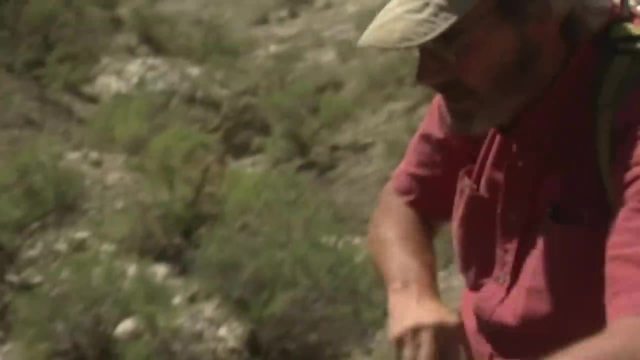 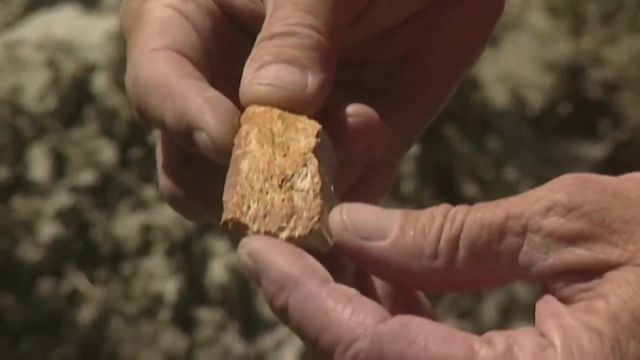 only he knows There's a piece of bone right there- Junk bone. Well, if you look at it, you'll see that it's. You can see the marrow. Yeah, So it's just a small fragment of a large bone. 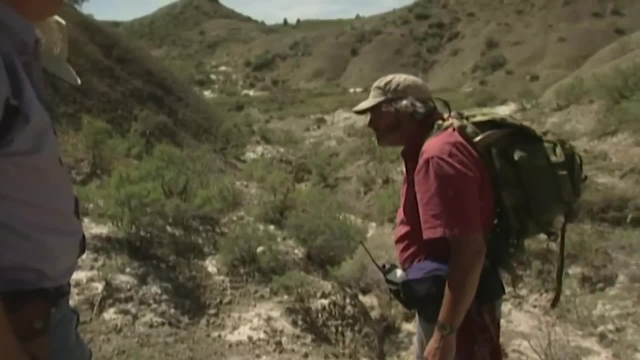 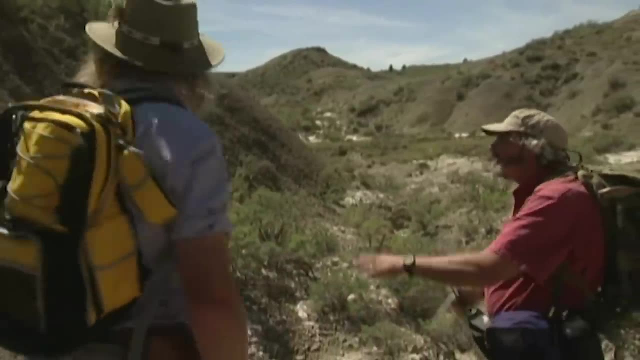 But that's what we're looking for: a piece of junk bone that we can follow up the hill So that bone is weathered down, is it? It's weathered down, probably on the slope here, somewhere It's come down and 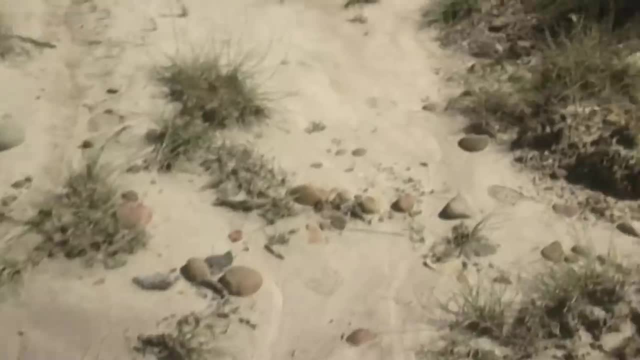 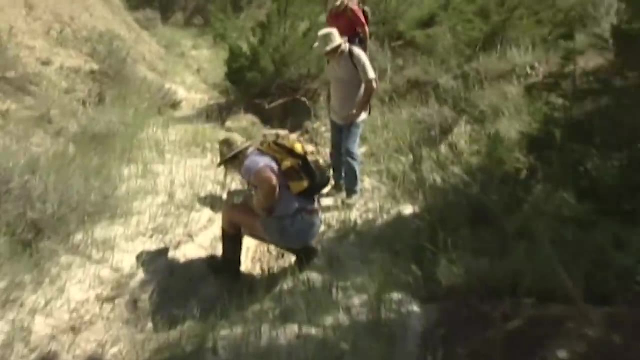 This is exactly like field walking, Tony, isn't it? I mean, it's just a matter of getting your eye in. It really is. It really is. Ah, There's an archaeologist looking for bones. Yep, that's a very nice. 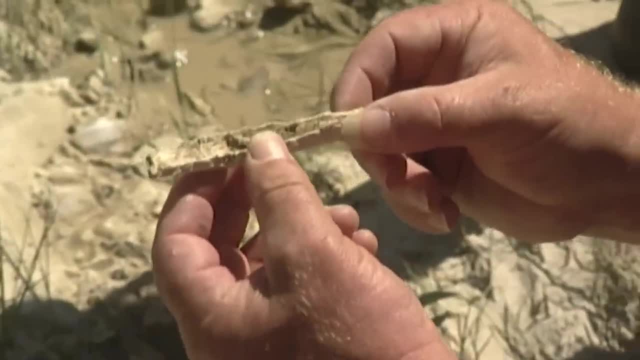 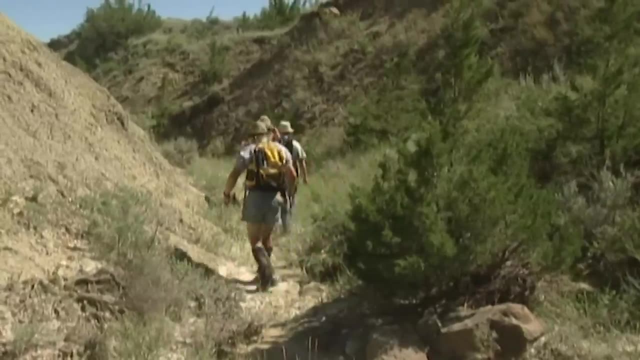 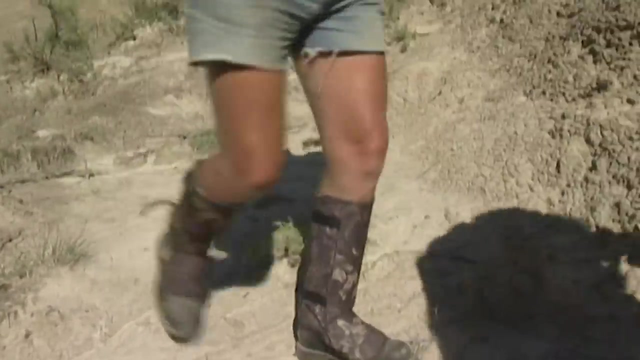 modern bone. For a paleontologist, a modern bone is anything less than several million years old. Phil's, no more than a few decades old, is brand spanking new. Still, I found me first bit of bone And it was the last bone we saw. 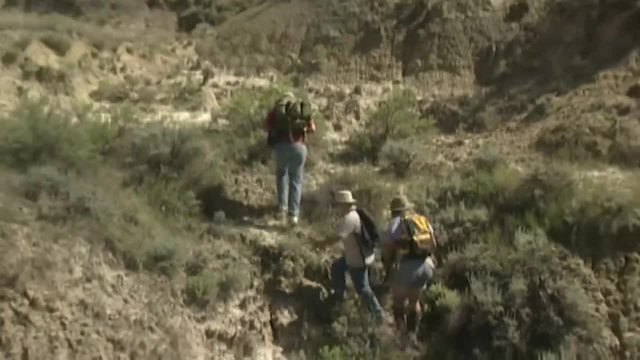 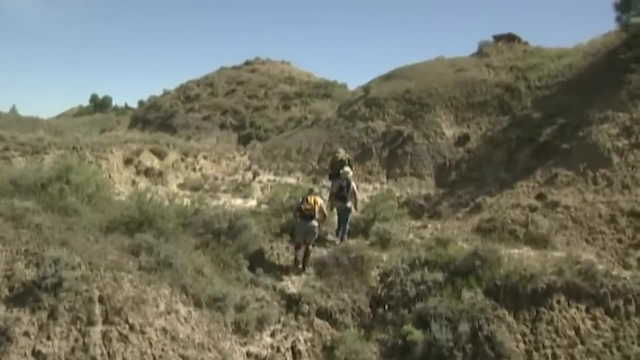 But although we were out of luck, sweaty grunt work like this has yielded an astonishing array of finds for Jack and his team. In the Hell Creek area, they've found the remains of more than 60 dinosaurs, including 50 triceratops. 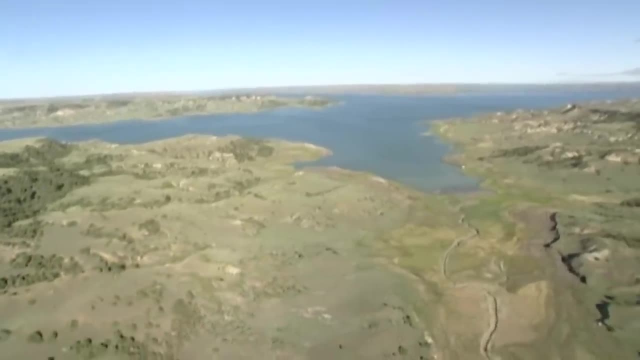 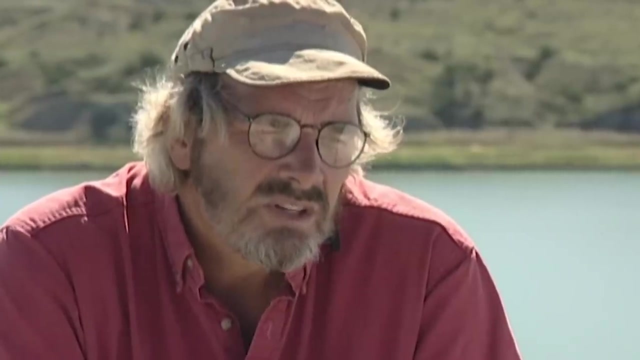 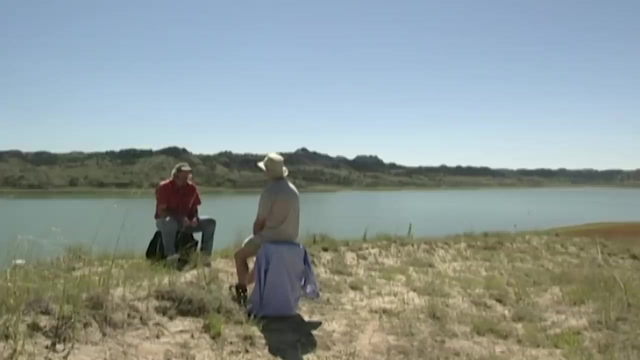 three hadrosaurs and seven T rexes. You say you've discovered seven T rexes. How many are there in the world so far? Oh, about 22.. So we've got a good third of them. Most of our information. 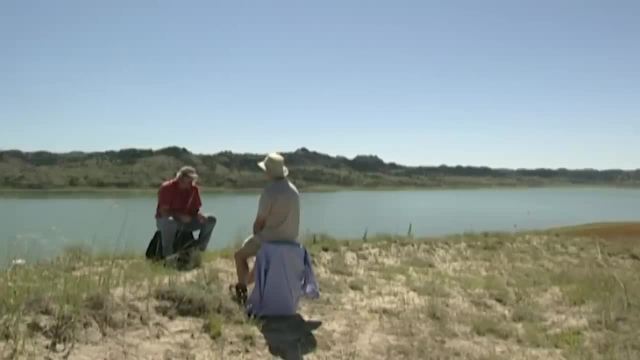 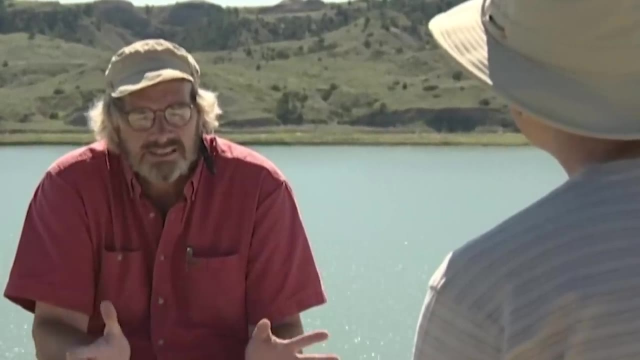 about T rexes come from here. Most of our information about triceratops, Most of our information about the K-T boundary- the last of the dinosaurs and what happened to them- comes from this area. So this for dinosaurs. 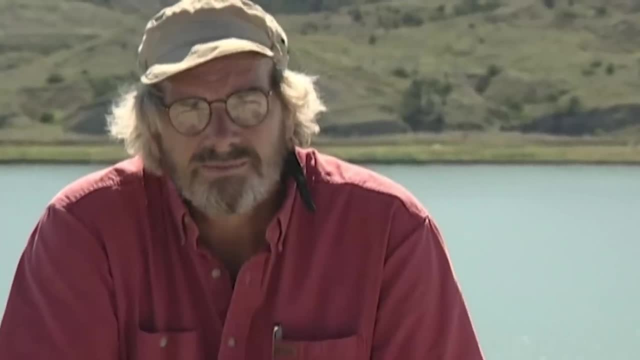 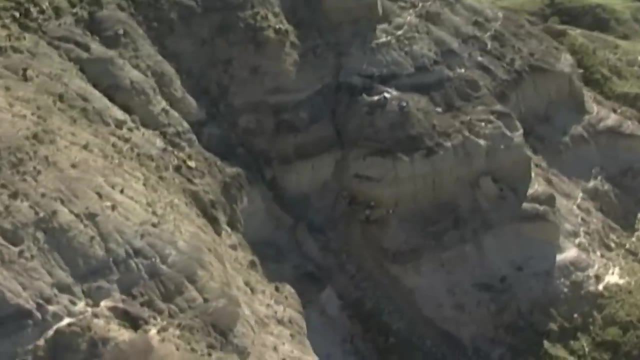 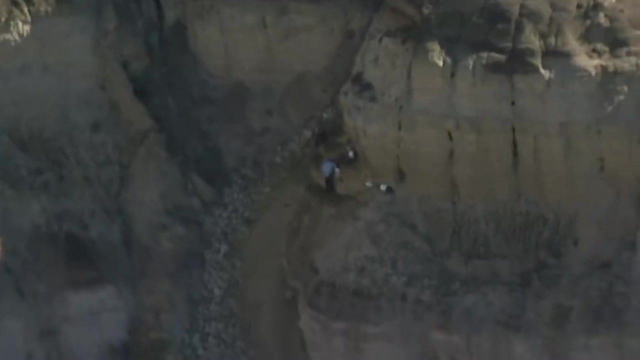 this is an extremely important area. The problem is, most of the sites are in very awkward terrain, and none more so than this. The latest discovery: Several miles from base camp, these distant figures are excavating an adult Tyrannosaurus rex. 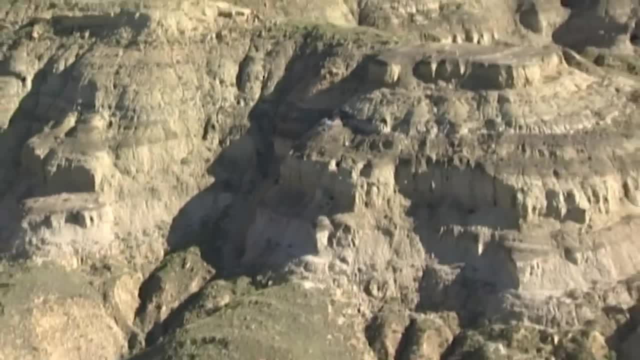 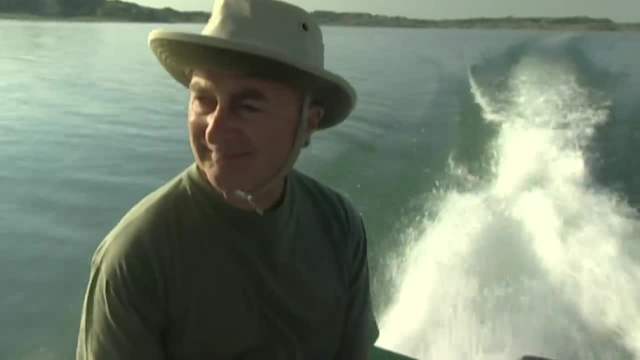 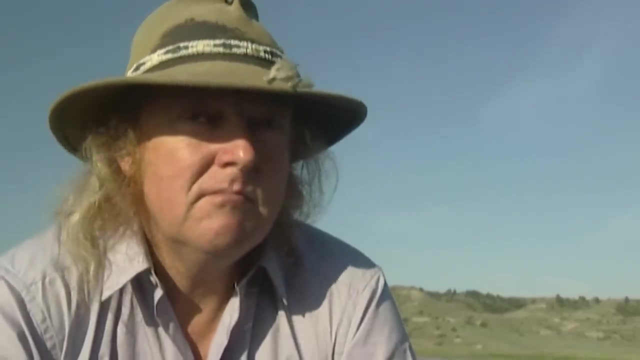 just what we hope to see, And it's where we're going next. It promises to be quite a trip. The sites are all known by the initial of the person who discovered them. B rex, as it's called, was discovered by our guide. 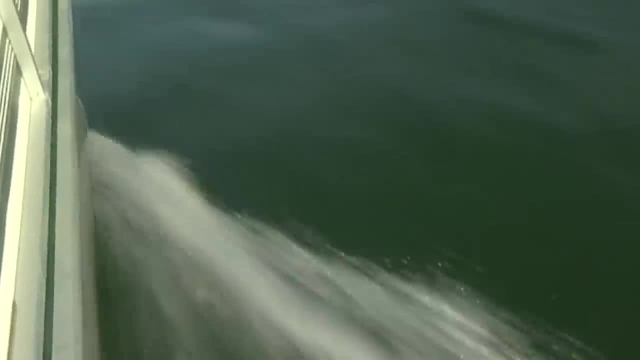 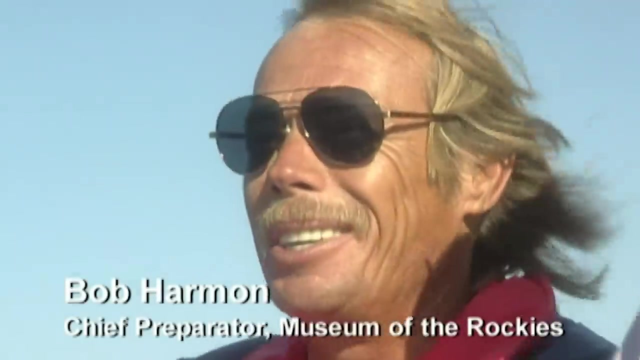 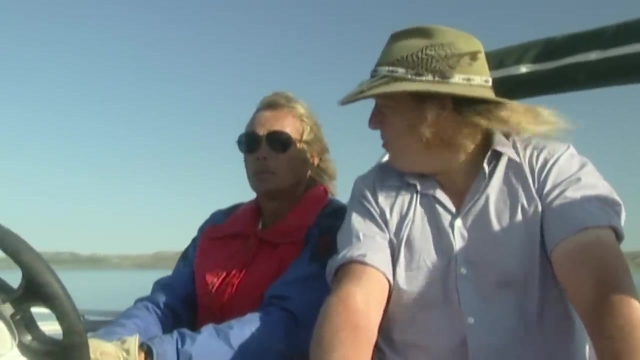 the other day, Bob Harmon. What is it specifically about dinosaurs that really gets you excited? Yeah, I don't know. They're cool. They're cool. You found- actually found- this site, didn't you? Yeah, How'd you find it? 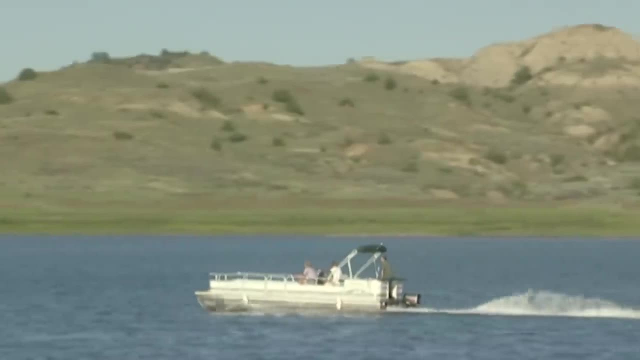 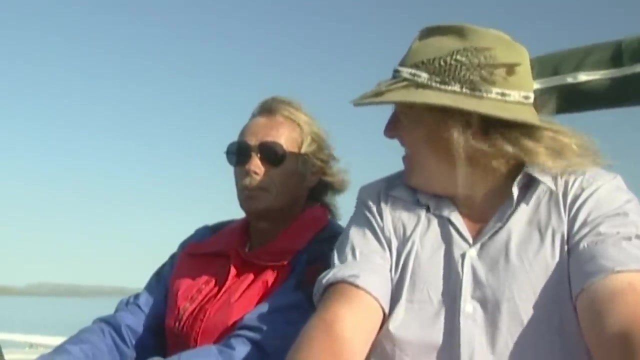 Not looking for dinosaurs. Yeah, Not looking for dinosaurs- Not to have lunch. How do you feel about it? you know, when you got your first T rex- Oh, it was exciting. Was there anybody there to share the moment with you? 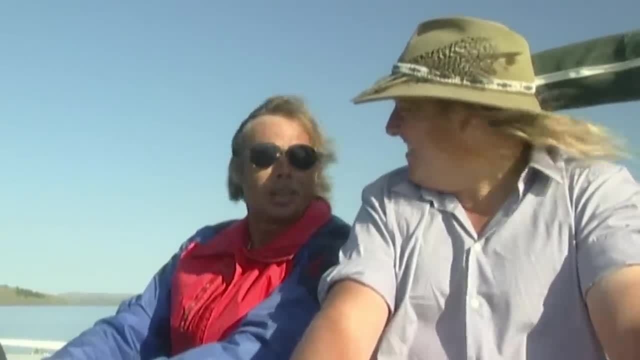 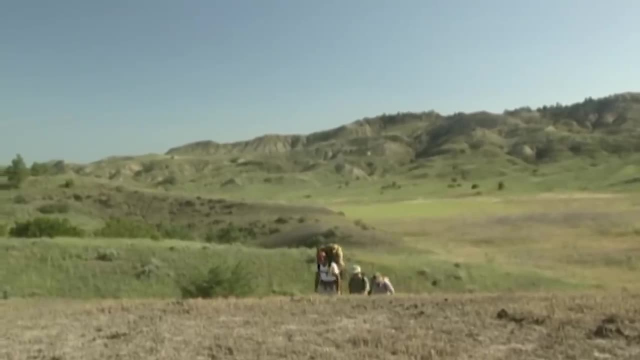 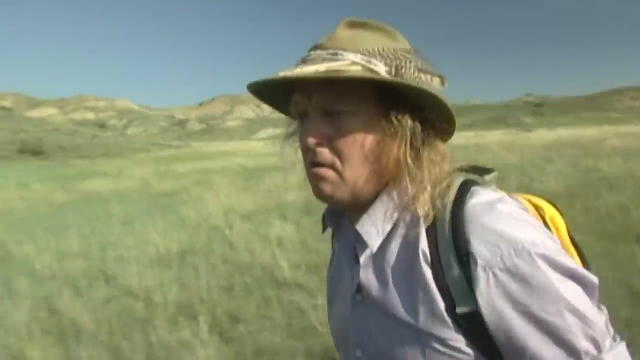 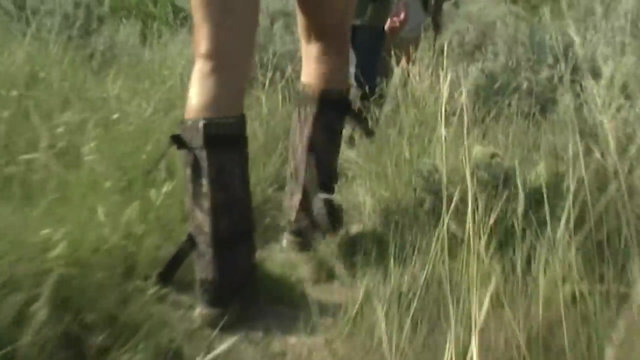 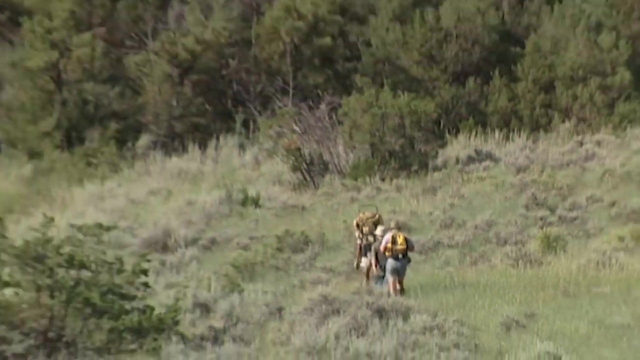 No, Just yourself Being a dinosaur. it is. The boat was the easy bit. Now we've got an hour-long hike And with the temperature climbing into the high 90s it's very hard going. It's easy to see why the people 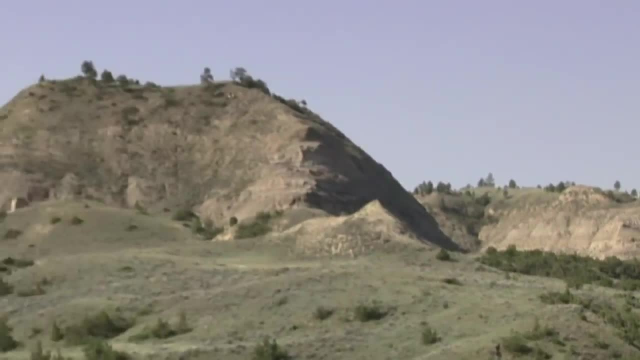 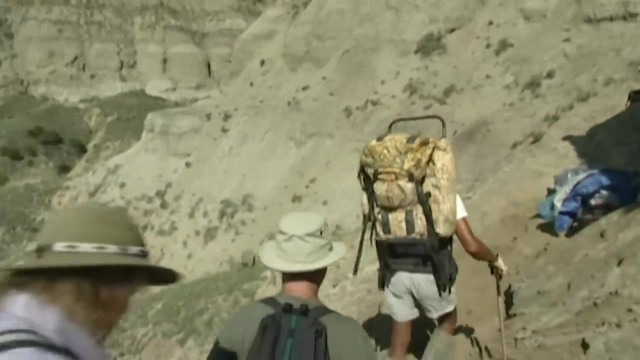 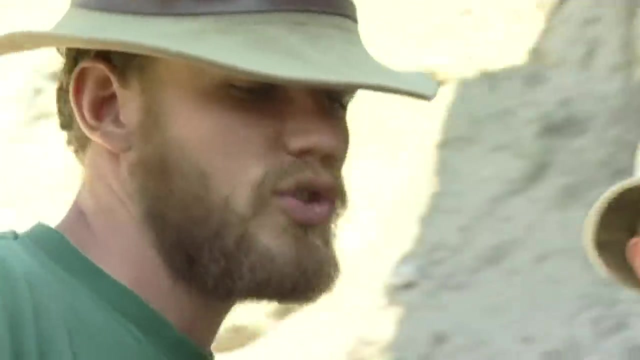 who work at B rex camp on site Looks like we're here. What have you got here? We've got ourselves a T rex. Oh, This right here, what you're seeing is a centrum or a piece of a vert. 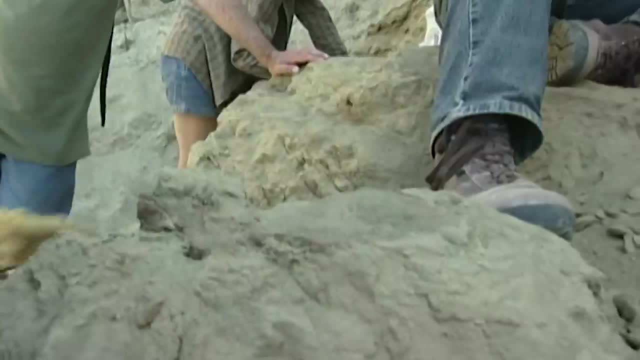 You can see the processes coming off this way. That thing had a spine some size there. It did, didn't it? Yeah, it did, And we're not sure exactly where this came from. so there could be many more verts that are bigger than this. 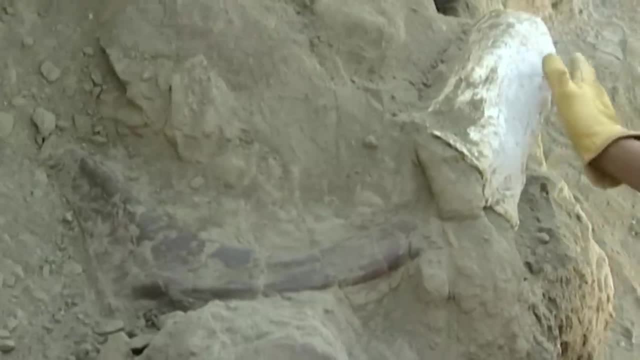 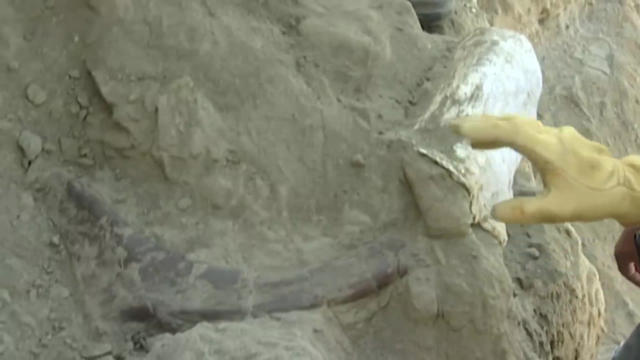 or smaller than this, And this right here, this rib. now, this rib was actually hanging out of the side of the cliff in this direction, right here. So really, that was one of the first things we went after: was that rib, to find out. 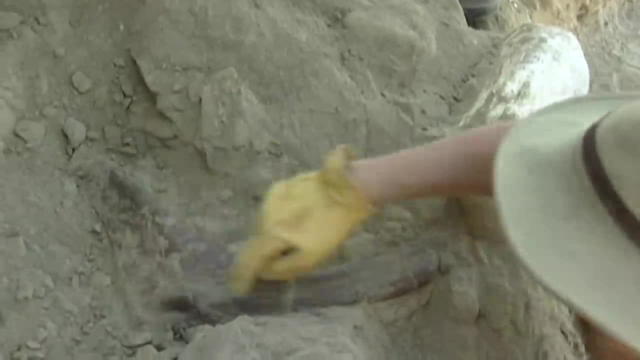 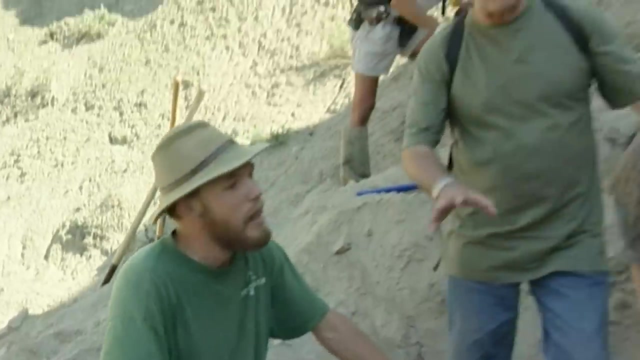 If it had moved or something, we would have lost this head right here. But as you can see, this head is in beautiful condition. No chunks out of it, no really terrible wear into the bone. Can you show me how much you've taken away? 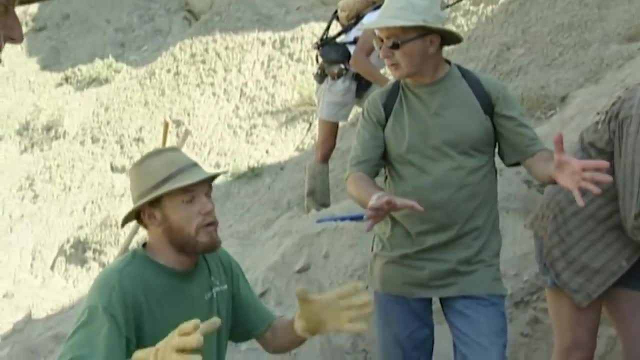 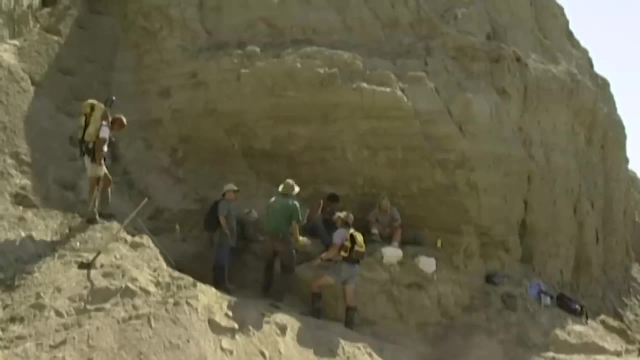 Since you started. I mean overburden or rock on top. Yeah Well, this wall here actually came out away from it and it went up 30 feet in the air, which is the fact it was overhanging a bit. 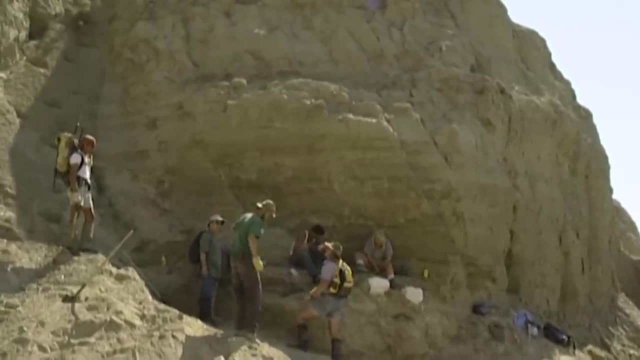 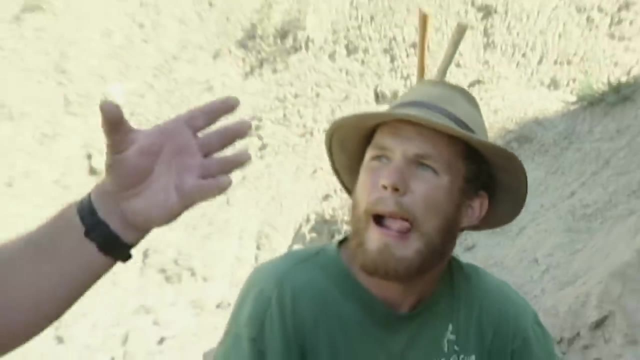 All this rock, All this rock. If you, just if you stand way back here, you can see the top layer of mudstone up there and that came straight out and straight down, But I mean just on the basis of two or three bones. 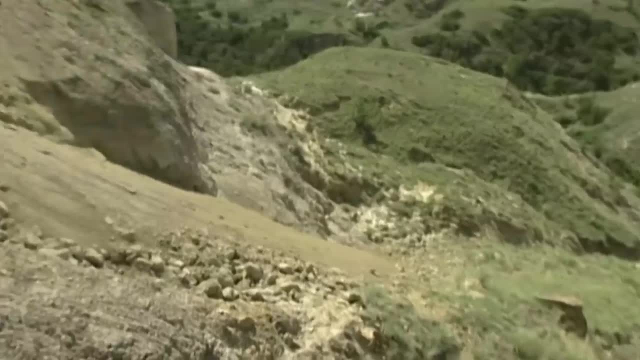 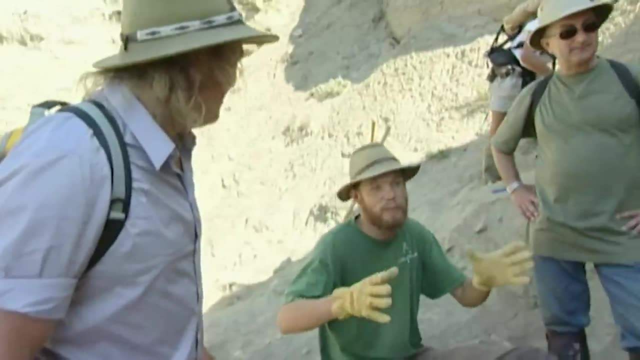 sticking out of a cliff. how do you actually decide we're going to go for this one? We're actually going to put all this effort into having a dig here. That's a good question. I mean, you come here and there's this huge pile. 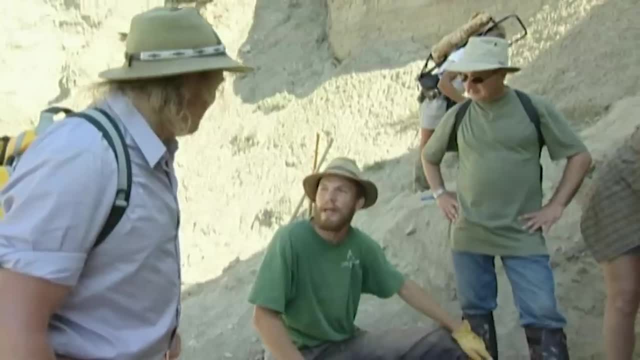 of heavy rocks on the top of these bones and you don't know, It's a big guess. I mean you have to be sure that there's something in there. But the crucial thing it said that it was worth coming in was the preservation of bone. 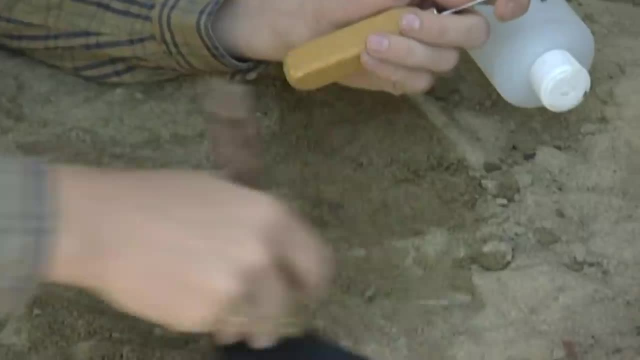 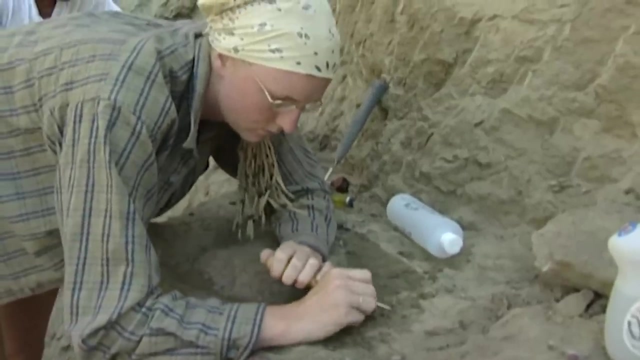 We've never seen T rex bone this well preserved, As well as the rib and vertebra. several other bits of B rex are beginning to emerge from the rock, And Phil's got his eyes on the biggest one. So what I'm going to have you do. 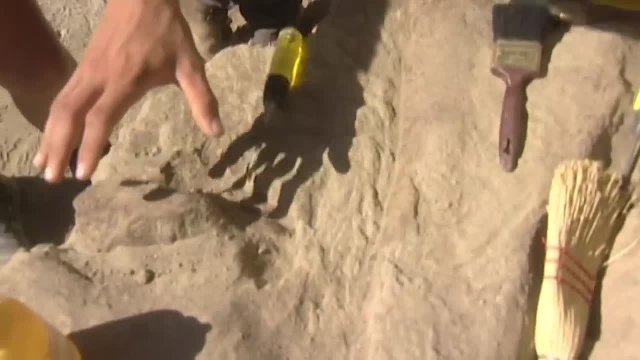 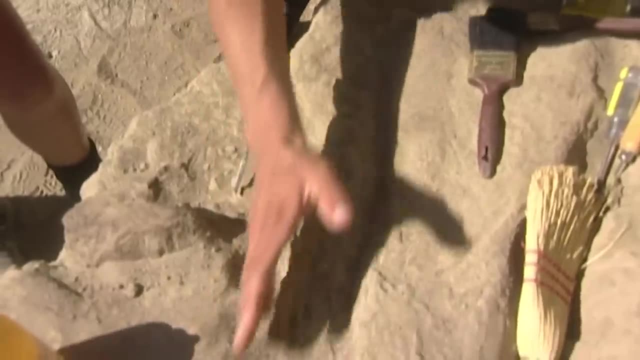 is, we need to separate this bone from this bone so we can put them in two different jackets Right Now, assuming they're different bones, Right. We always go into the assertion that they might not be, so you have to be really careful. So we need to trench through here. 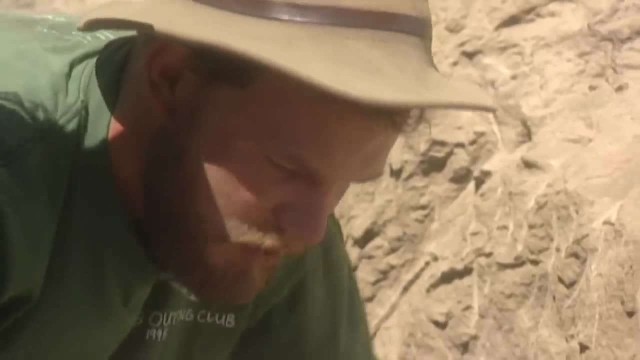 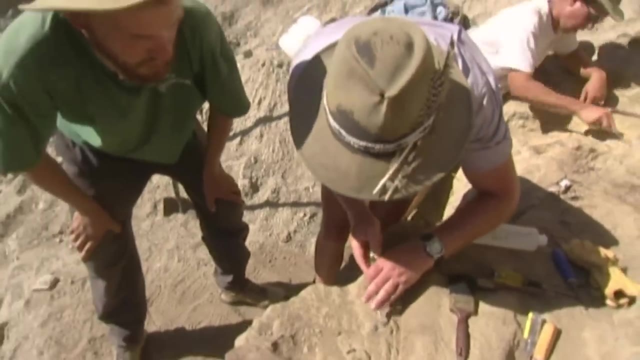 just like this, Right, And you want to stay about an inch away from each one of these bones, Right, It's so impossible. If I start in there, God it's. you know, that was amazing, because I just eased against it. 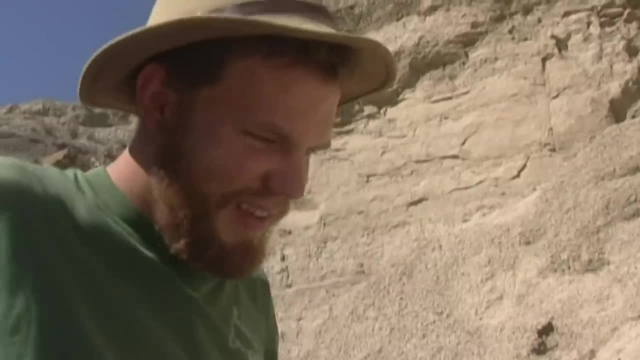 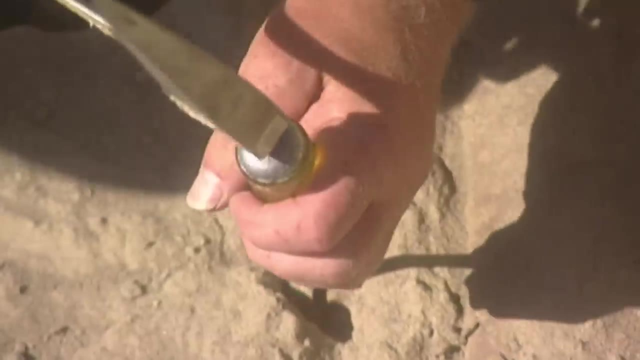 It's immediately softer than I thought it would. It's Under Nels's watchful eye. Phil's going to try Phil's soon, quarrying like an old pro. Now this is something that I don't normally get to do on a 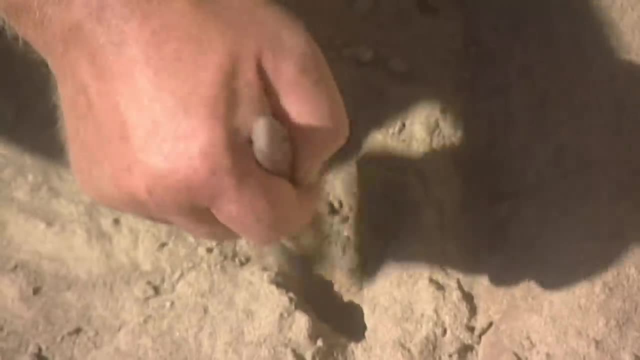 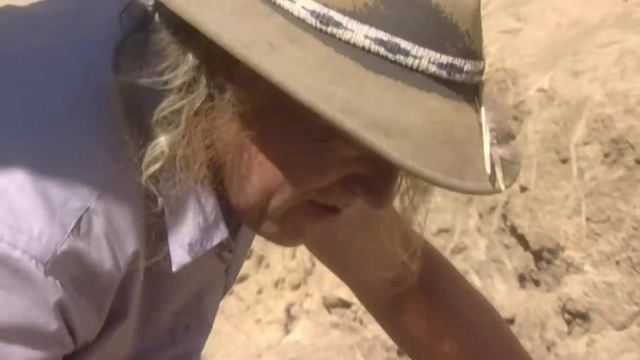 on a dig, Use a hammer and chisel. I'll have to remember that next time I'm digging up a dead Saxon or something like that. You were a bit scathing about archaeologists when I when I turned up on site. 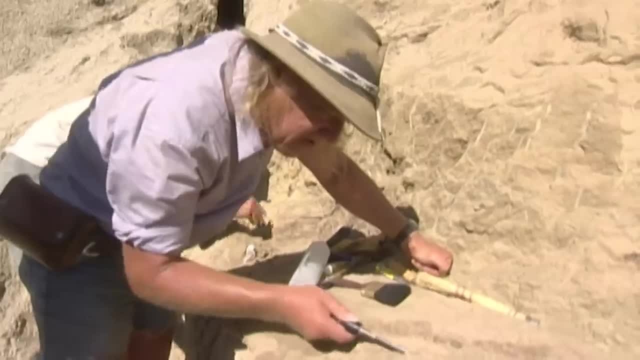 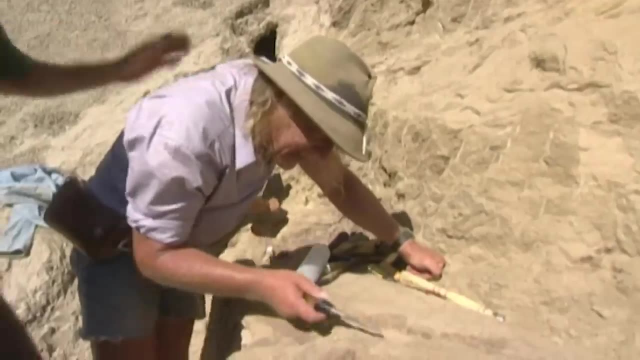 Oh no, You said. you said there's no room for archaeologists here. you said I have to. you know, in all in all, in truth, we're all diggers. Yeah, but you have to admit, dinosaurs are cooler than. 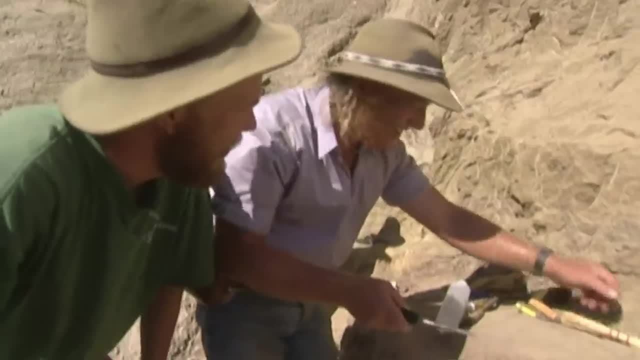 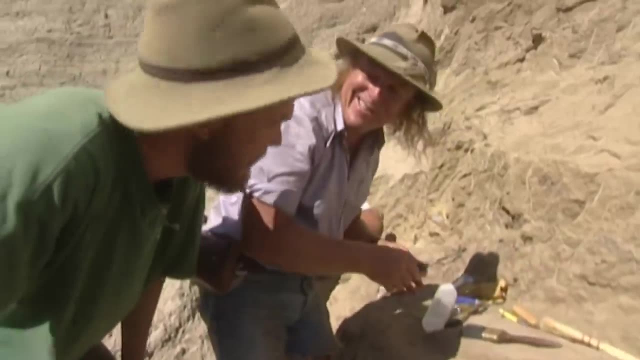 than than anything else there is to dig up in the world. Cooler, Cooler, Is that right? Yeah, more awesome. Well, they're certainly more awesome with the temperature in the 90s. I don't know whether cool is quite the right word. 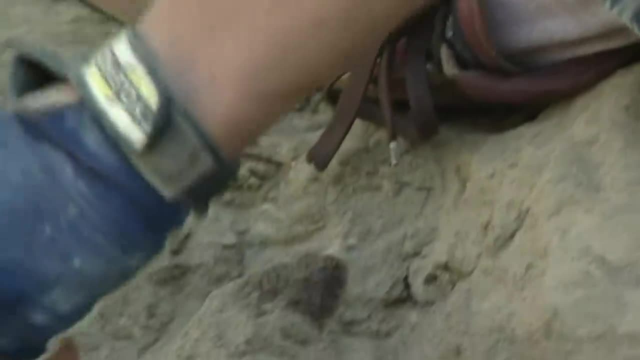 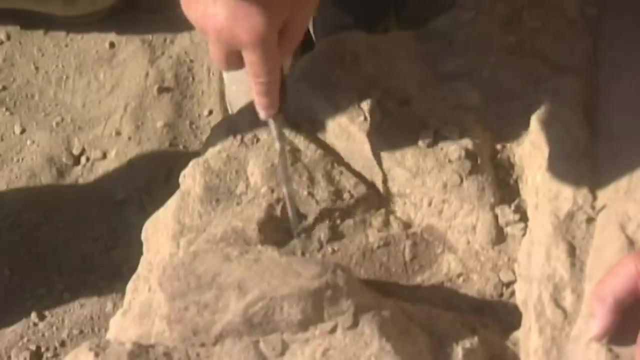 It's going to take at least another year to recover the whole animal, Though Phil's really keen to get his bone out of the ground before the end of the day. But the more he scrapes, the bigger it gets- Nails Yeah. 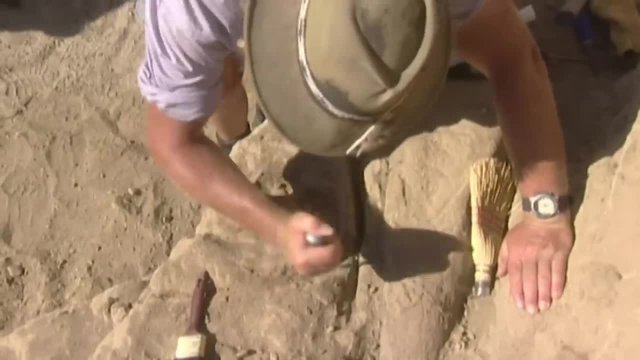 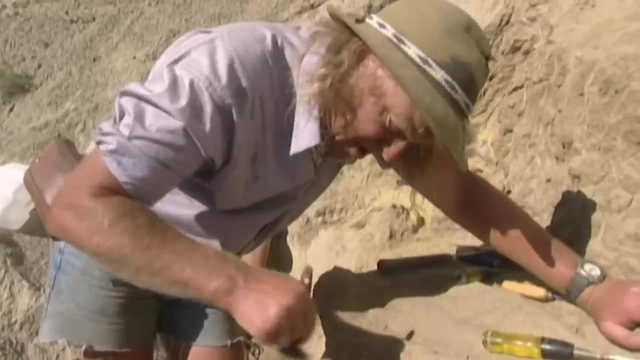 Have you got them in there? I do. I'm beginning to beginning to run, beginning to run away with me. Oh Look, we have this big lump of bone on there to start with, which is why we've got this big lump. 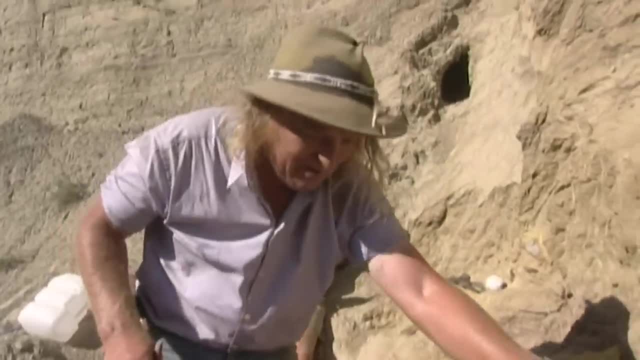 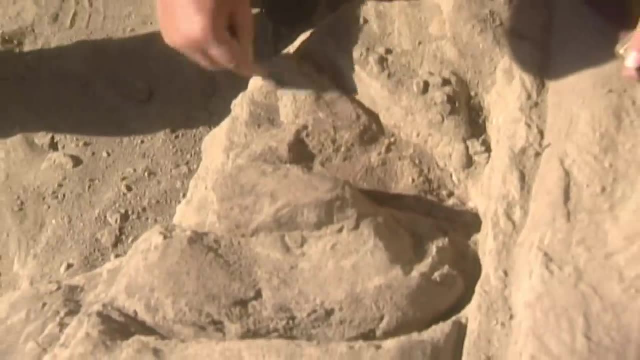 of bone on there to start with, which is why we've got this big lump of bone on there to start with, which is why we've got this big lump of bone on there to start with, which is where I was trying to trench all the way round. 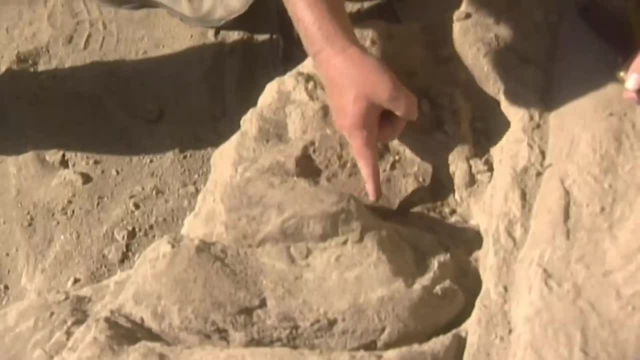 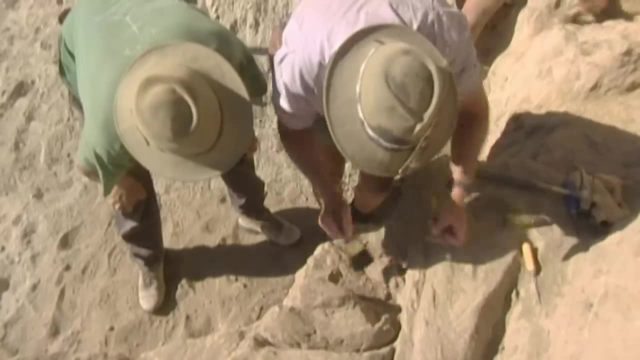 But look, it's folding down there, Look, it's coming right the way across there, Look, look. and if that cracked surface is bone and that surface there is bone, it's getting enormous. In the end it turns out to be too big. 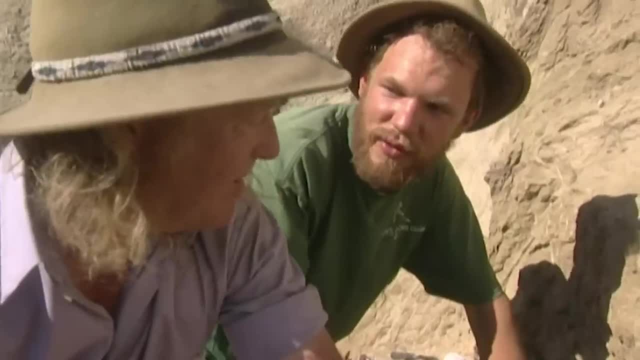 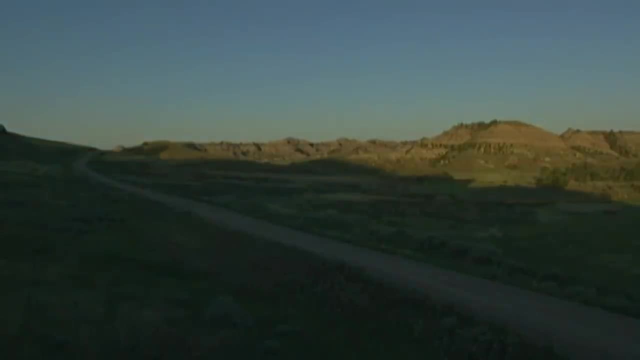 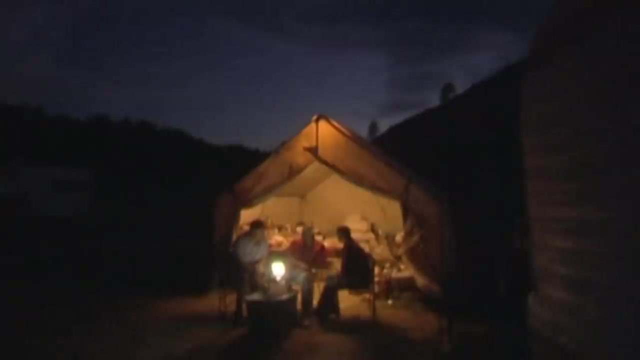 even for Phil to handle- and he has to admit defeat. We need more work first. That's a major piece of work. At the end of the five years, what would you like to walk away from this site having achieved? I hope that we will have gathered. 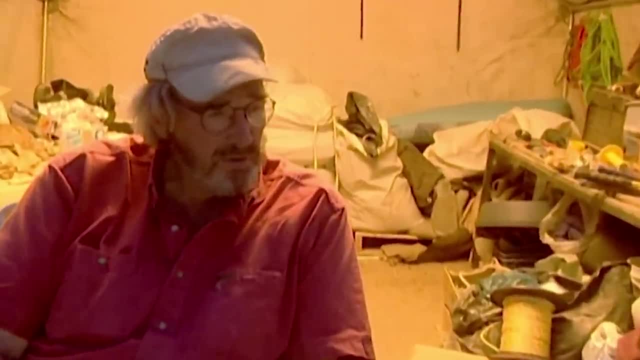 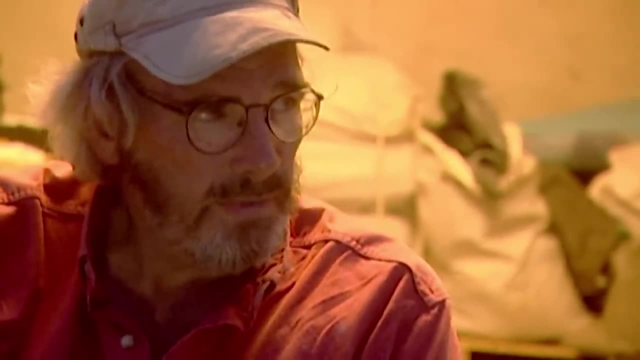 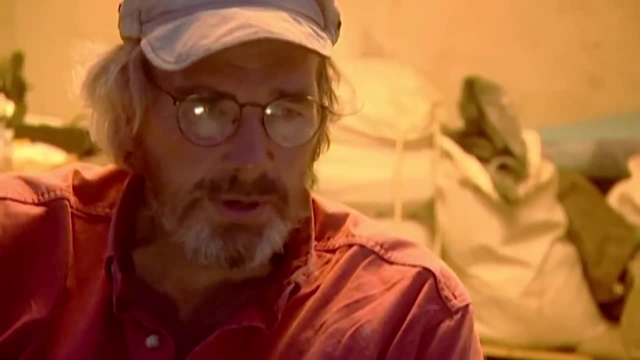 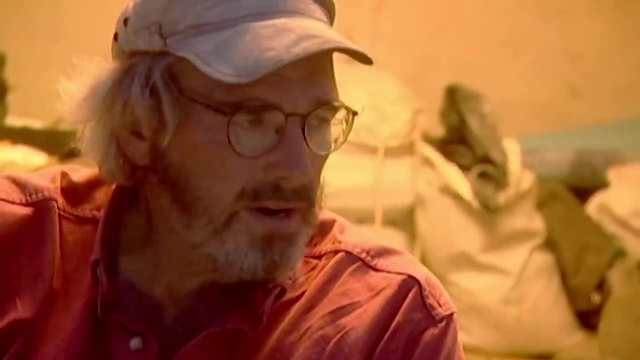 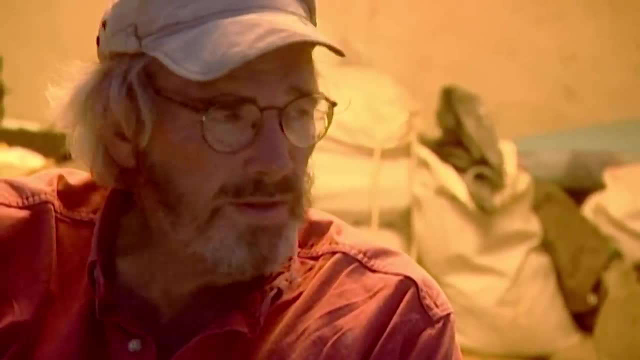 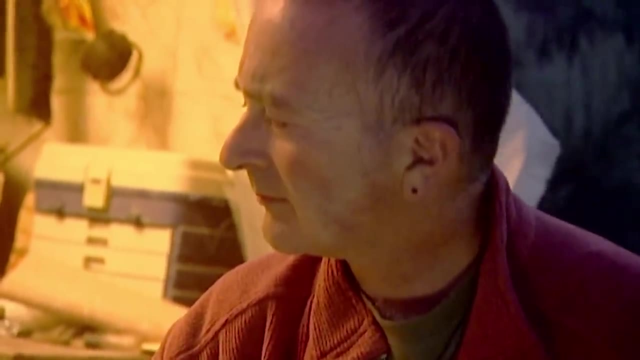 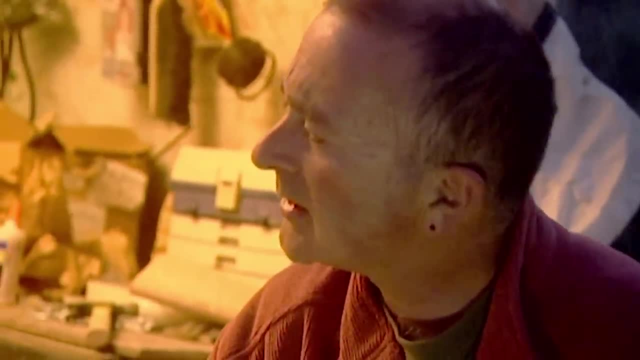 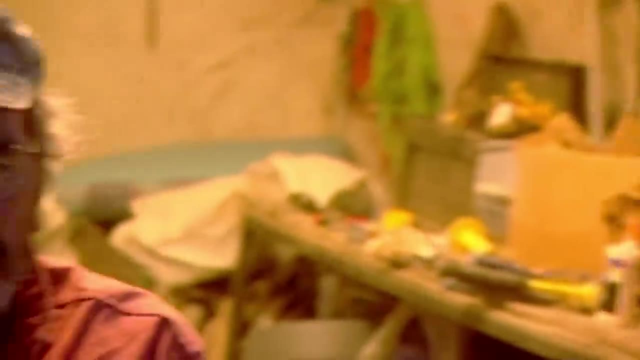 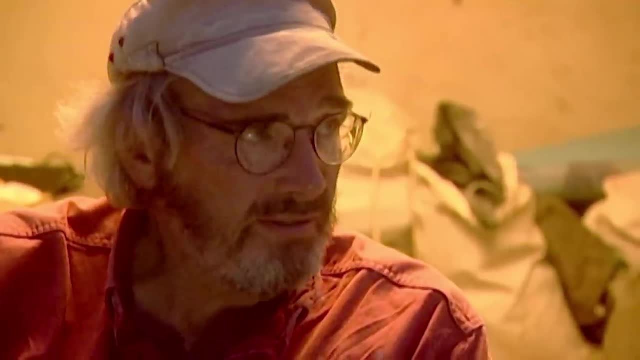 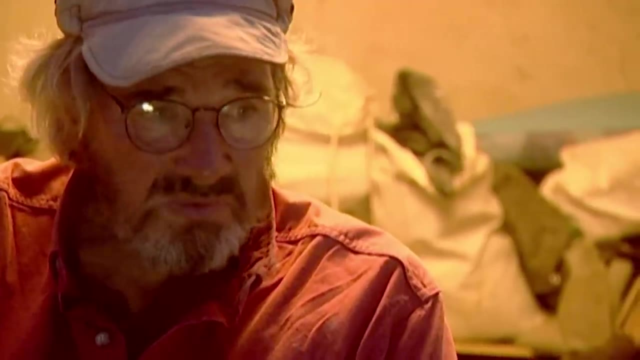 dig up a dinosaur, bring it back to your museum, shake all the dirt off of it, mount it, put it up, make a big, pretty skeleton, go back out and find another one. Some people you know have gathered a little bit of evidence. 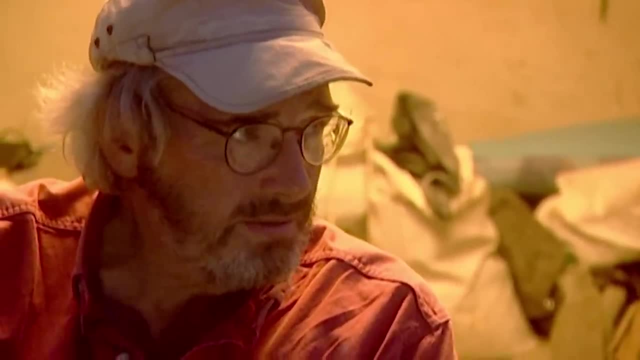 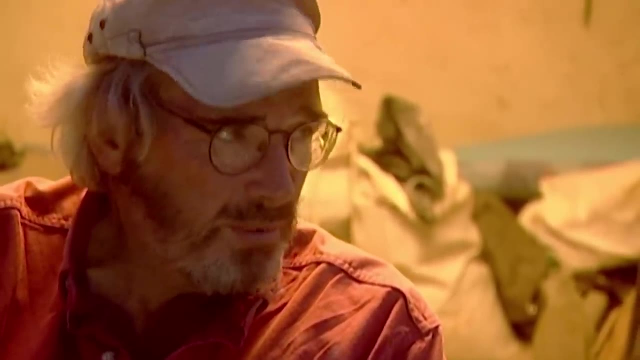 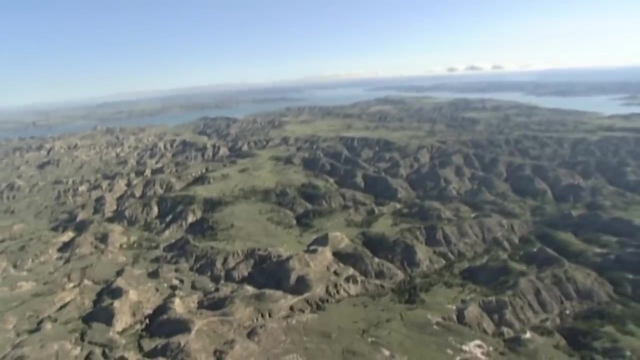 to say, to get a general picture of what kind of climates you know or what kind of environment the animals lived in, but not specifically, not to the degree that we are doing it. In fact, after just three years, Jack and his team already have enough information. 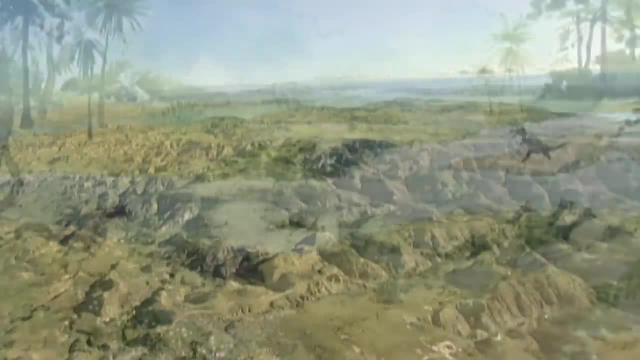 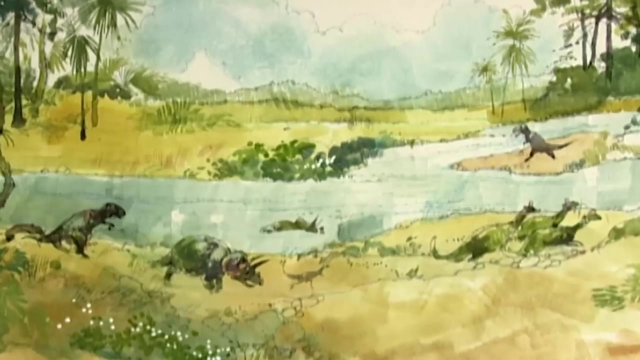 to produce a basic picture of life here in the Cretaceous. Then Hell Creek didn't exist. The land was flat and sparsely forested with huge trees like giant redwoods. Numerous slow-flowing rivers meandered lazily across the plain. Lizards, mammals, crustaceans and fish all lived here, But the dominant creatures were the dinosaurs. Herds of Hadrosaur, the wildebeest of the Cretaceous, foraged in the savannah alongside Triceratops. 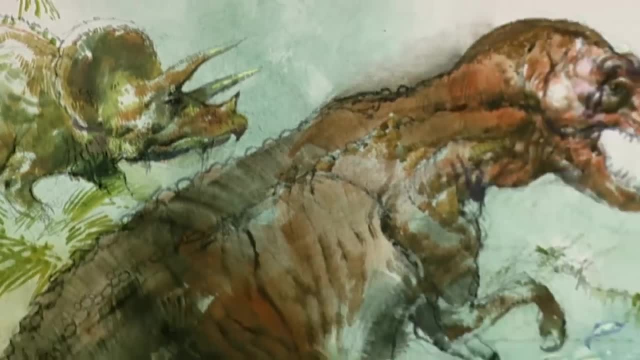 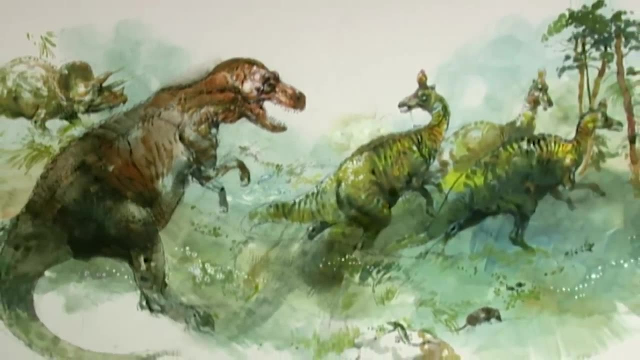 and various other plant eaters, all eyed hungrily by the ever-present T rex. But this was the very end of the Cretaceous and the dinosaurs. Within a few million years, they'd all be dead, Jim. we've heard so much talk about dinosaurs. 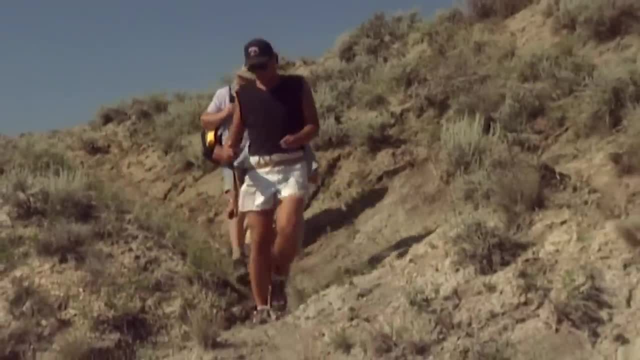 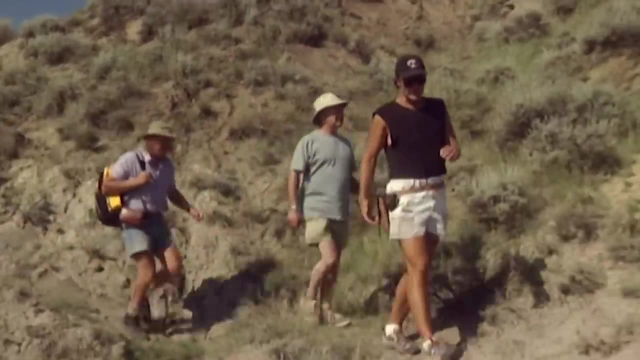 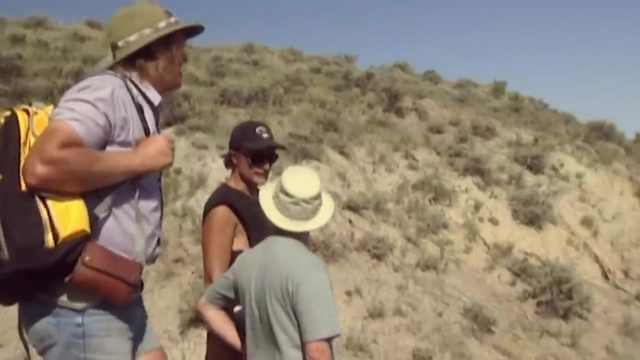 but what about the K-T boundary? What is it? Well, the K-T boundary marks the disappearance of dinosaurs from the fossil record, And so the K-T boundary separates rocks below that contain dinosaur fossils from rocks above which do not contain dinosaur fossils. 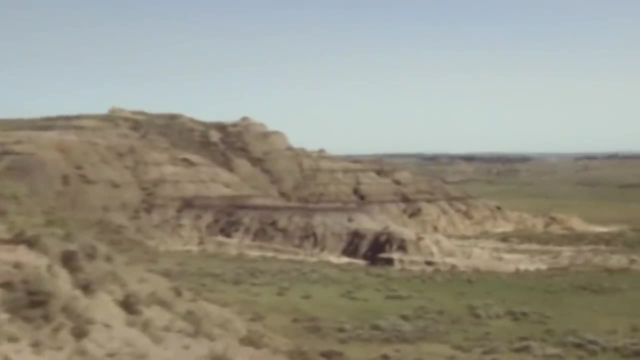 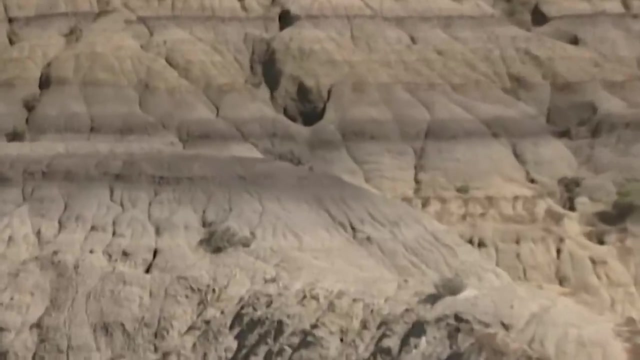 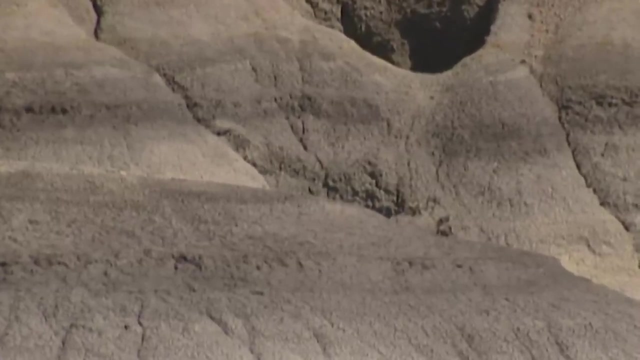 And if we look over here on this ridge, we see actually the K-T boundary exposed. If you look at the layering in the rocks, what you see are a whole series of black layers and those layers are coal layers. The lowest coal layer that you see there is the K-T boundary. 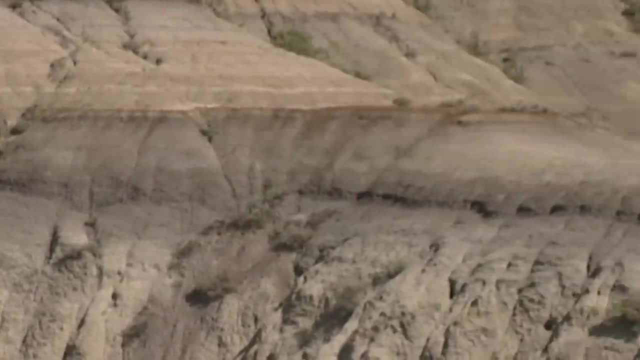 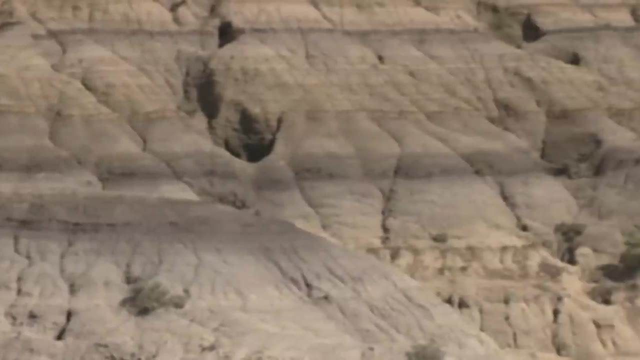 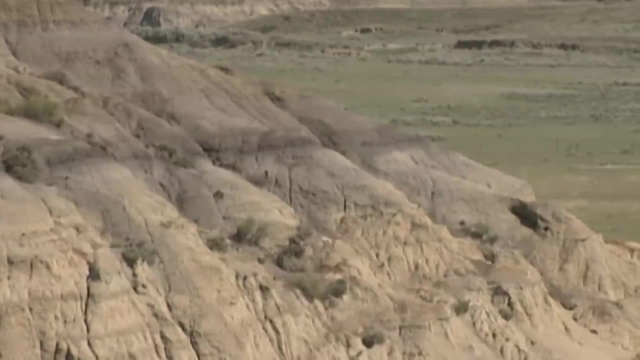 The K-T boundary records a huge change in climate. There's much debate about what caused the change, but the most popular theories centre on the impact of a giant asteroid. And do the dinosaur skeletons go actually right up to the boundary? Can we actually say that it looks as though whatever happened? 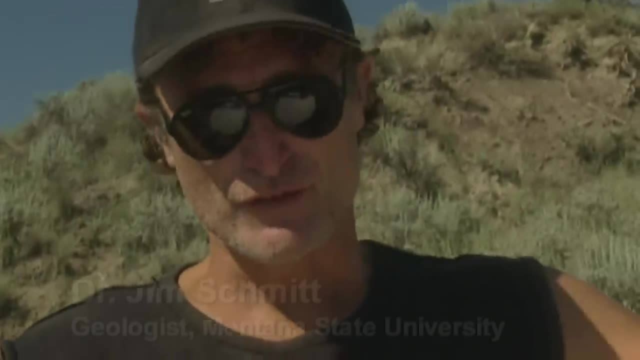 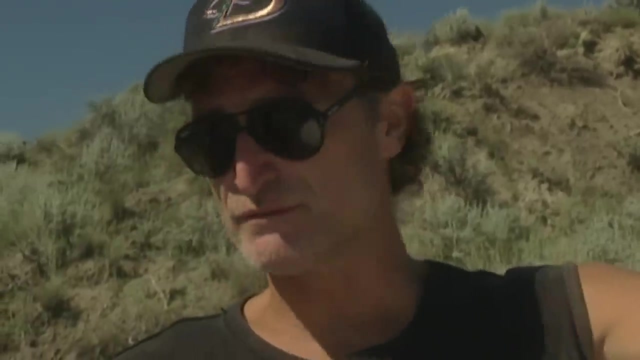 it was that thing that killed the dinosaurs off. Actually, essentially everywhere you look at it, you cannot say that. In fact, what you see is a very, very slow disappearance of dinosaur fossils as you go up towards the boundary. So it's a very gradual disappearance of the dinosaurs. 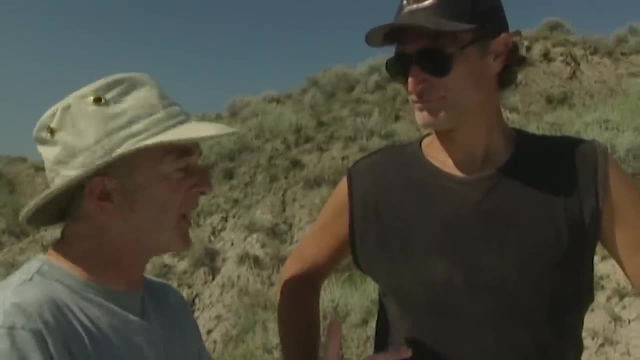 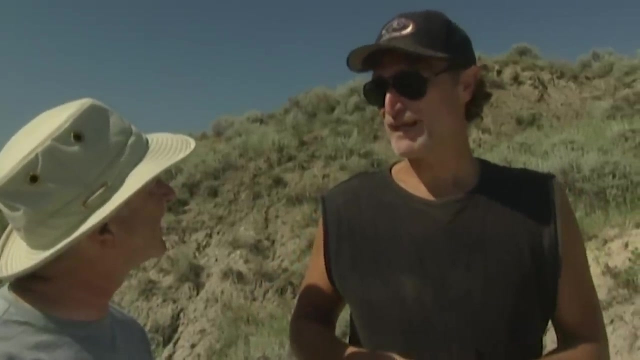 So this thing that everyone was taught at school that the dinosaurs were all living and happy and suddenly something went zoomf and wiped them all out? that's not true. That's probably not exactly the way it happened. The effects of that impact probably took hundreds, thousands. 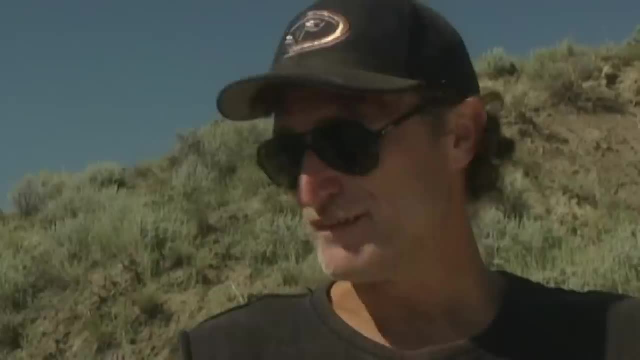 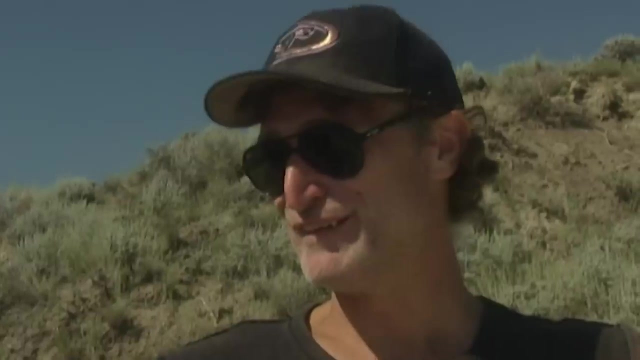 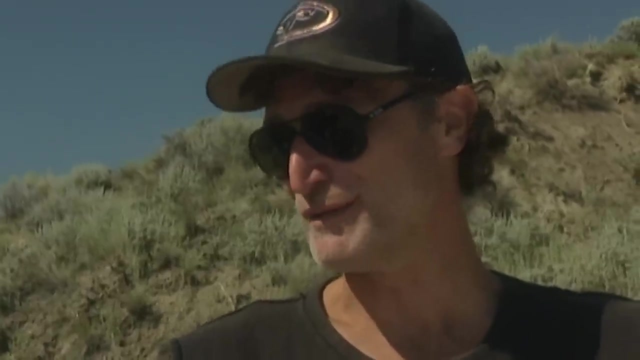 perhaps tens of thousands of years to play themselves out. The notion that you have from everything you've learned about an asteroid flying over the sky and dinosaurs looking up at it and it hits the Earth and they fall over all dead all at the same time, is not the way it, in all likelihood, happened. 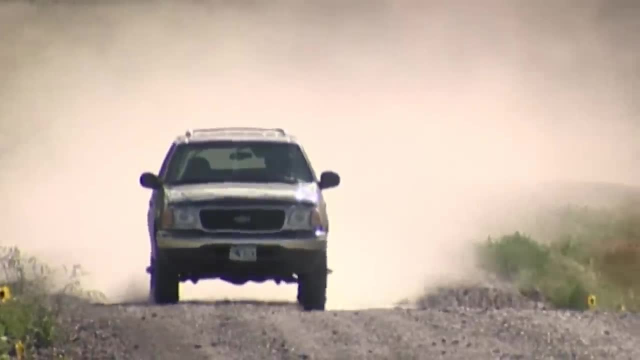 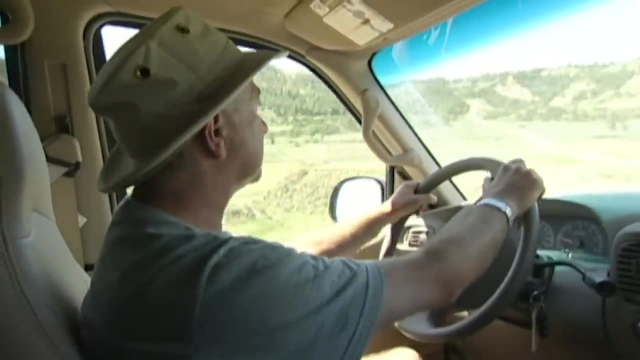 We've had a great time in Hell Creek, Especially Phil, who's still bragging about his T-Rex bone. But that's not the only thing bothering me. You know what really frustrates me? We've been here for the best part of a week. 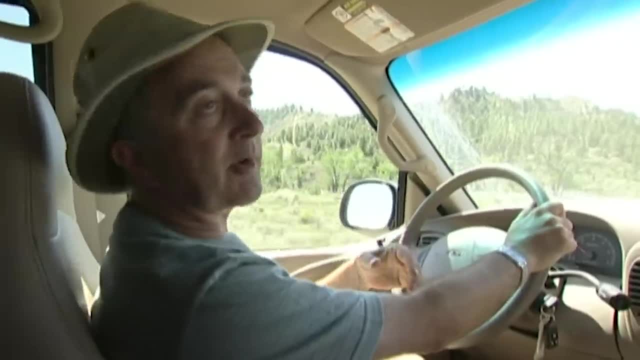 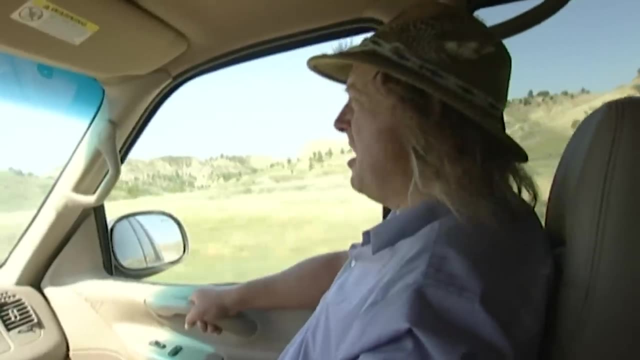 and I still haven't seen a clean dino bone. Everyone I've seen has been surrounded by clag and rock. Yeah, but I mean I suppose it just reflects the time that you've actually got to spend taking out each bone. I mean, I'm sure that the only way that you're going to actually 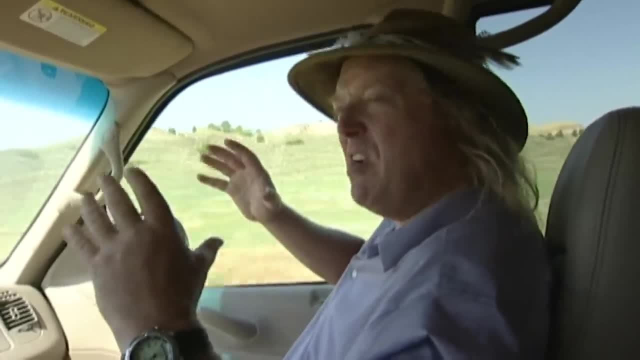 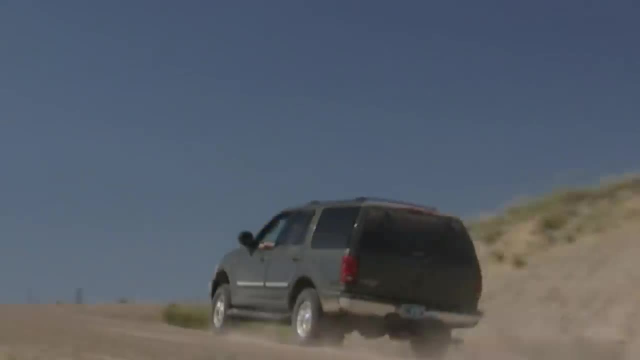 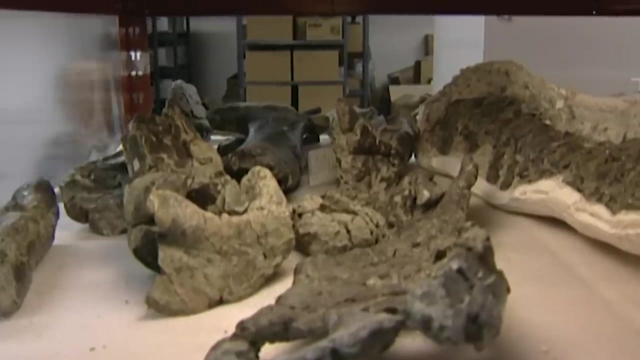 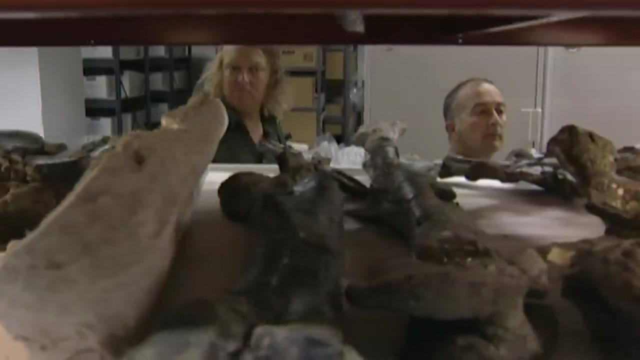 physically see a bone intact in whole is actually in a laboratory. Philip, that is precisely where we're going, And we've been promised some big surprises. We've come to the Museum of the Rockies to see bones, and the labs are full of them. 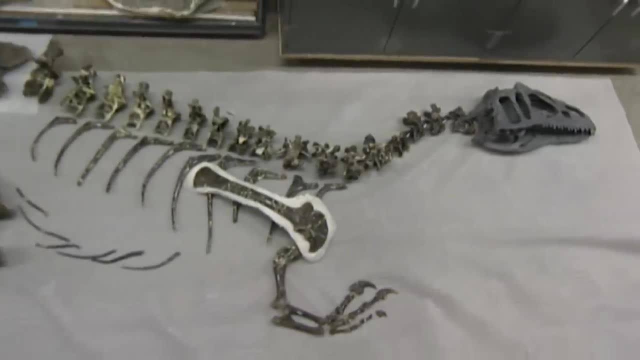 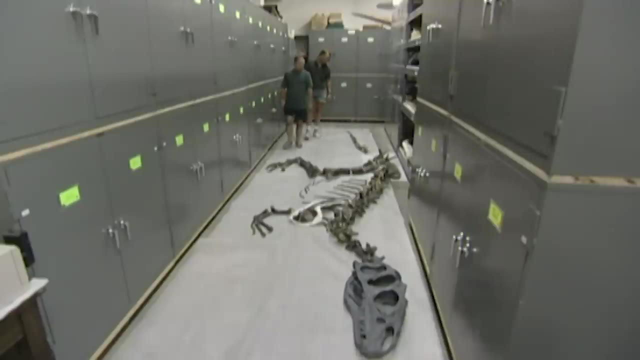 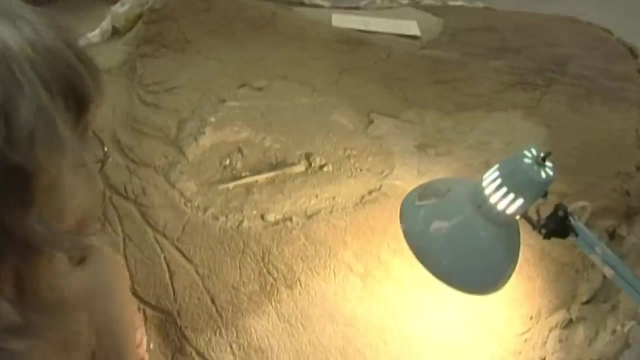 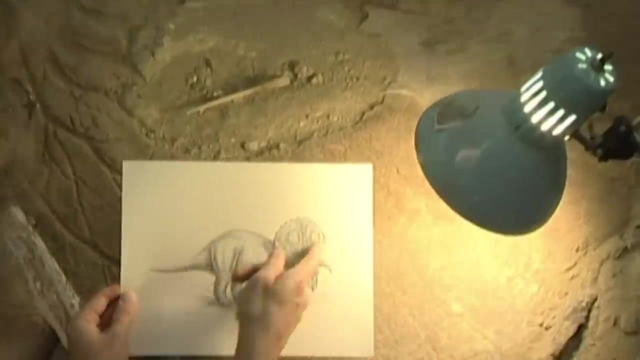 The staff have even laid out an Allosaurus skeleton for us. They come in all shapes and sizes, these bones, but with a five-foot diameter. the biggest and weirdest is definitely this: It's a Torosaurus frill freshly excavated from Hell Creek. 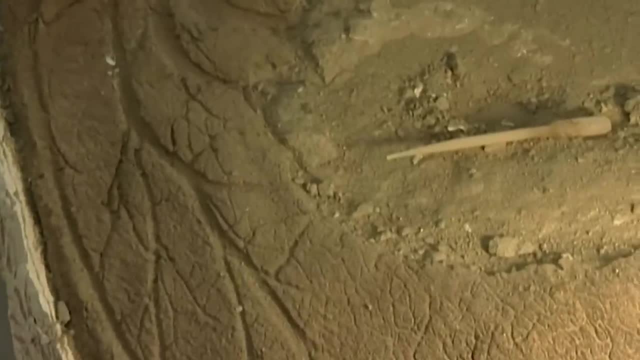 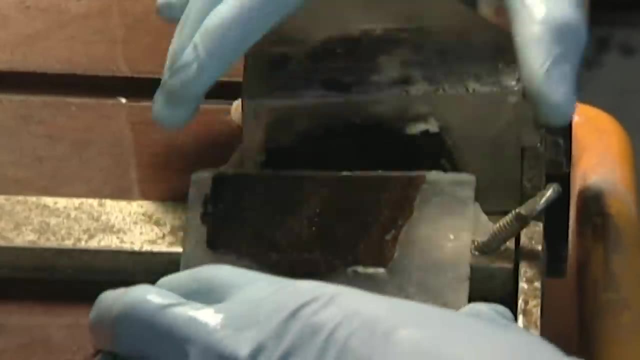 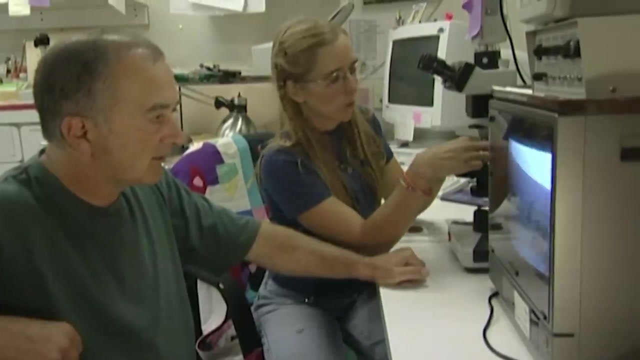 The grooves are where the veins ran. The bones are full of information. Amazingly, fossilisation preserves bone cell structure, and this allows scientists like Ellen Lam to build up a detailed picture of individual animals. This, for instance, is a fossilised turtle bone. 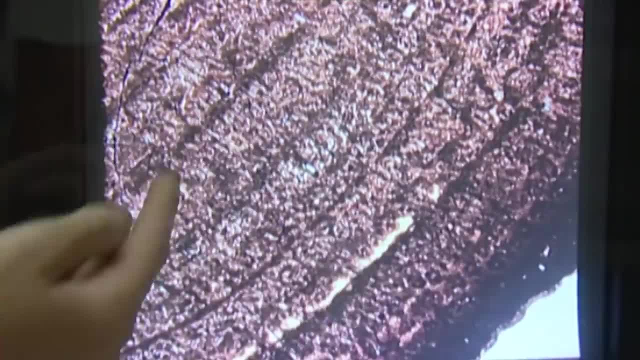 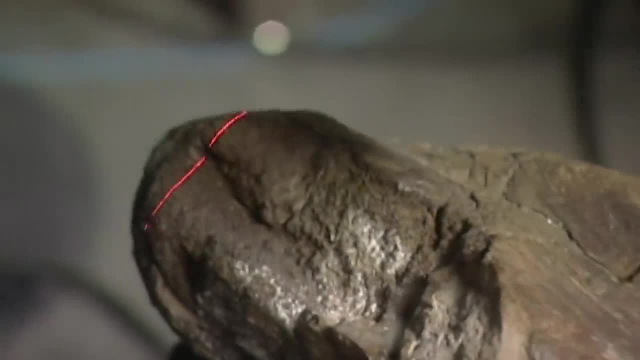 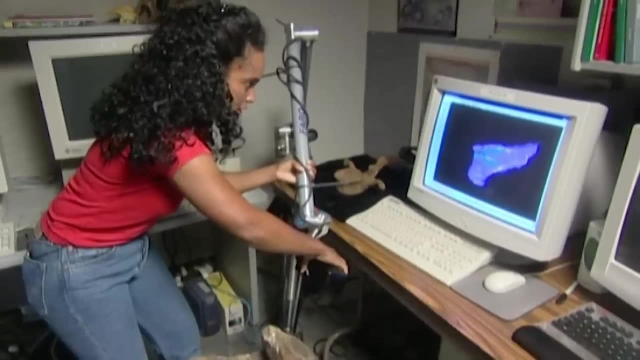 and the growth rings show it was unusually old when it died. Celeste Horner is building a virtual T-Rex. By scanning its bones into a computer, she can recreate its movement And the results look set to cause a big stir From the information that we have now. 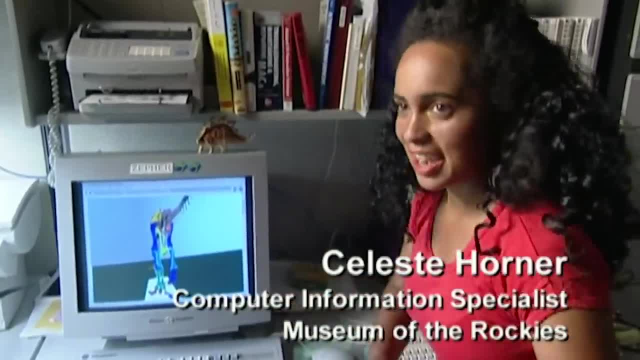 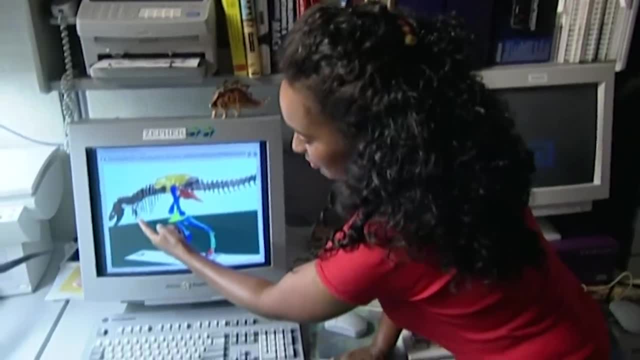 T-Rex could not really manoeuvre side to side like an athlete would, and the kind of actions that you'd need if you were a hunting animal. We see a T-Rex had very small arms. That would be a great disadvantage if you were a hunter. 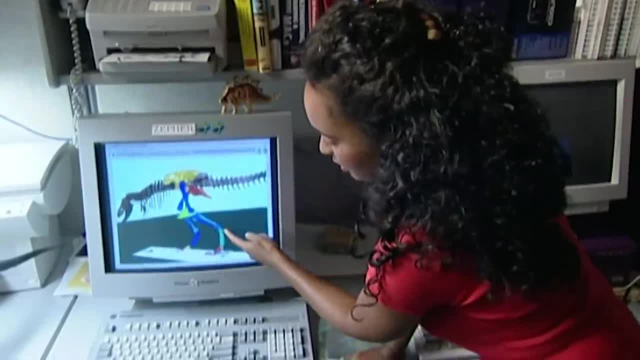 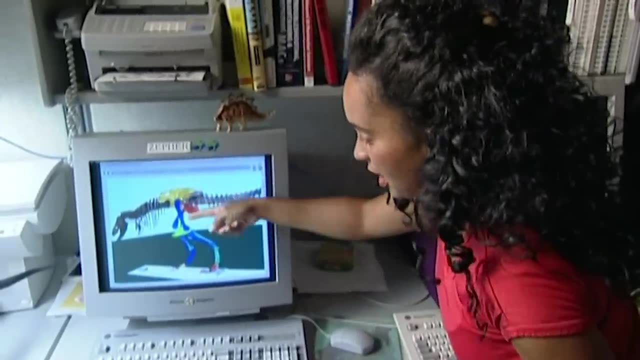 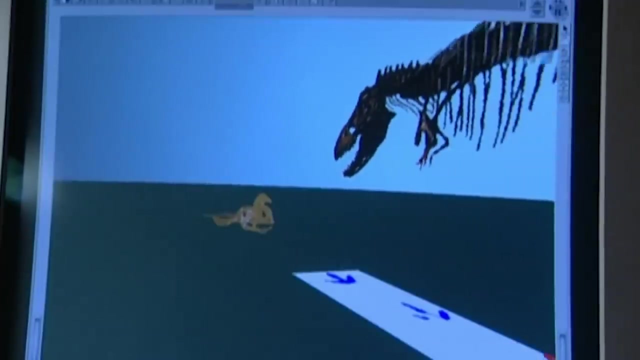 It has almost equal thigh and shin bone proportions, which is not what you would expect in a fast runner. A fast runner usually has a short thigh bone and a long shin bone. In other words, T-Rex might not have been the fearsome predator portrayed in books and movies. 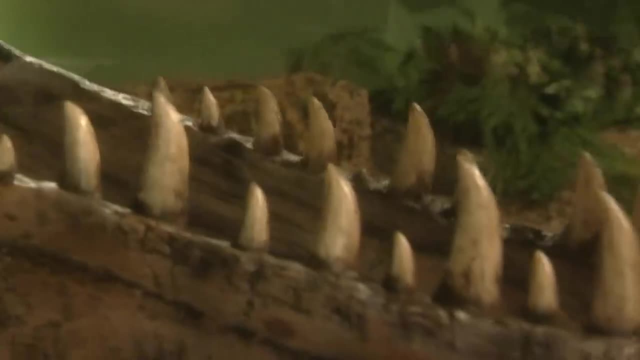 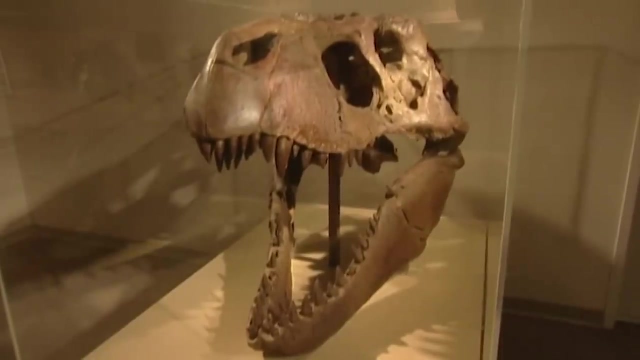 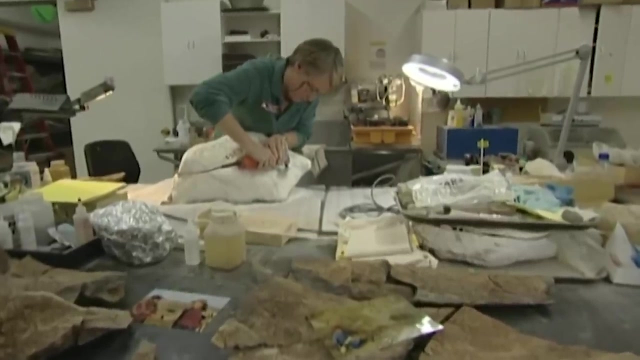 Celeste thinks he's more likely to have been a scavenger, a kind of giant prehistoric hyena, which just goes to show how misleading appearances can be. Getting the bones into shape for all this analysis is the job of preparators like Jamie Jett. 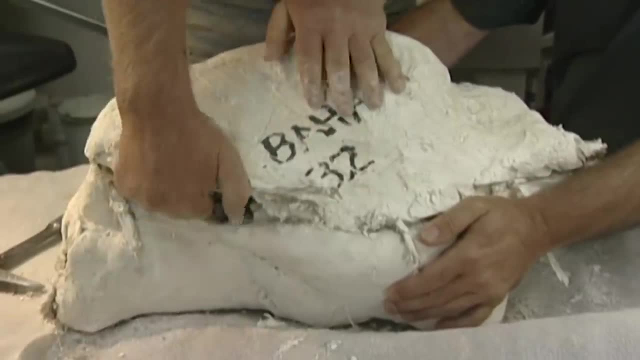 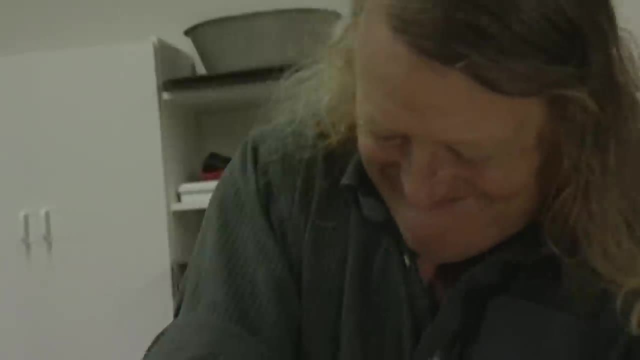 Somewhere in this jacketed lump of rock is a dinosaur bone. In fact, this one is from Dave Vericchio's Bahamas site, so there's likely to be a jumble of them. That's it, that's it, that's it. 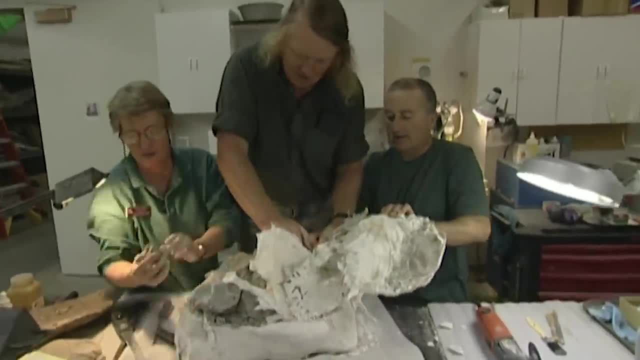 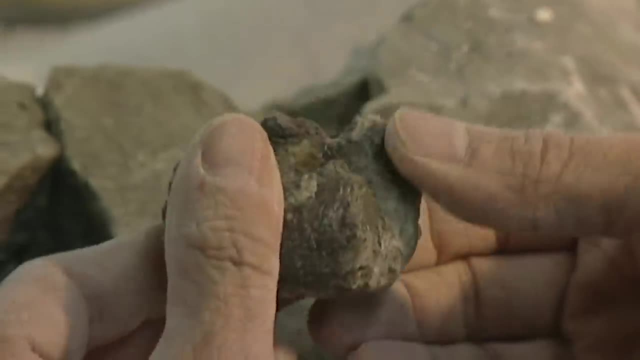 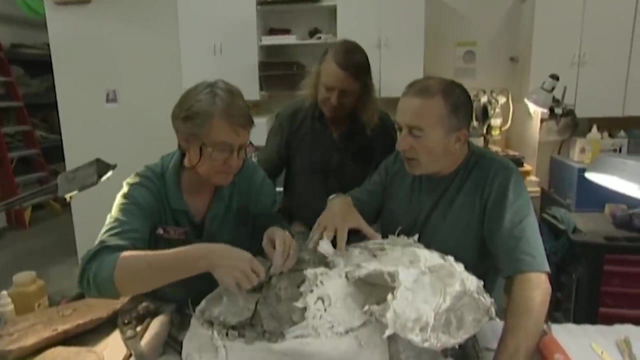 Ah, here we go. Phew, that made me blow a bit. There's some dinosaur bone, So the job now is to get all of this matrix off of these bits of bone that are in here. How long will it take you to get all this rock off? 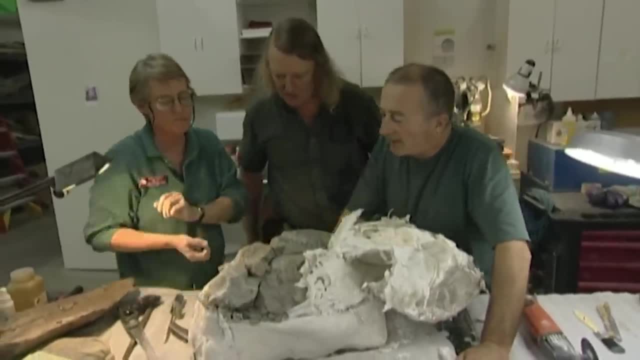 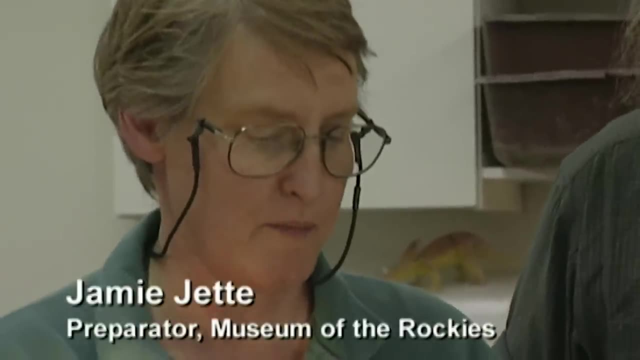 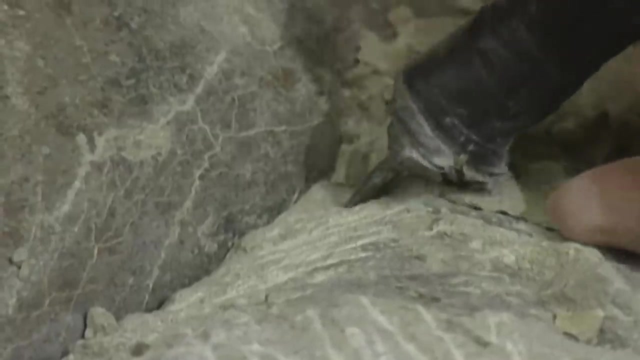 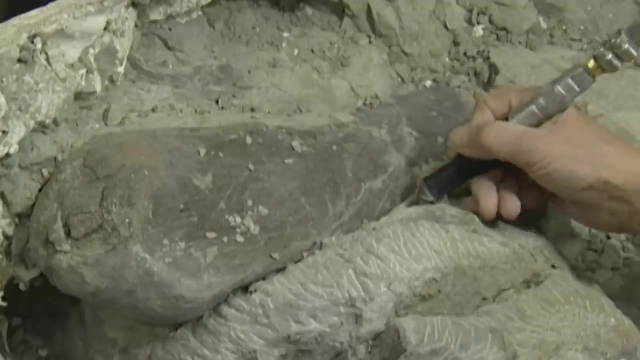 and clean this out. If I'm lucky, maybe a couple of months. If I have trouble getting the rock loose from the bone, it can take anywhere up to six months, And you can see why Jamie can't just hack at the rock for fear of damaging the bone. 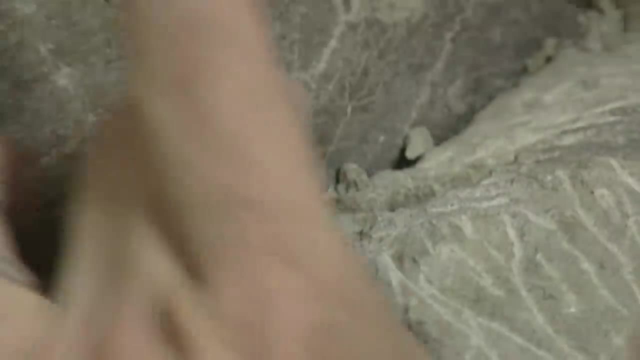 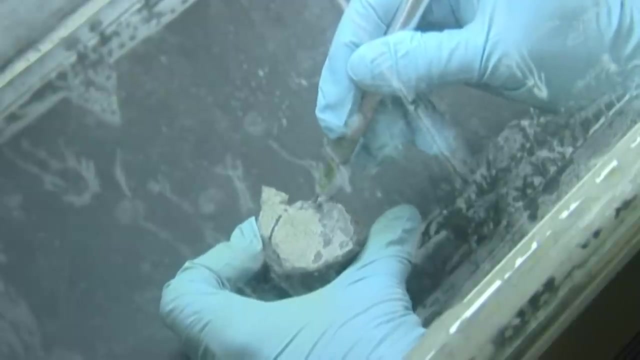 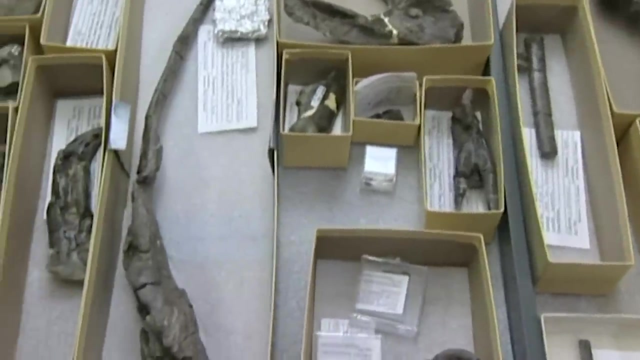 Instead, she's got to remove it millimetre by millimetre. It requires almost surgical skill, But the effort's worth it. All this stuff came from your site. This is last year's collection. It's beautiful, isn't it? It is. 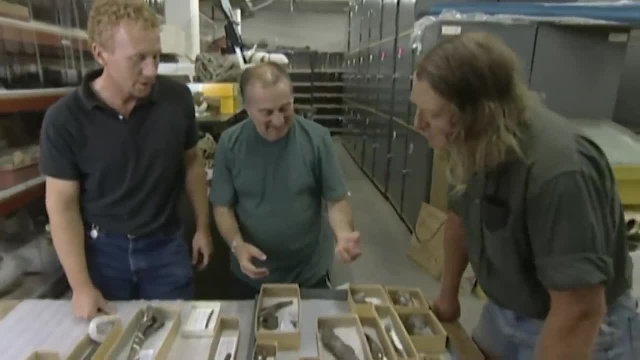 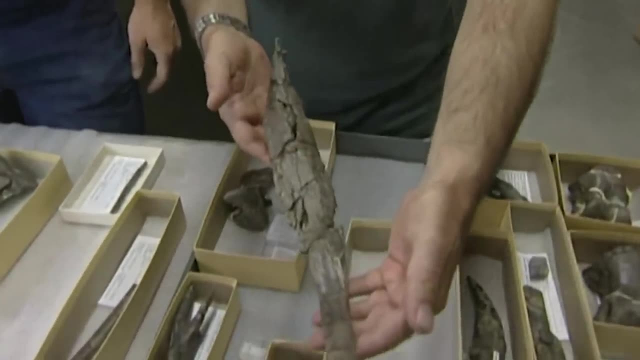 When you see it in the rock, it doesn't look as though you'll ever get it to this state. What's this bit here? That's one of the belly ribs. Look at that. Good Lord, I know you're nowhere near finished. 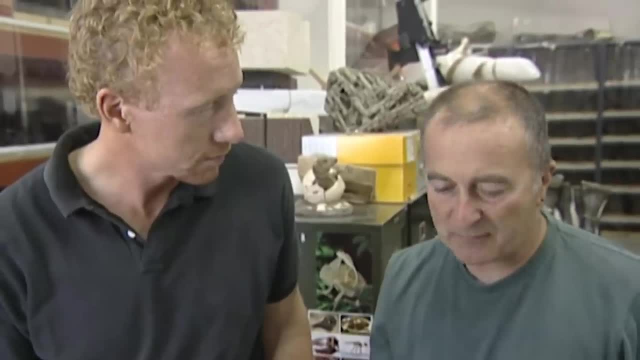 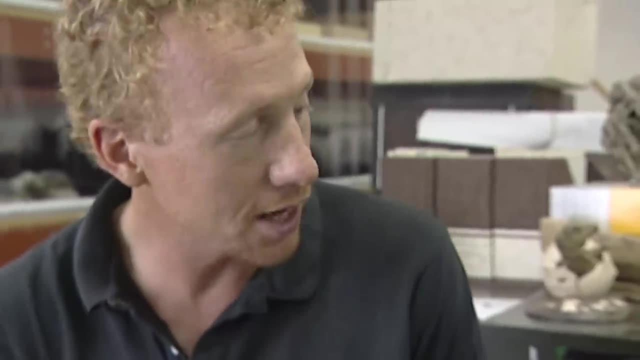 but from the evidence that you've pulled together so far, what can you tell about this animal? Well, we can definitely tell it's a Tyrannosaurid. From the material we worked on this summer, we can actually tell it's a Displetosaur. 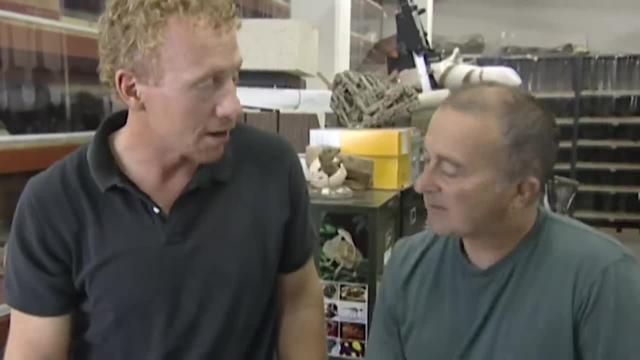 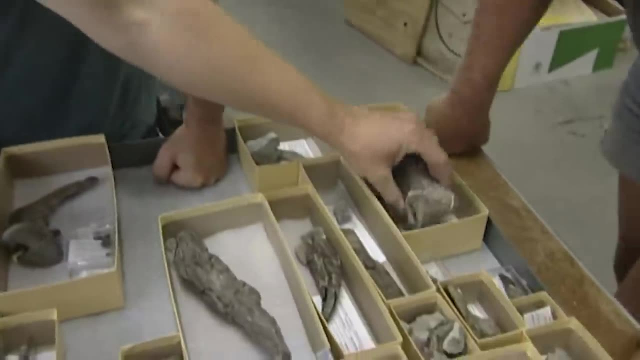 so a particular type of Tyrannosaur. We can tell it's larger than our other specimen, so this is probably a full adult animal. Yeah, and we can see that on Here's a toe bone, So this is just one of the bones from the foot. 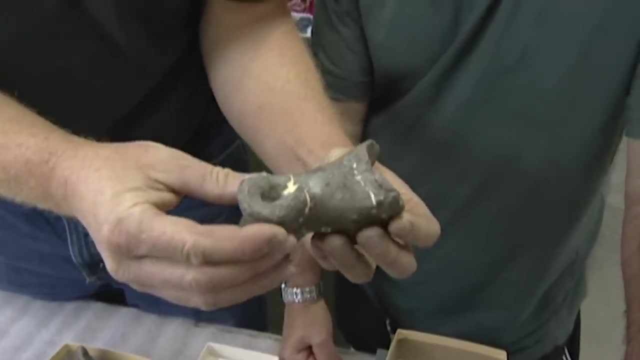 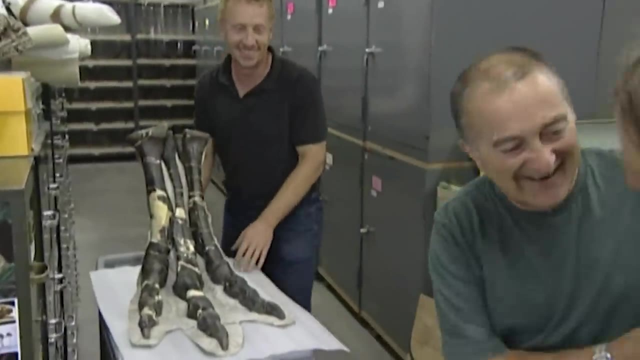 Good Lord, And we can compare that with our other specimen. Why don't you hang on to that, Yeah And then, Ah, We're back in the movies One day. one day, yours will look like that, Hopefully, hopefully. 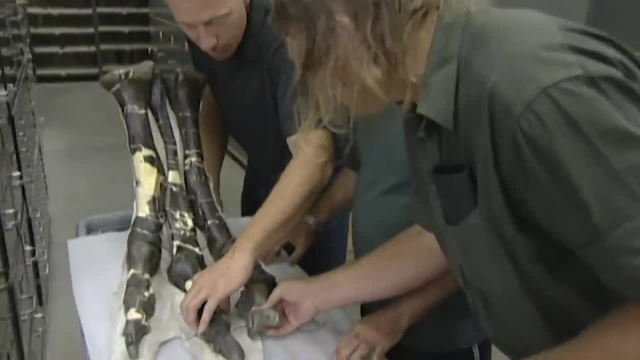 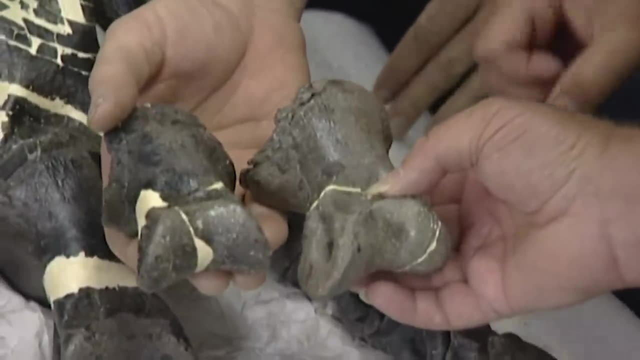 So which one is This? one matches this bone here. yeah, Let me get that out. Yeah, so you can see It's bigger, isn't it your one? Yeah, And this actually is a fairly mature individual, so ours is definitely a mature individual. 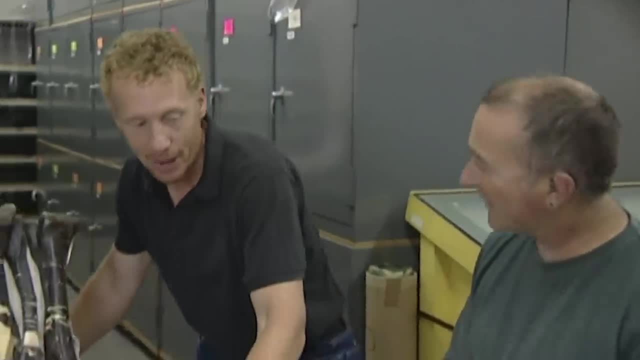 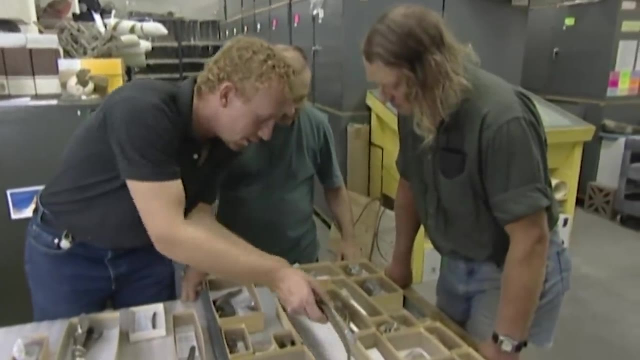 And we also have some unique features too. some pathologies, Ah Ah, Injuries to the bones, Yeah, And this bone that you picked up earlier is actually one of them. This is the belly rib, And so you can see it sort of has a normal portion down here. 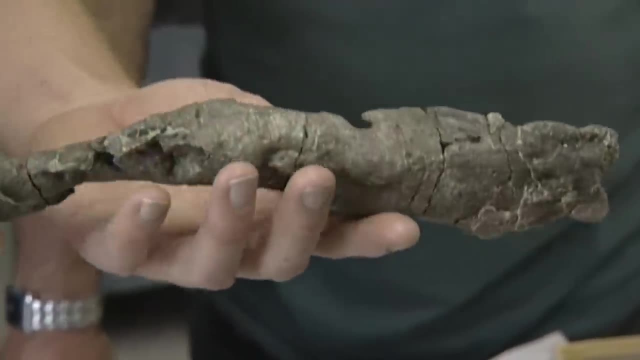 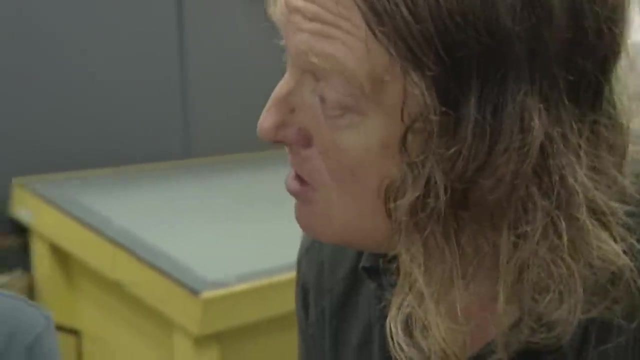 and then we get to this area here and things really go haywire. That's not just because it's been smashed up, No, So does that mean that during its lifetime it had an injury and that healed Right? Well, I'd say it. 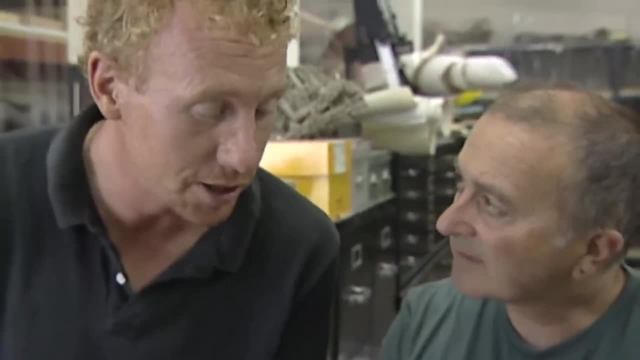 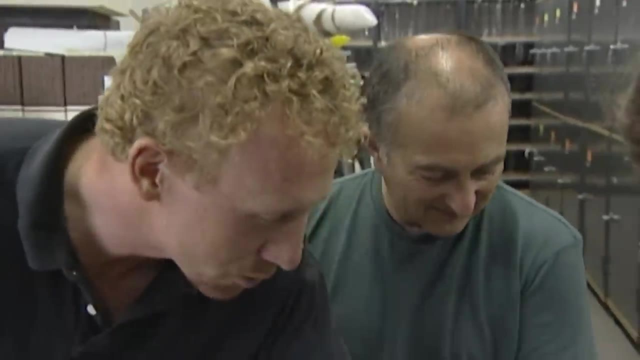 I'm not sure it actually healed The bone reacted to that injury, So it didn't die of that injury. Ah, that's a good question. It could have. I mean this. I'll show you. This is what it should look like, this end of the bone. 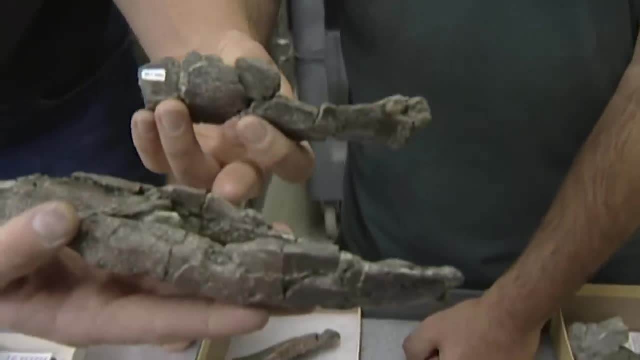 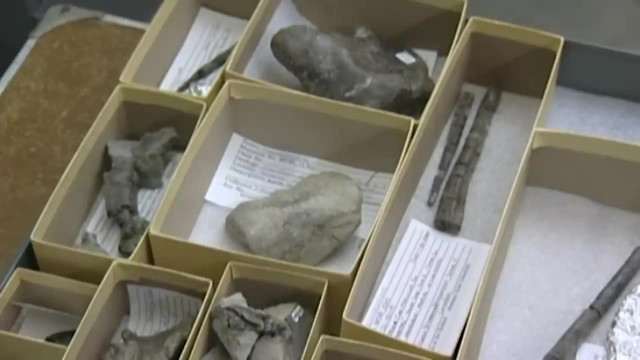 It should be very flat And instead we have this large cavity which suggests there's some kind of- maybe an infection or tumour growing within the bone. This is beginning to feel like archaeology again. The only difference is on Time Team. 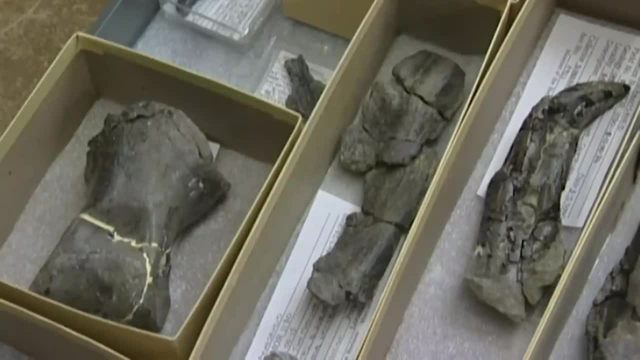 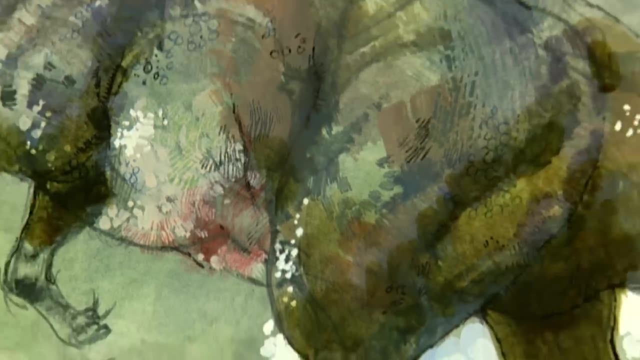 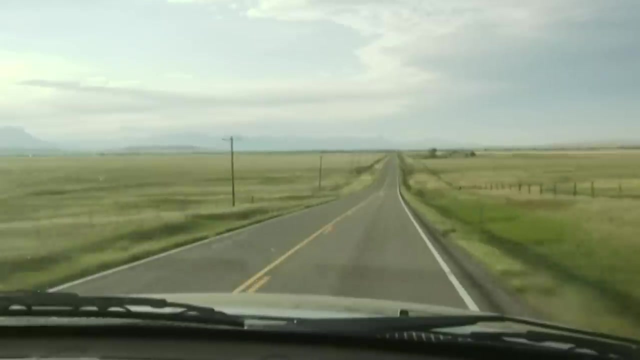 we're used to getting results in three days, not six months. Nevertheless, Dave's daspletosaur- one of only four in the world and probably the most complete- is slowly coming to life, But most of its bones are still in the ground. 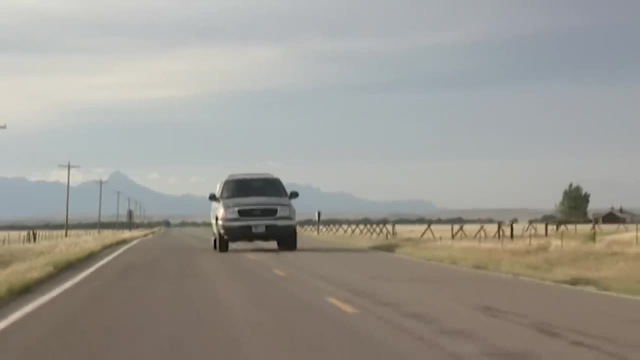 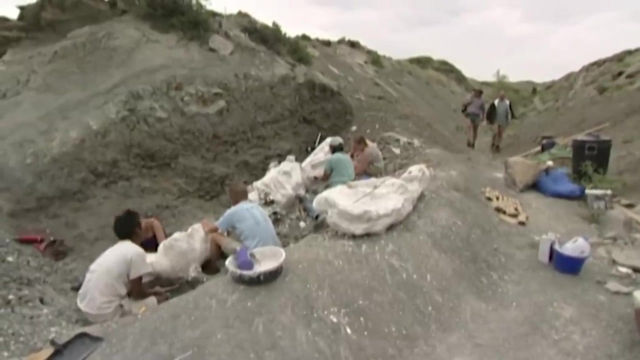 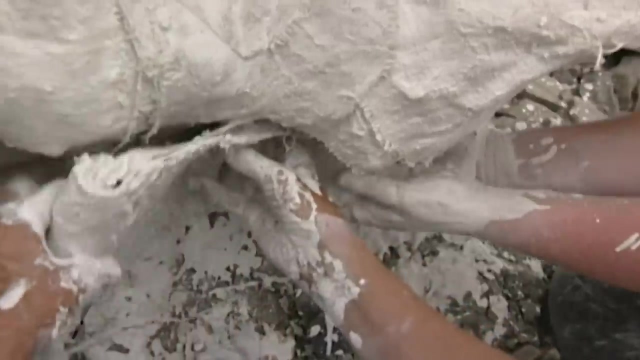 So on our last day we're heading back to the Bahamas to help Dave get them out. They've finally been isolated into clumps, recorded and jacketed. Now it's just a matter of getting them off the site and back to the preparators. 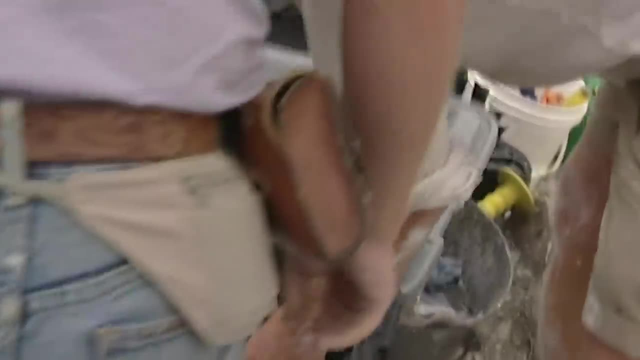 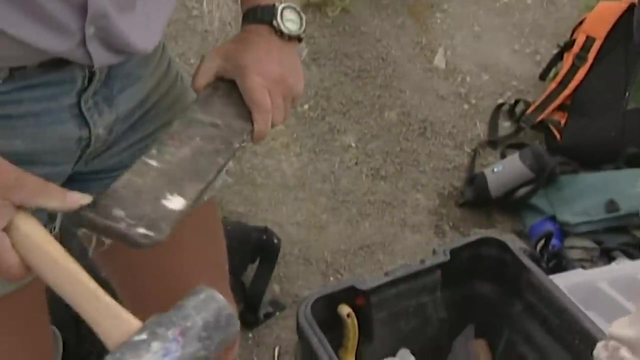 We have a special tool for this called the Dino Killer. The Dino Killer Looks like a big hammer to me. This is the Dino Killer. Oh, good God, that's a good tool. I can equate with tools like this. 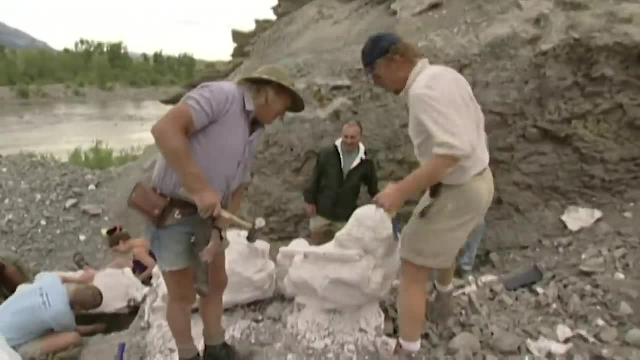 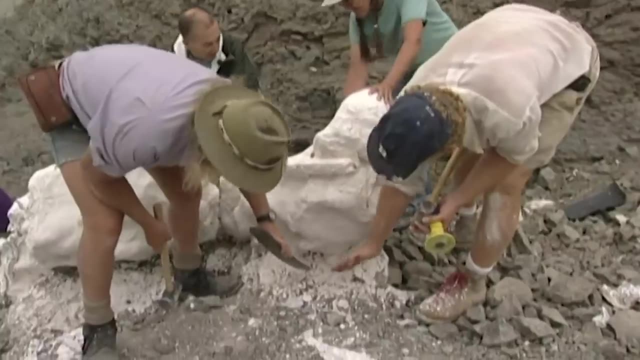 Right then. so what do we do with the Dino Killer? Basically, we have to drive it under this, But since the bed's dipping this way, we don't want to drive it horizontally, but down. So in there, Yeah. 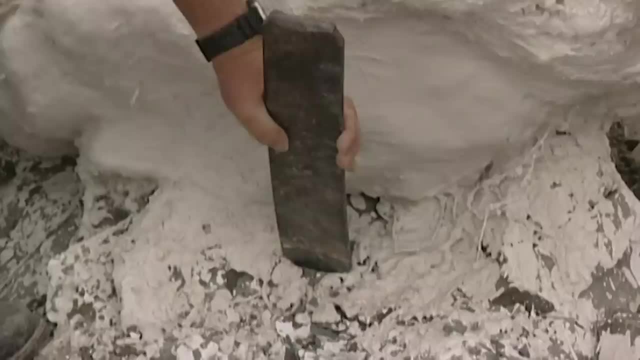 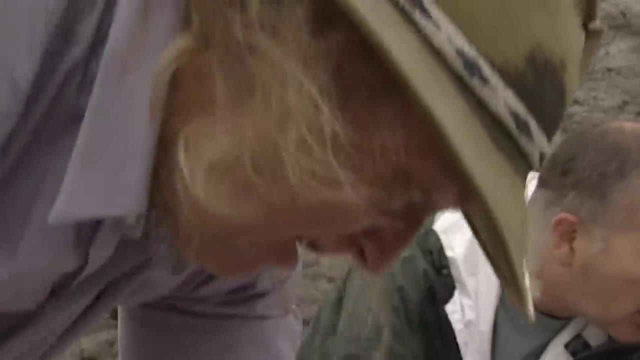 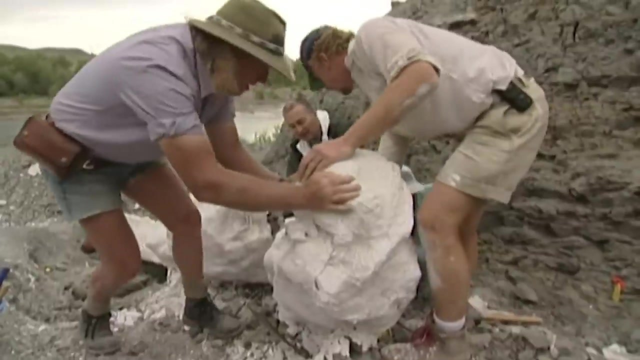 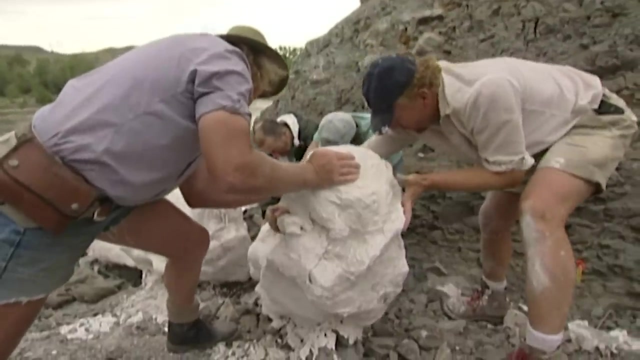 And then Oh, ah, That's right, It's gone. Yeah, it's gone. Wait, wait, wait, Are you ready? Yeah, Can you jack this? Yeah, Let's pull it around, Come on, come on. 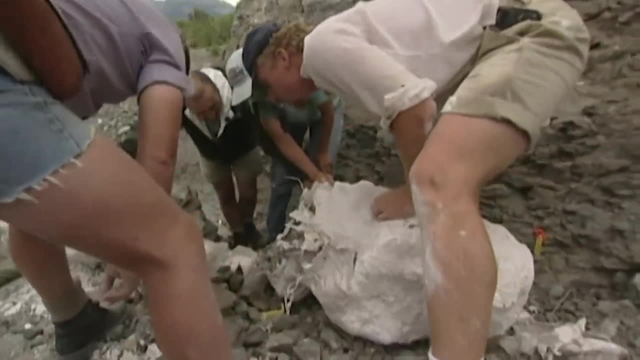 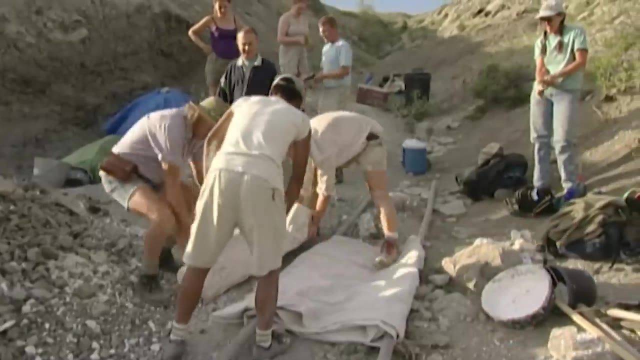 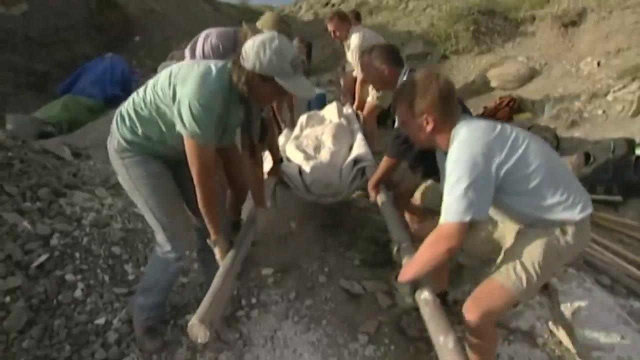 Bring it over, bring it over, Hey, that's it. that's it, Whoo. Now the Dino's dead, the fun really begins. Each of the jackets weighs around half a tonne, and we've got to carry them up the gully. 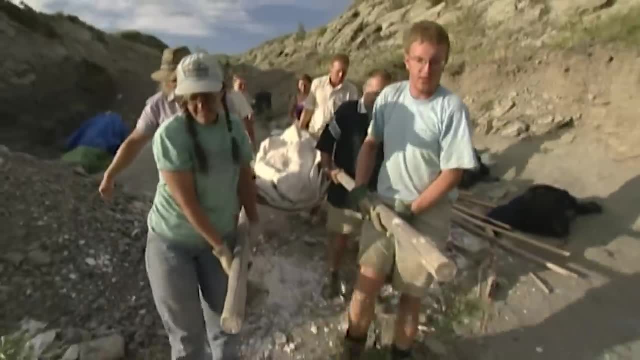 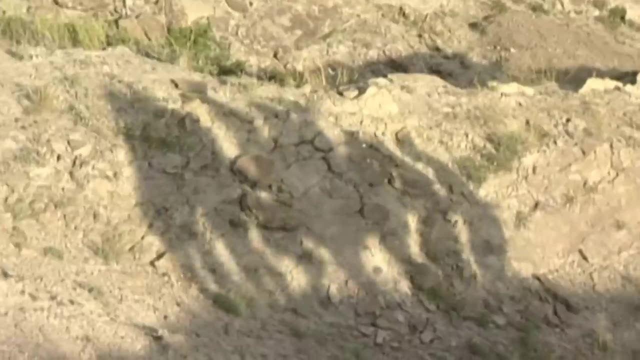 to where the trucks are parked. Sometimes it's really light, and then the weight shifts: It's incredibly heavy. Yeah, So this is why Dave wanted us back. You know what Got it? Whoa, How do we get it in? 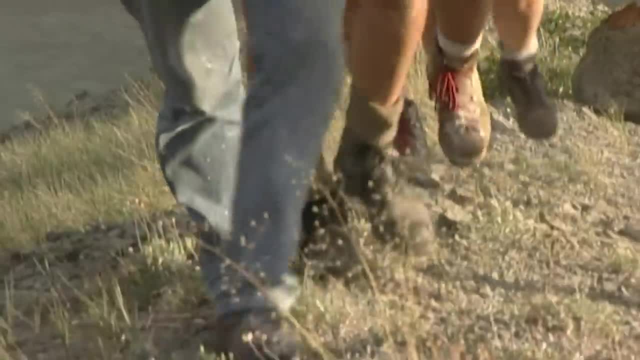 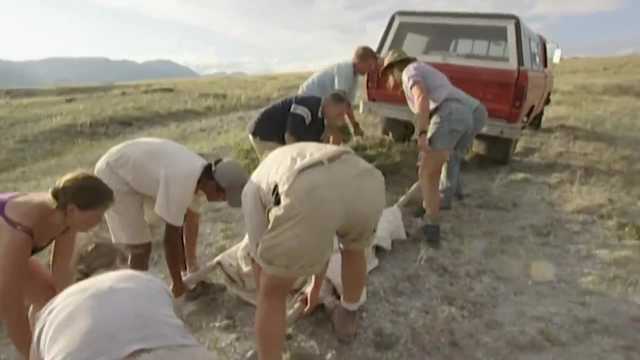 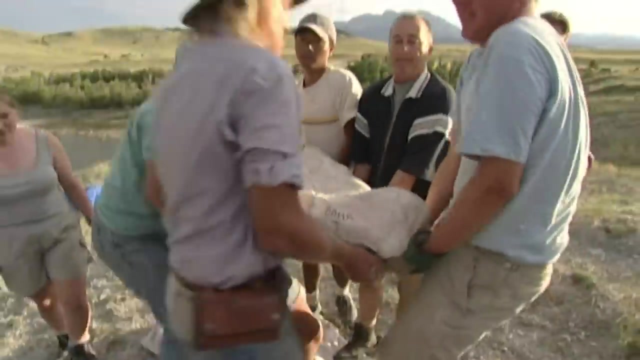